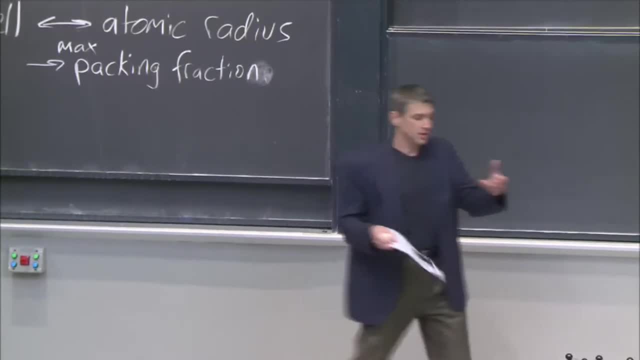 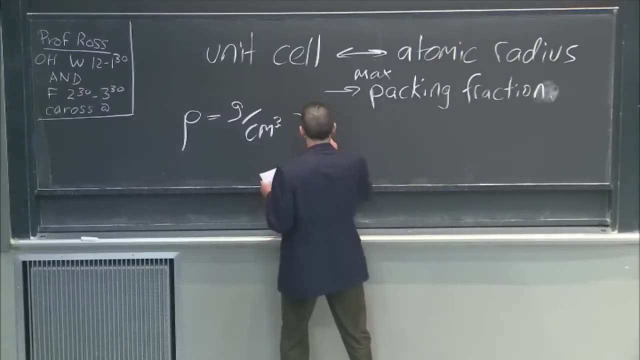 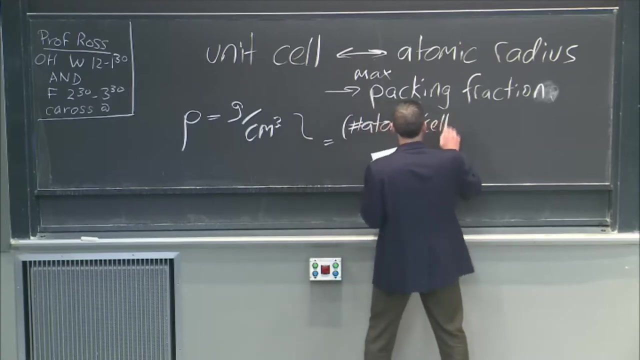 you know the unit cell and you can know something about the radius of the atom. maybe then you can get the density. For example, here the density could be defined as the number of atoms in the cell, right times the grams per mole of that element divided by the volume of the cell of the 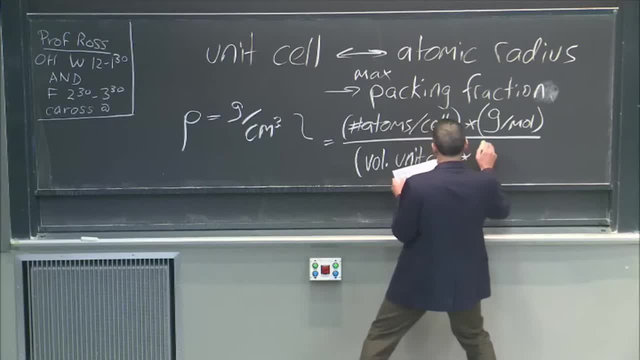 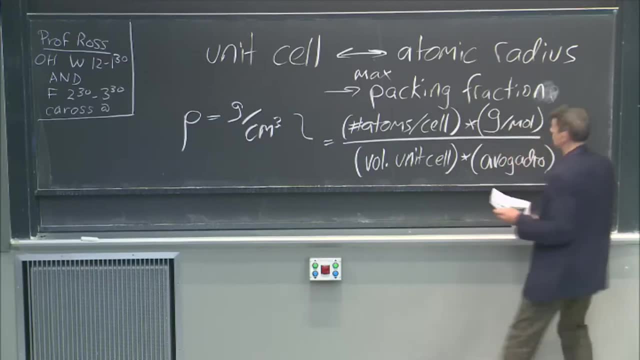 unit cell right times: Avogadro, Avogadro, Avogadro. Now you can go through the units and you can work out that this is grams per centimeter cubed. All right, And so just as an example, right? 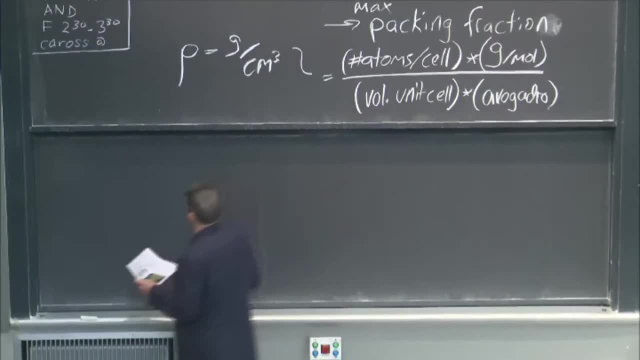 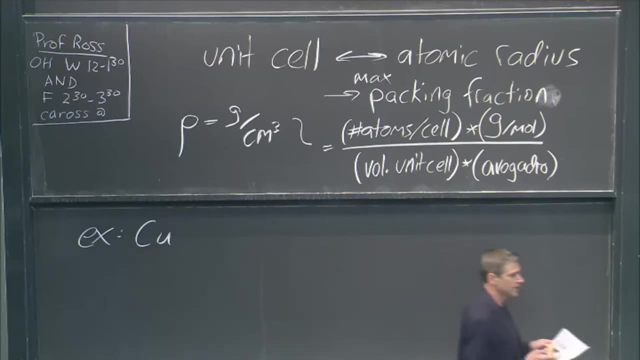 If I had. Let's see An example. I have is copper. So example: copper right. So everything comes from the periodic table, everything Life class, everything comes from the periodic table. So I say I want to know stuff about. 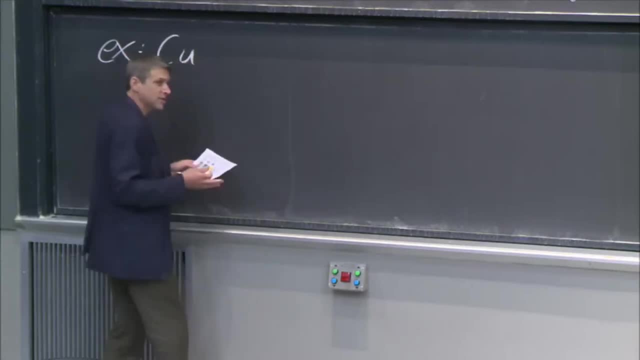 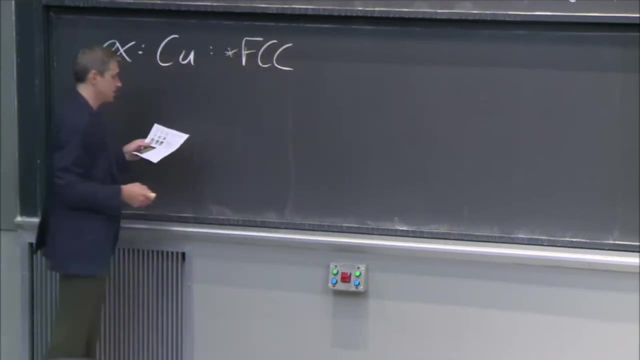 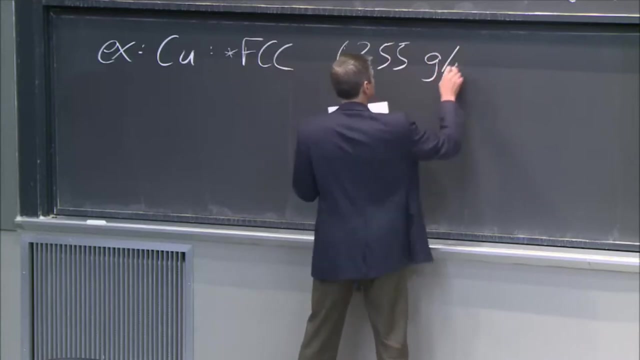 I go to the periodic table and instead of looking up the density, I look up other things. So I look up, for example, that it's FCC right, And then I look up that it's It's 63.55 grams per mole. okay. 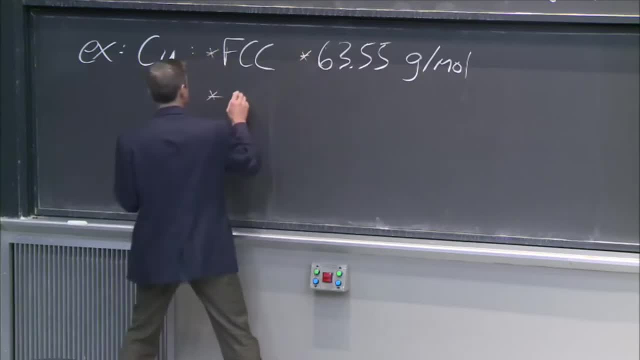 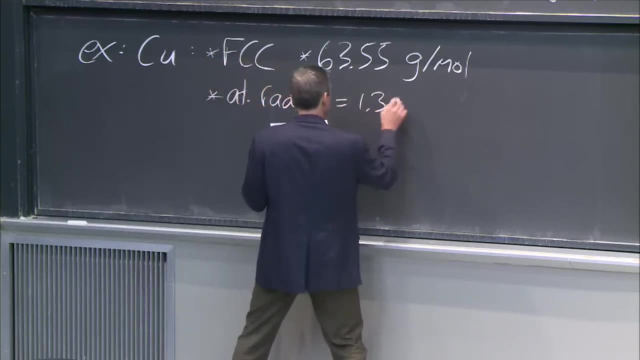 And I also look up the atomic radius. So I look up these things, right, The atomic radius, And that's equal to 1.3 angstroms. So I look all this stuff up And the point is I can now go back and forth. 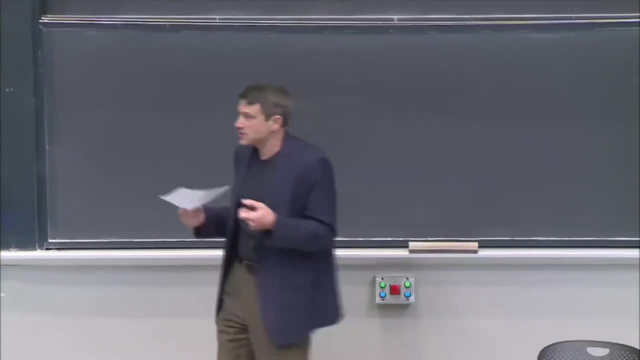 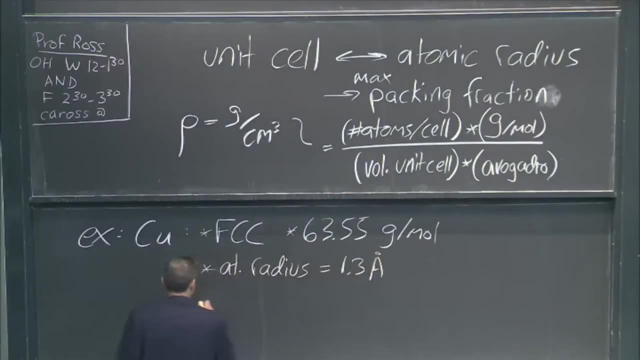 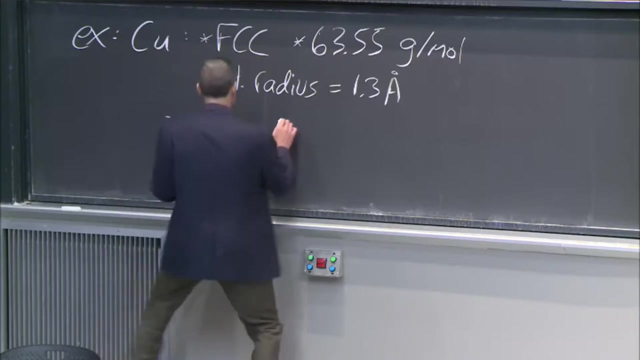 I can use the information because I know if it's a crystal and I know the crystal type And I know the FCC, then I can use this information to get other aspects right, So other properties. So for example, I know that the radius of the atom for an FCC if it's close packed 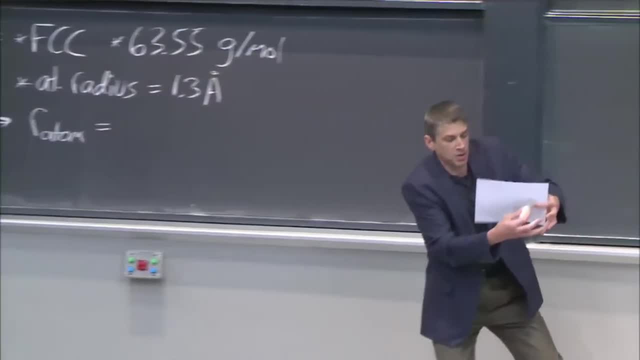 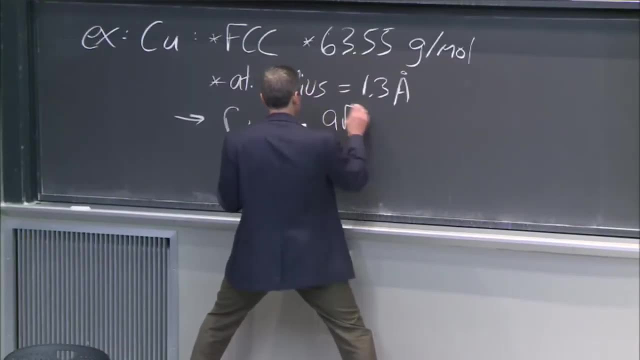 If it's FCC- one element, remember. it grows out until they touch right And that got us how we get the radius of the atom And it's A root 2 over 4.. Well, I also know that there's four atoms. 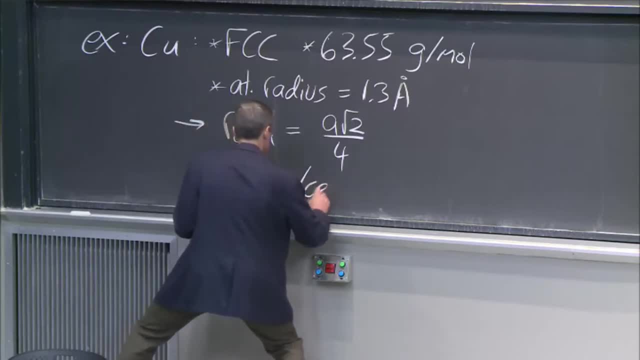 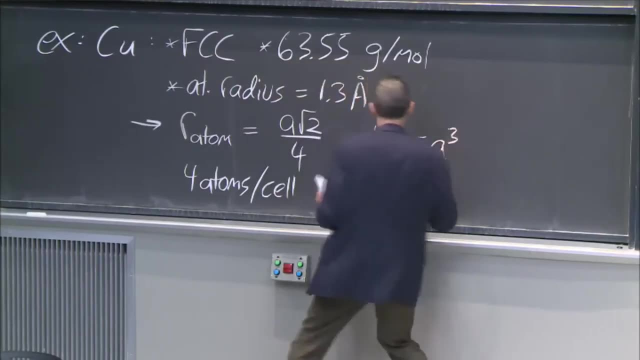 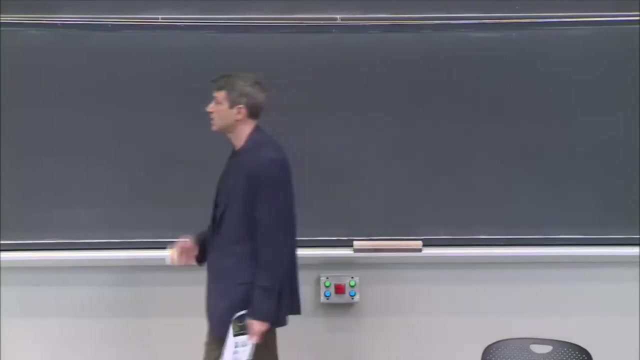 atoms per unit cell, because it's FCC. I also know that the volume of the cell is simply the lattice constant, cubed because it's a cubic cell. All the ones here are cubic, So the volume of these cells are a cubic. From this information I can compute the density. 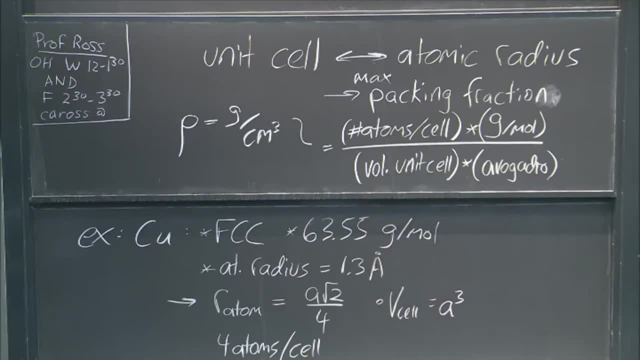 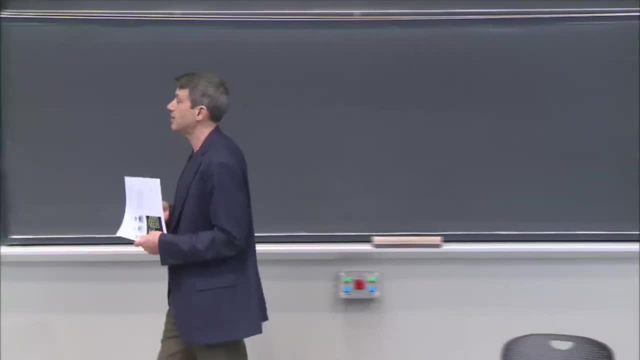 So again it's going back and forth: The radius of the atoms packed in the lattice constants, the number of atoms in the cell. these are the things we talked about on Monday, And as you go back and forth you can do things like this: 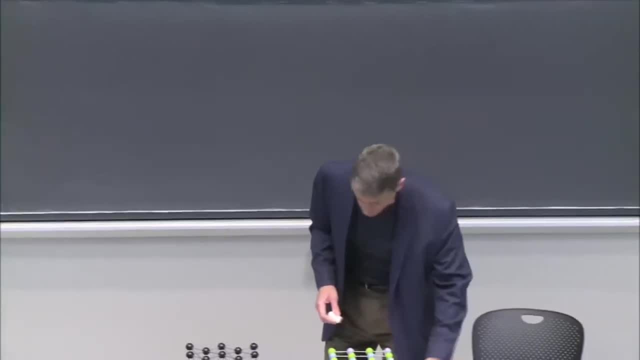 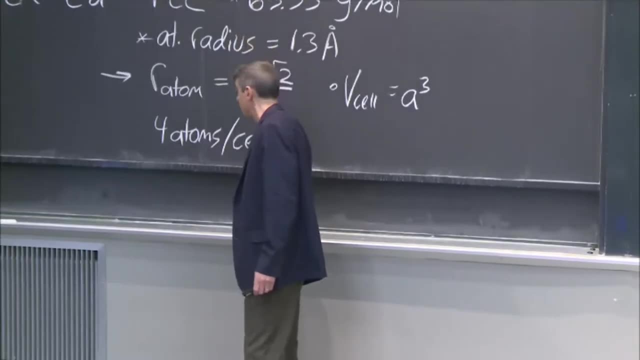 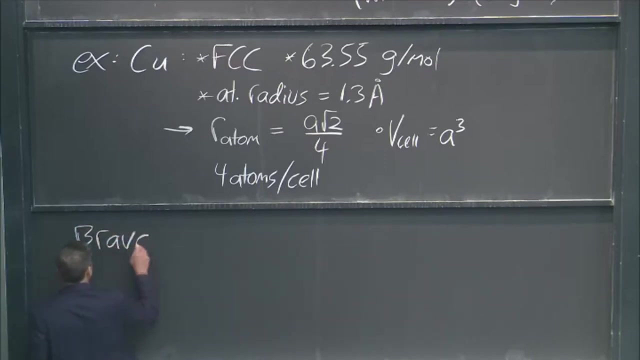 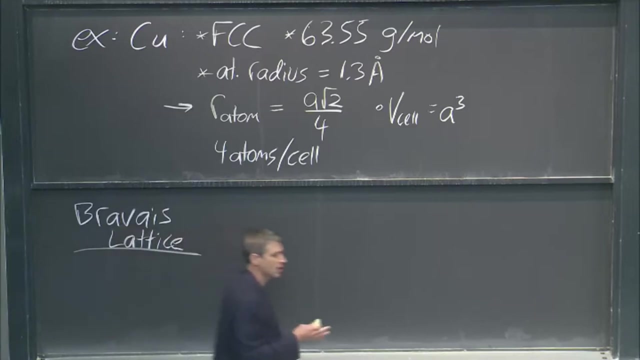 All right, good, OK now we talked about the Bravais lattice there, And those are three Bravais lattices that I want you to know- Bravais lattice. But the thing is that There's something else you need to know in order. 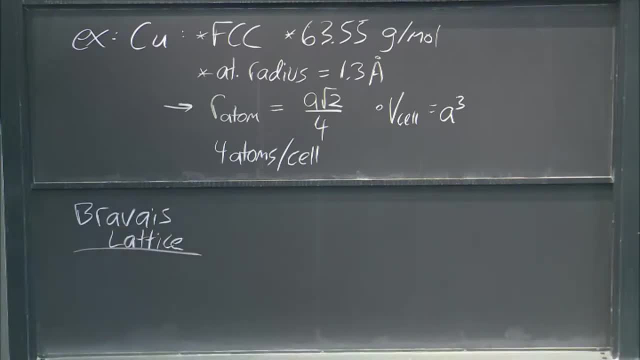 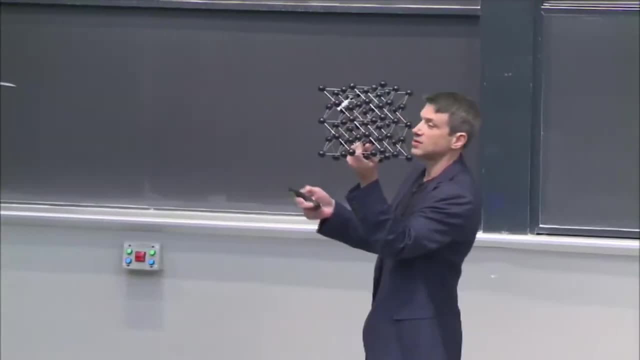 to know what crystal you have. And so this is the FCC Bravais lattice. There it is. It's over there on the right, It's the face centered cubic. OK, Gesundheit, And I'm going to pass this around. 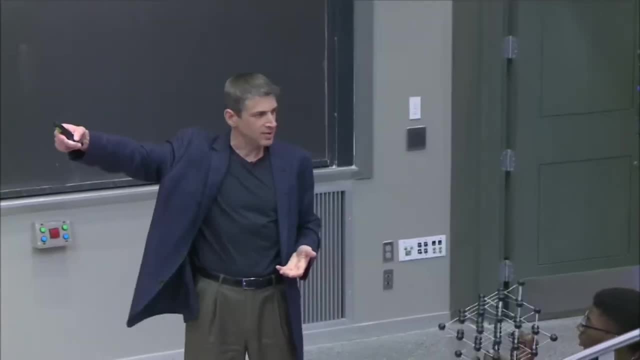 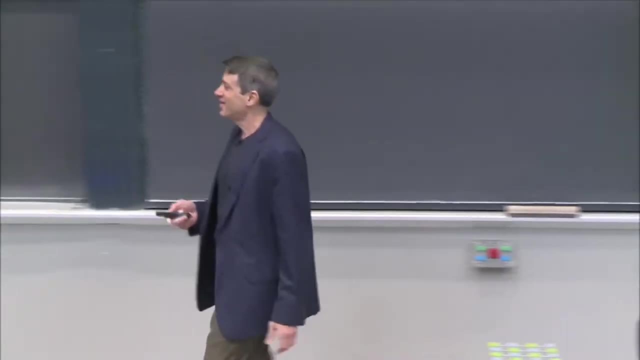 Oh yeah, I'm starting over here because I keep on starting over there, And it's not fair, That's not right. Yeah, All right, got a couple, OK Now. OK, so that's FCC, right. So we're going to write down FCC. 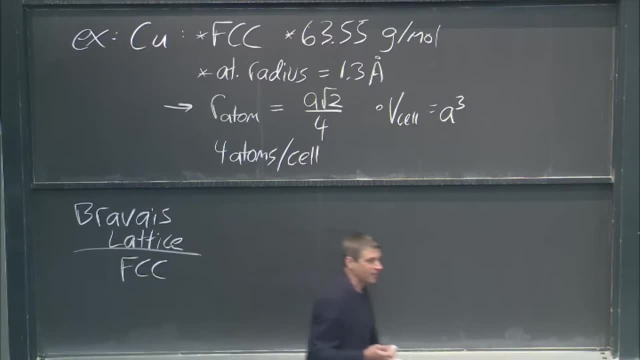 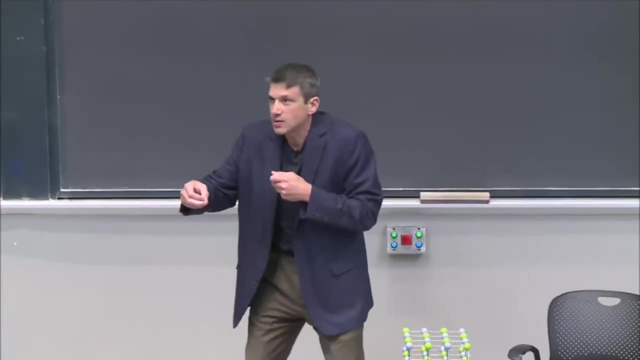 But the thing is that, see, this is a stamp. Remember, we emphasized this on Monday. It's a stamp of points that are equivalent. That's what the lattice vectors are. They are not the things that you put at that point. 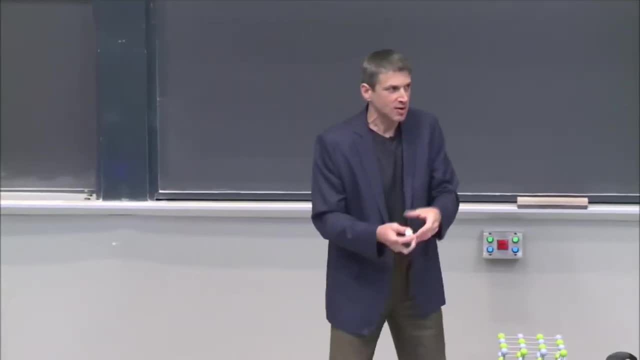 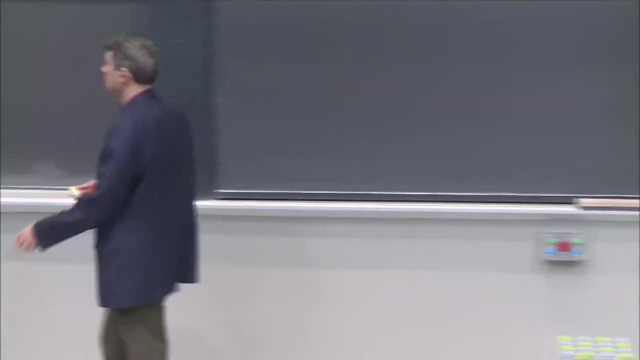 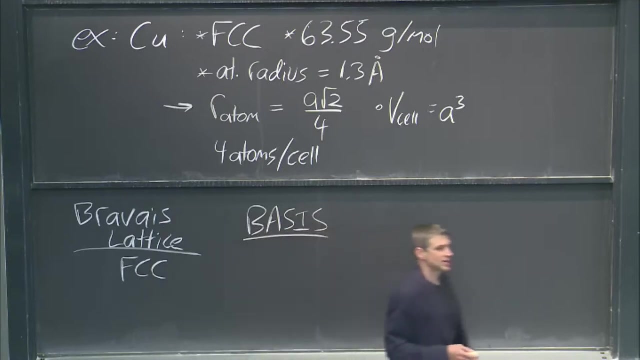 That is something else. Now, on Monday we put the things. there were atoms, spherical particles, And they're all the same. That was our introduction. That was our introduction to crystallography. But the basis can be more than just a single atom. 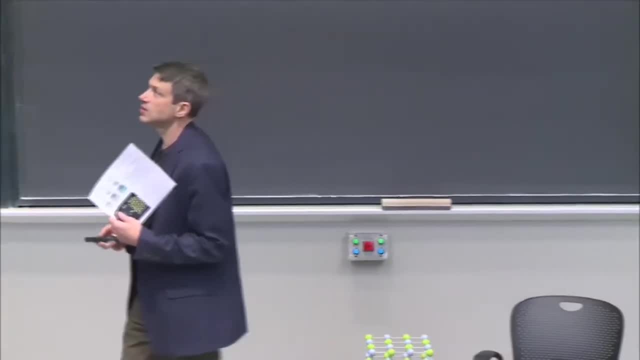 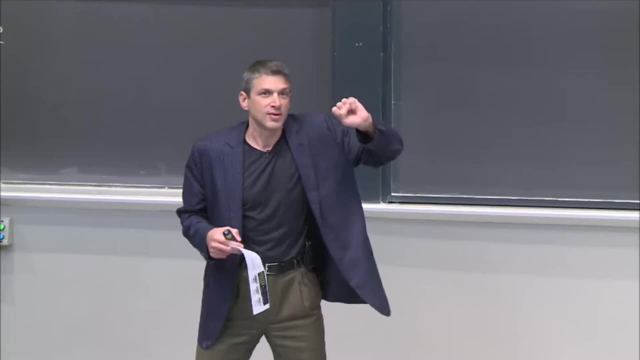 It can be more. So how do we think about the basis? So here's a lattice. This is a lattice of points. I haven't. The way you want to think about a lattice is a stamp without putting things there. yet The basis is what you put there. 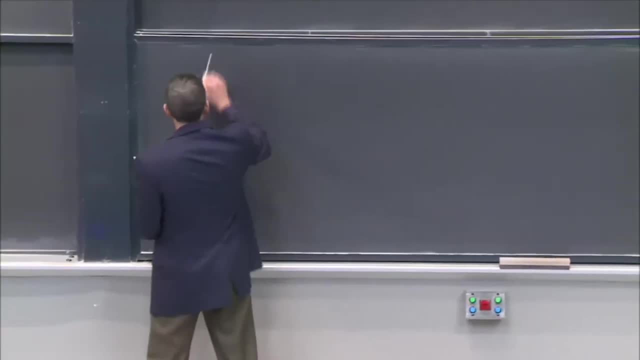 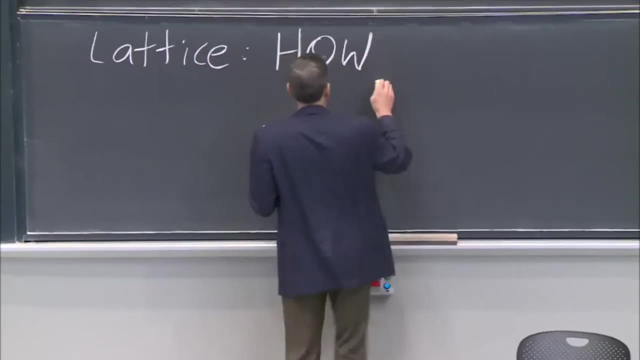 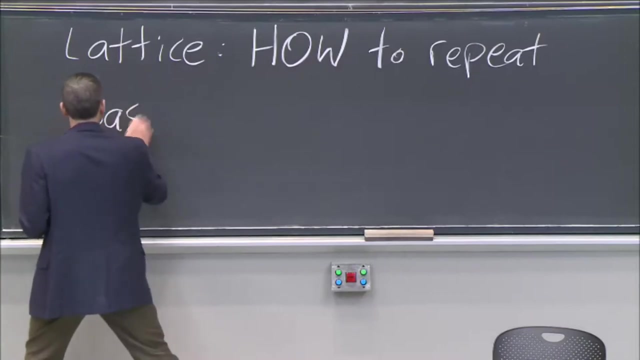 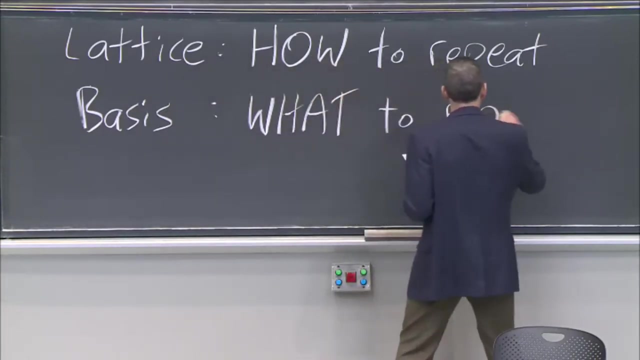 Let's write that down because it's so important, OK, So the lattice is all we're going. oh, I'm going all caps. How to repeat? OK, And the basis is what to repeat? OK, So if this is my lattice and I decide. 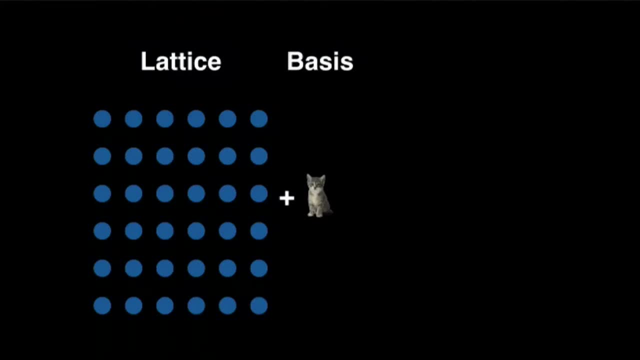 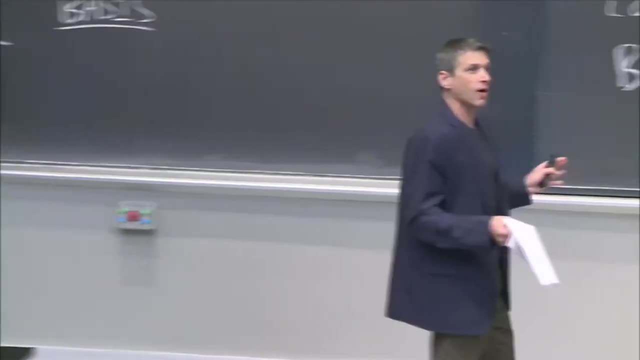 that I want to get a million downloads on YouTube. I'm going to put a cat there And this is my crystal. It's a crystal of cats. That's OK. I have done nothing wrong, Because I have simply according to the rules of crystallography. 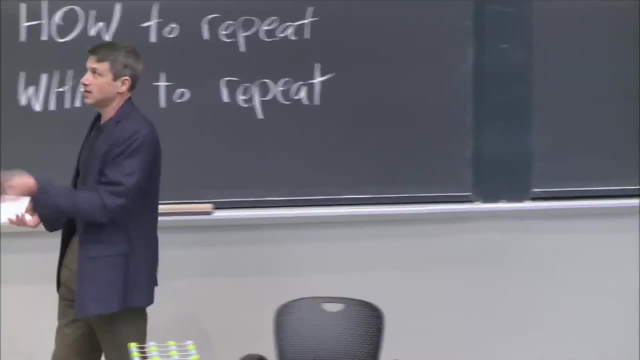 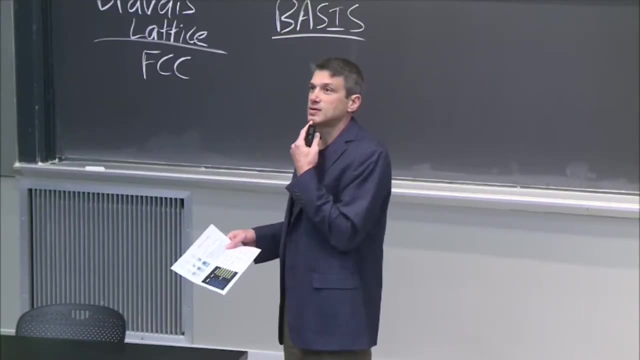 I've had a lattice and a basis, And I've just defined my basis as a cat And that's the crystal you get. But see, the basis could also have been, for example, two atoms colored differently to show that they're different atoms. 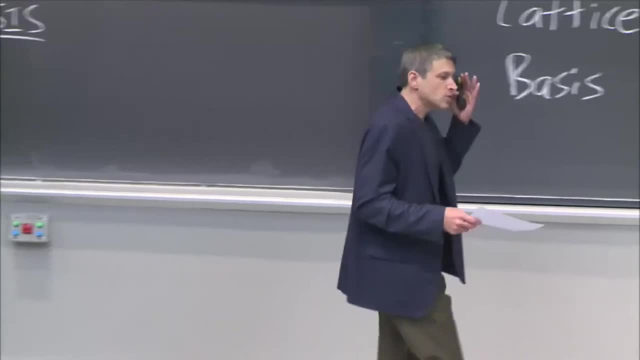 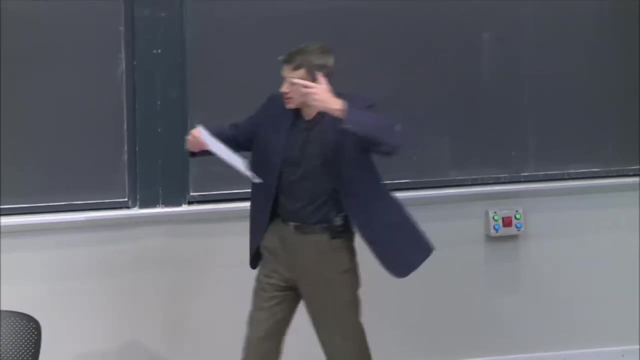 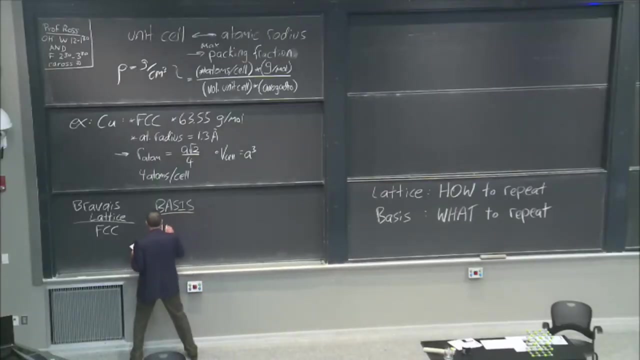 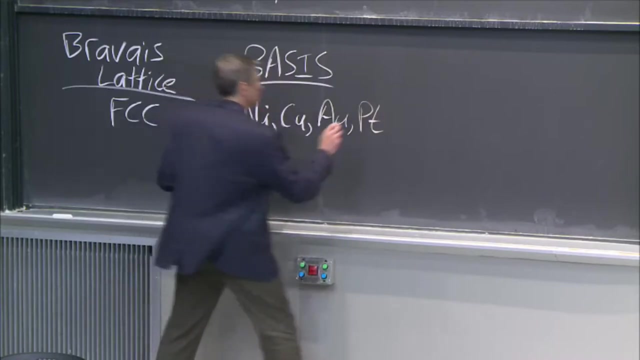 And then this would be my crystal. So the actual crystal that you get may be different than the lattice structure. So let's take a look. So, for example, over here, if my basis is a single atom- nickel, copper, gold, platinum- well, 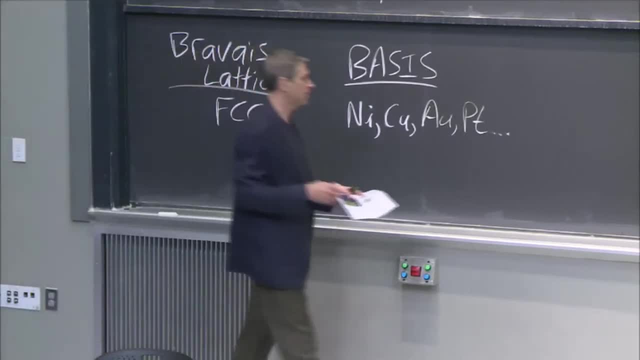 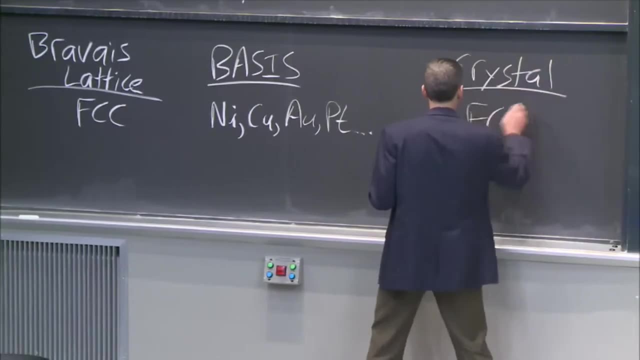 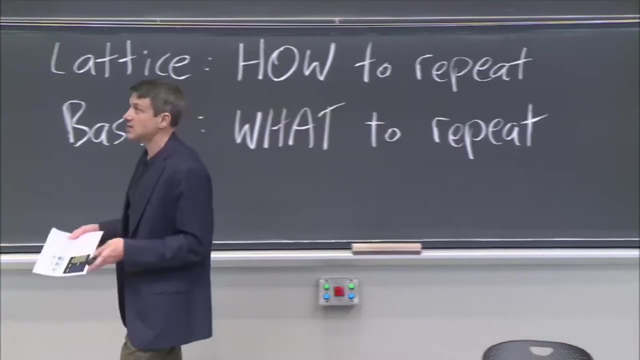 I showed you these from the periodic table on Monday. We highlighted them when we talked about FCC, Then the crystal, The crystal that you get, is FCC. These are the ones we did on Monday. Those are FCC crystals, But at the same time, if my basis, check this out. 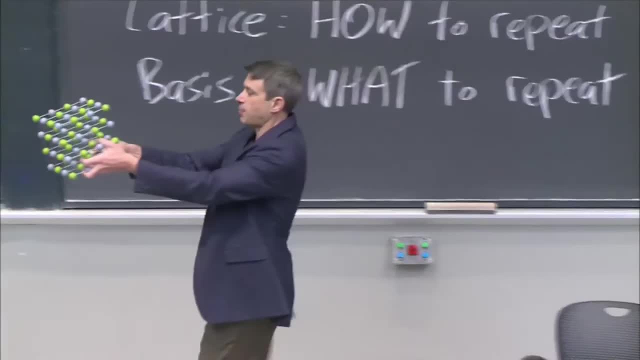 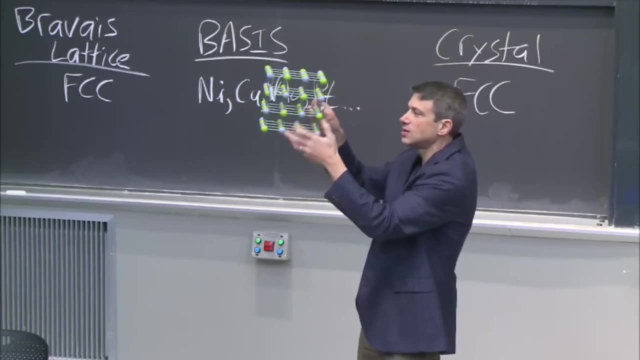 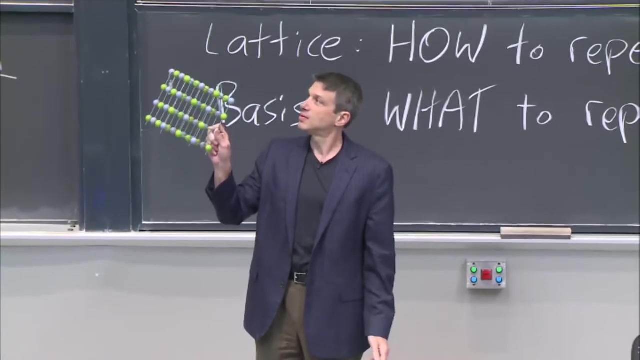 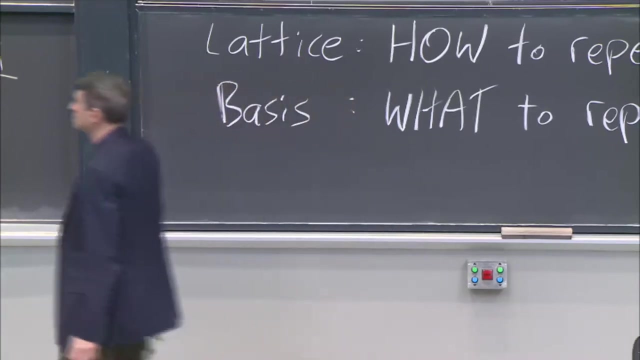 This is salt. When you guys pour salt on your food, do not see it anymore, except as this, This is salt. This is salt. It is, Let's see, Simple cubic. Is it, though, Because a lattice a simple cubic? 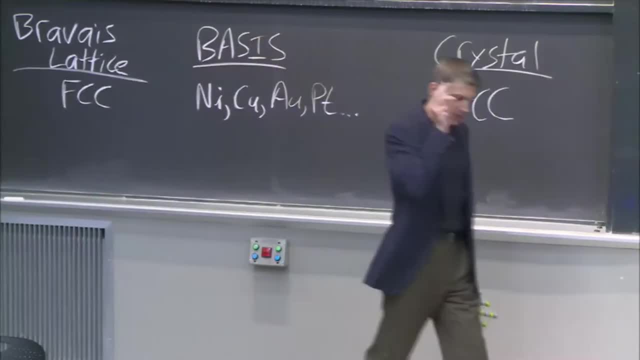 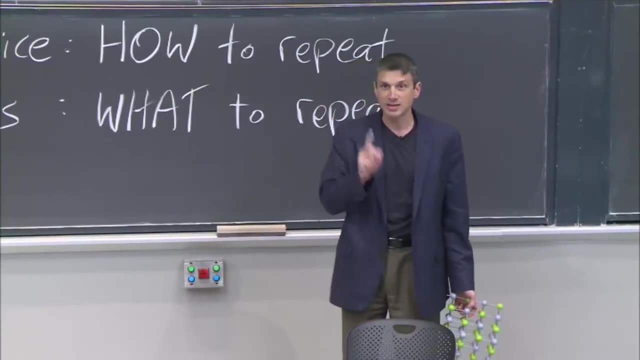 remember the definition: A simple cubic lattice would mean a stamp of a simple cube where every corner is exactly the same, Exactly the same. That's what a lattice is. So this cannot be a simple cube. This is not simple cubic, because they're different. 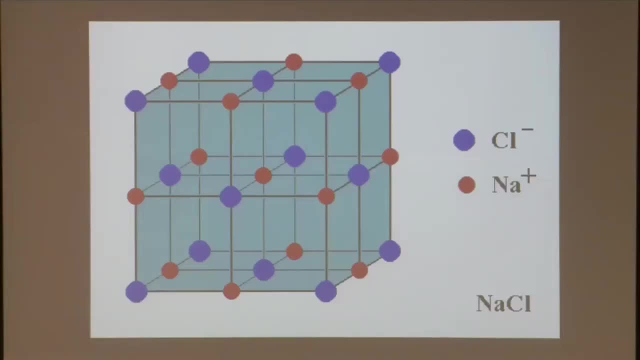 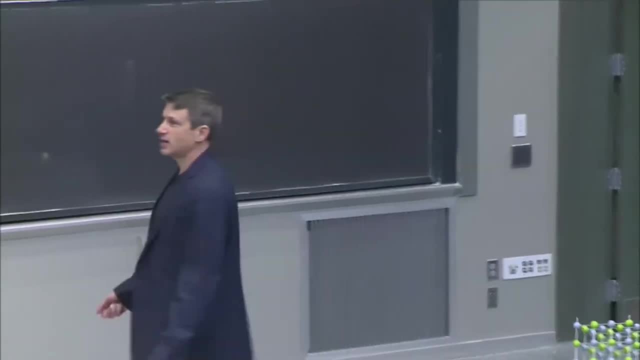 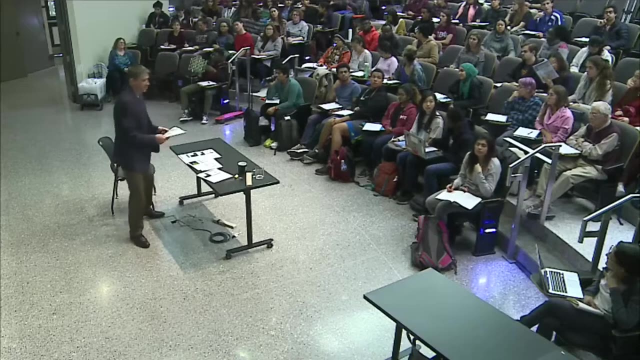 This is an FCC. Yeah, I'm starting over here again Trying to even it out. That's an FCC lattice, but with a basis of sodium and chlorine. So it's an FCC. You can call it an FCC lattice, but the basis. 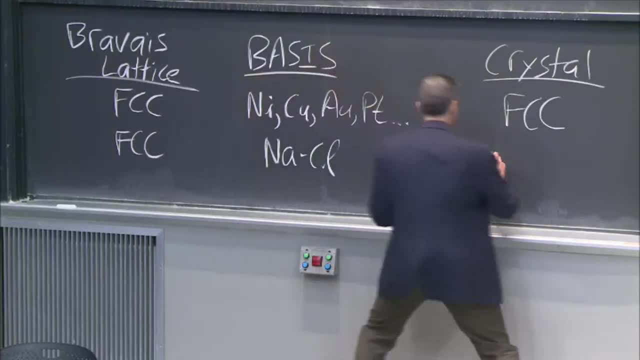 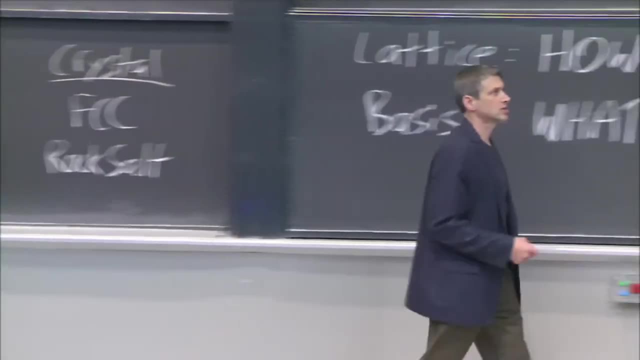 but the basis is a sodium chloride pair And this has a name: It's called the rock-salt structure. It's called the rock-salt structure. It's an FCC lattice with this two-atom basis. where, look, you can see the FCC lattice here. 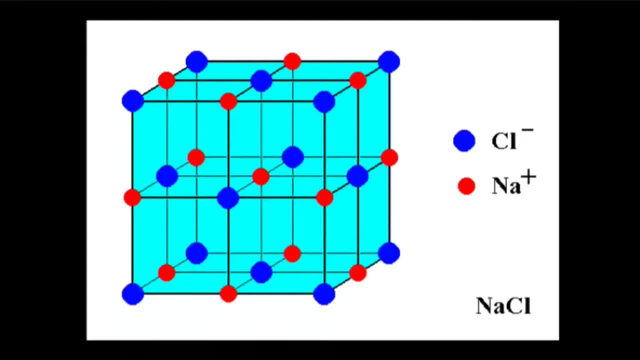 Look at those blue points right. Blue outlines an FCC lattice. But now the basis is one atom here and one there. So now I take that this pair and I put that at all the lattice points. You see that You put that at all the lattice points of FCC. 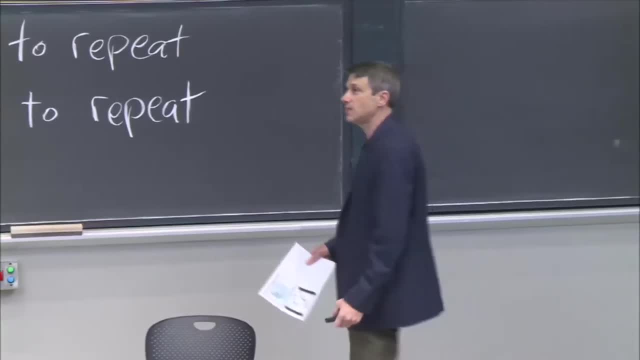 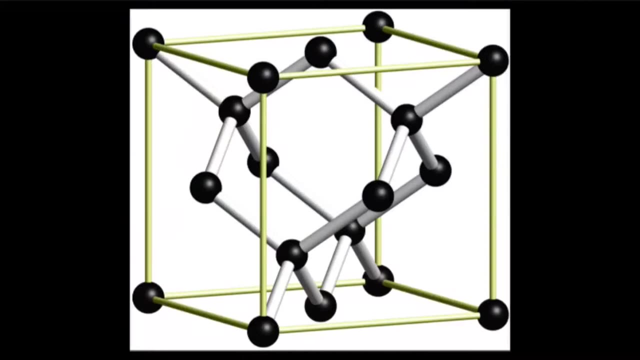 and you've got salt, And that is how you must see table salt from now on. But we talked about diamond. This is diamond. Diamond is the same Bravais lattice. It doesn't look like it at first. It doesn't look like it at first. 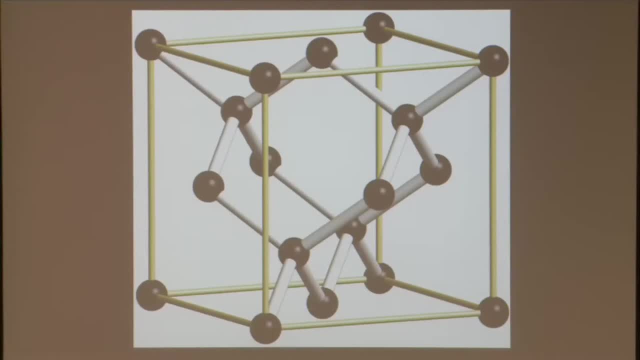 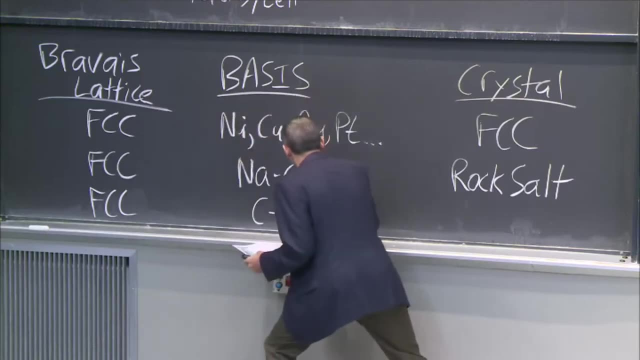 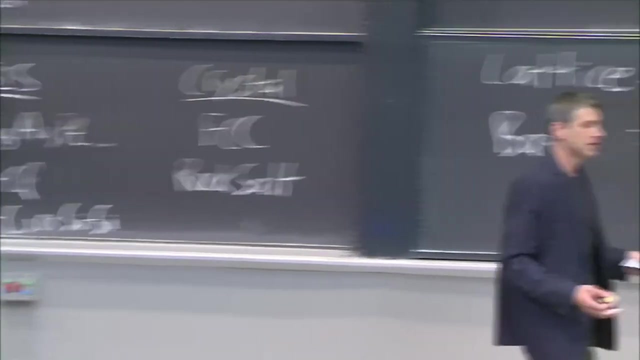 But see here, here I have a different pair, Here I have a carbon-carbon pair, Or it could be, or silicon-silicon. There are actually a number of pairs of atoms that would form this diamond. In fact, we specify because there are different types. 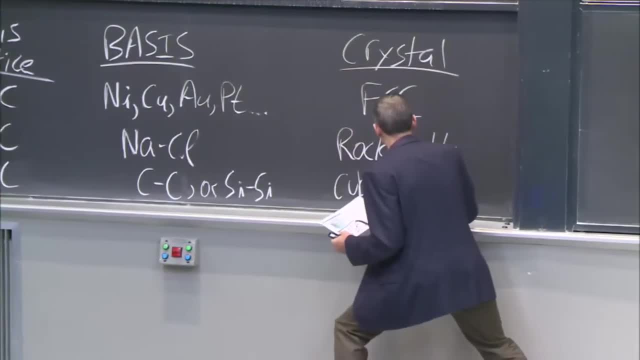 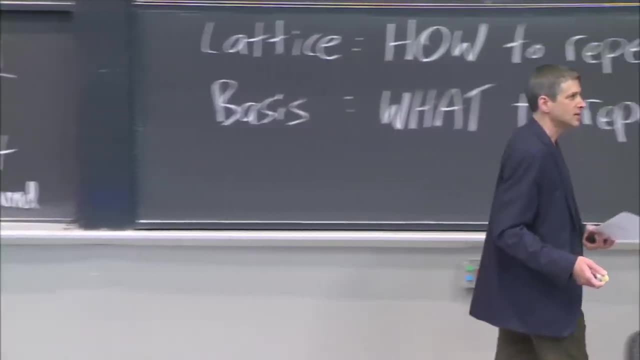 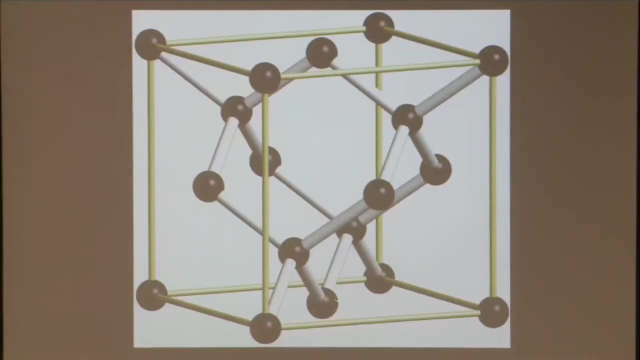 this is called cubic diamond crystal. This is the cubic diamond crystal. What is the lattice? It's FCC. It's FCC. Now, let's take a look at that. Look, There is my FCC Here here, here here, right. 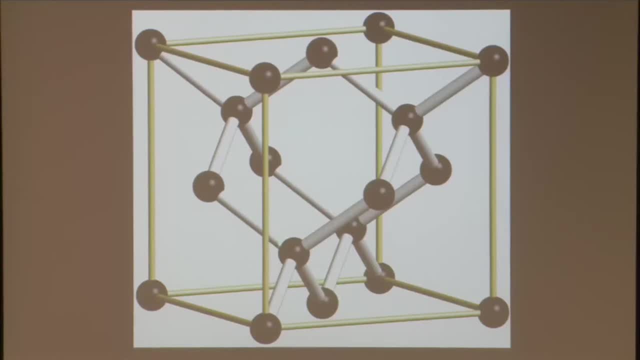 But inside of the FCC I've got this pair of carbon atoms. So now they're the same type of atom And instead of one being kind of in the middle of this edge, as it was with sodium and chlorine, now the other atom is kind of off on a diagonal. 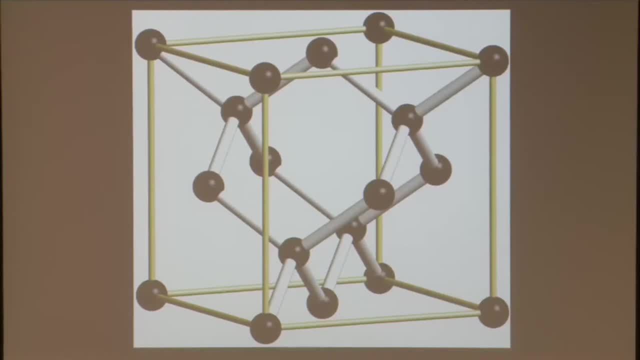 But it's still just a pair of atoms. It's a pair of carbon atoms, But if you look carefully at diamond- and this doesn't go on in this picture but it does in real life- this is an FCC lattice of these pairs. 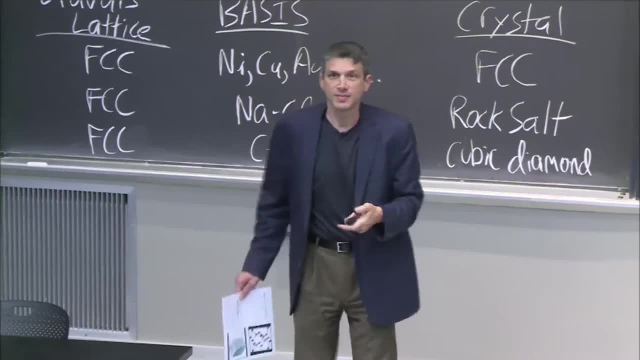 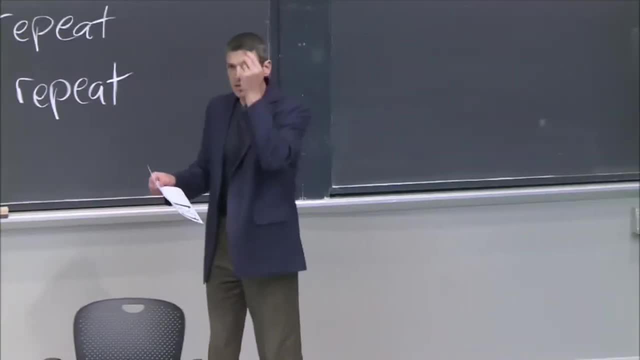 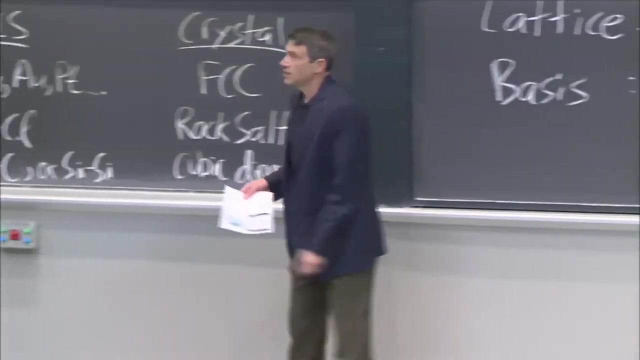 repeating everywhere. That's what diamond is. It's an FCC lattice, So the symmetry is FCC, But the basis is a carbon-carbon dimer And that gives you cubic diamond. So there's the Brabe lattice and there's the resulting crystal structure. 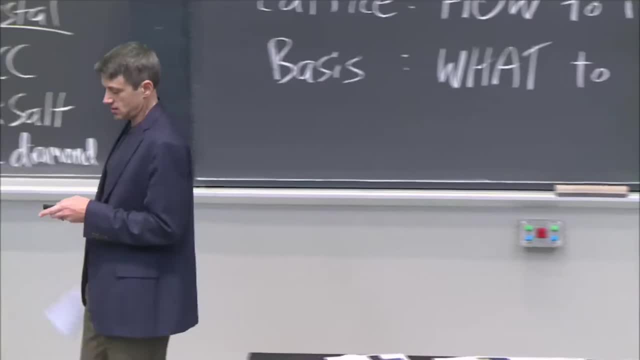 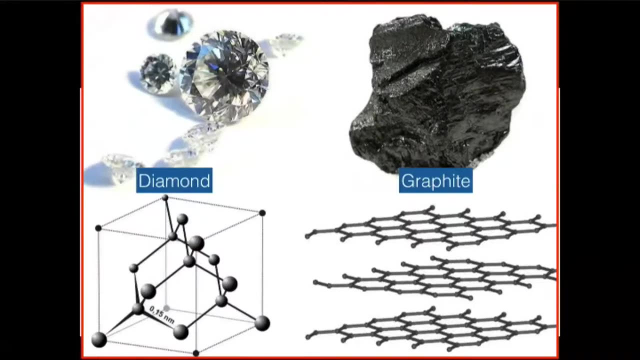 Now Speaking of diamond- And this is a graph that I showed you a while ago when we were talking about the differences between diamond and graphite, One of the things that you can see that's so important- this is the same element, two different crystal structures. 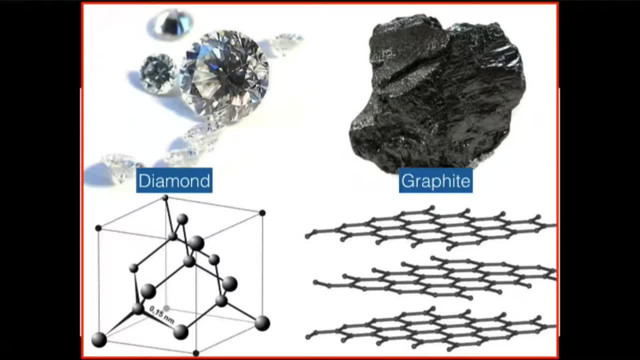 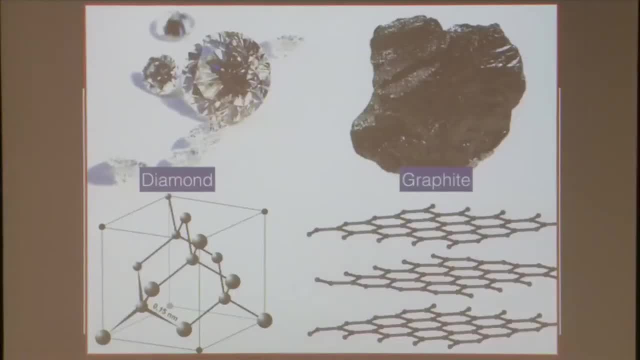 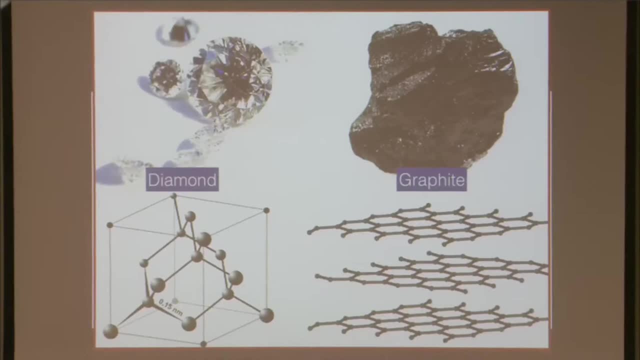 One of the things that you can see that's so important is how direction is going to be an important property. You need to know how to identify direction, Because in this case it looks like maybe if I point in different directions, the thing would look kind of the same. 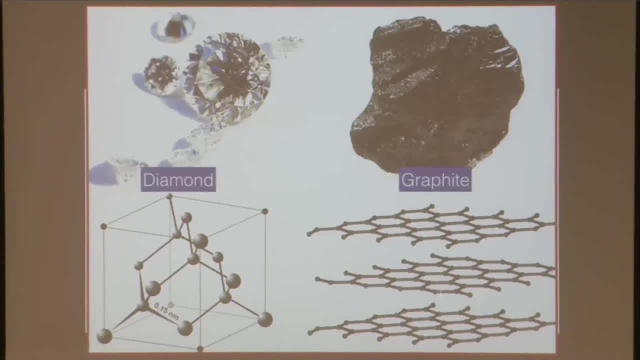 And maybe have similar properties along. But look at this, This looks seriously directionally dependent. It looks like if I did something like trying to carry charge or thermal energy this way, then it would be very, very different than if I carry it this way. 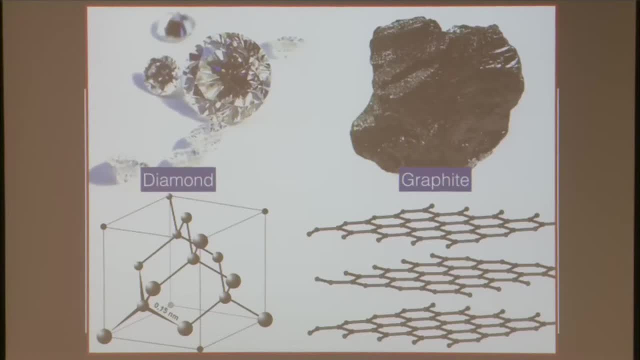 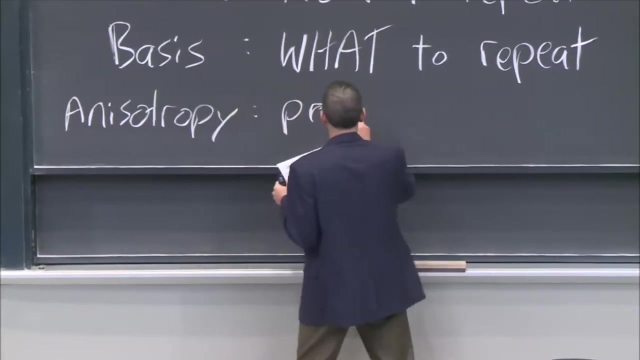 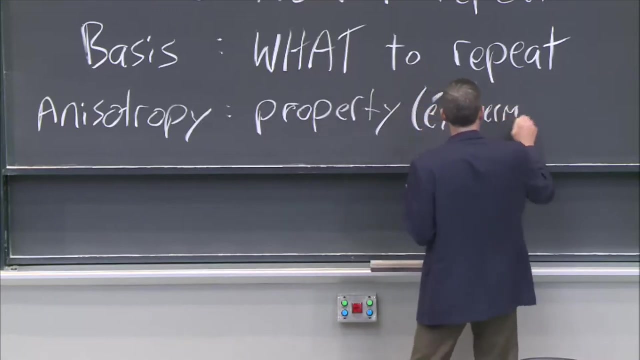 Well, we have a word for that, and that's called anisotropy. And so this is another important word: anisotropy, The property. if it's anisotropic, then the property. well, it could be like electrical or thermal conductivity, for example. 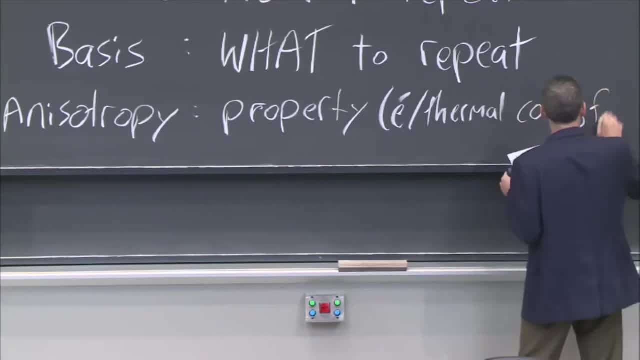 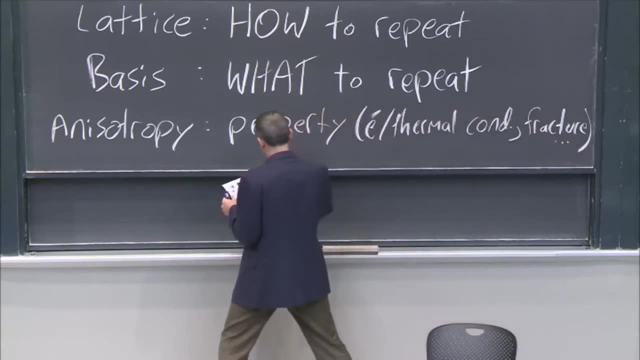 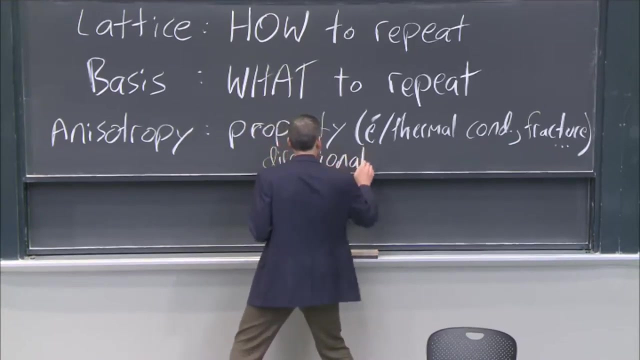 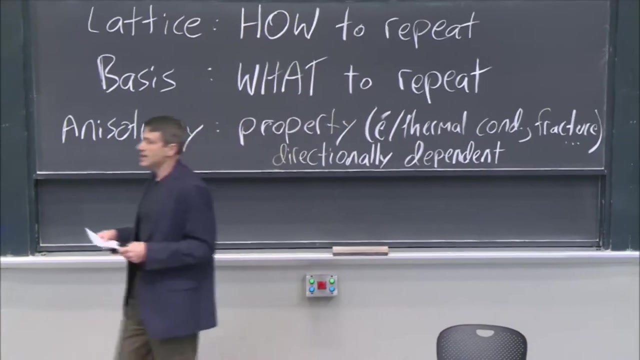 Thermal conductivity could be like how it breaks the fracture and so on, But that the property depends. I'll just say it's directionally dependent, Directionally dependent. So the reason I'm telling you this is that I now need a way. we've come up with sort of ways. 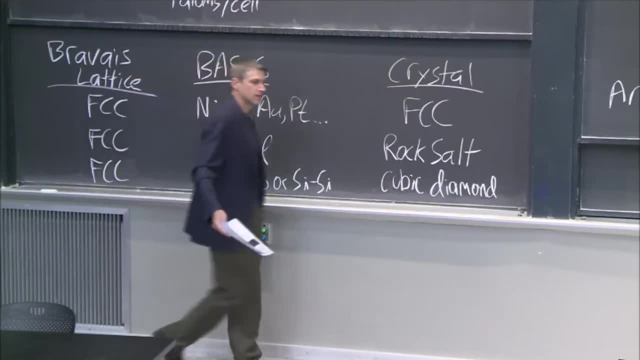 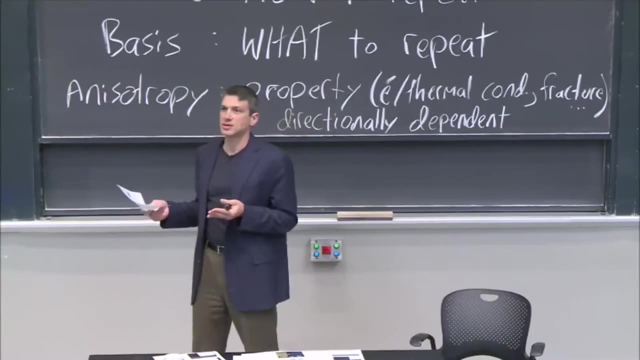 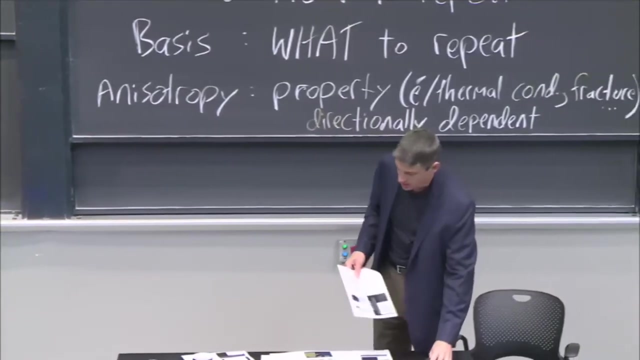 to talk about crystals, but I now need a way to specify where I am in a crystal and maybe how the crystal cuts. I need a way to talk about directionality in these crystals, And that's what I want you to. that's the topic. 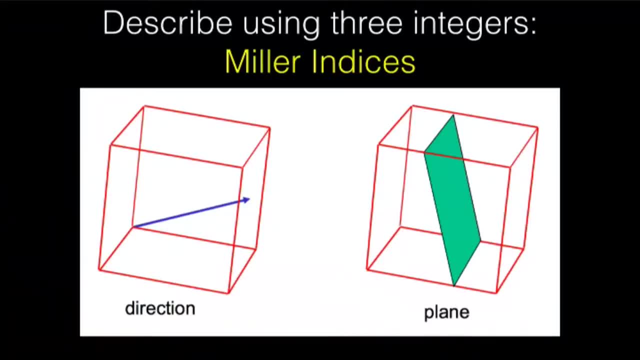 That's what I want you to do for today. So the first question, so to jump to the punchline- is: there's these things called Miller indices. That's what we're going to learn today- Miller indices, and they describe direction and cuts. 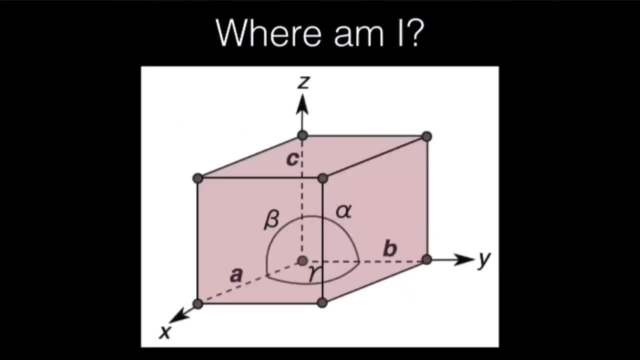 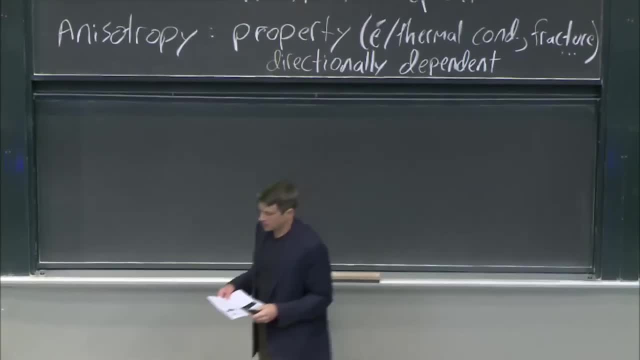 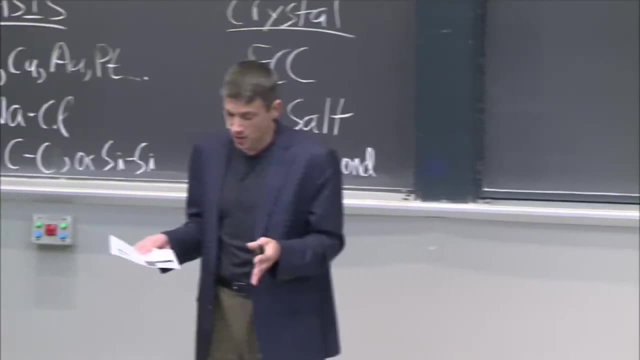 planes, OK, And the first question you can ask is: where are you Now? where are you Now? it turns out that there are these people called crystallographers, And they came up with crystallography and they have very strong ideas about notation. 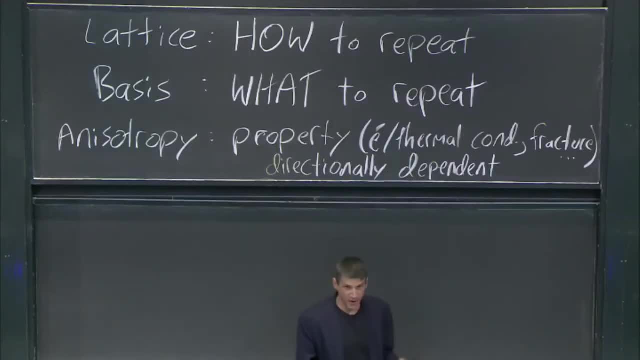 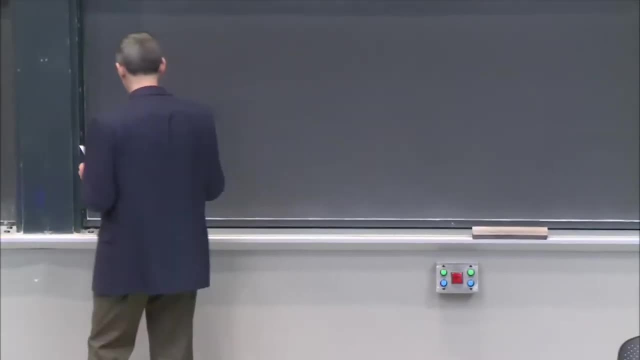 So we'll be talking about crystallographer notation And we'll be very careful not to do anything that would upset a crystallographer, because that is not something you want to see. But the first question that you could ask is: where are you? 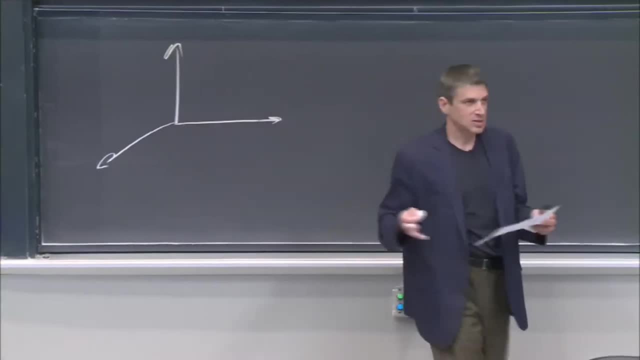 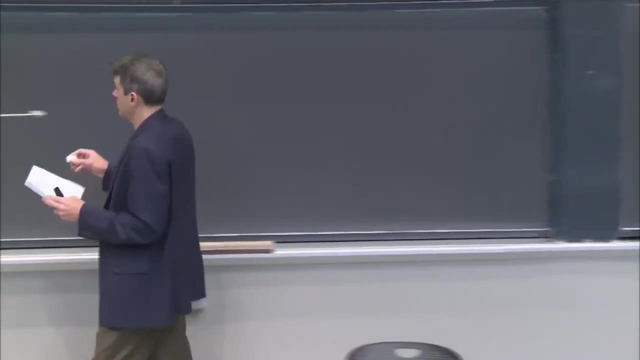 So I'm going to draw the planes, the axes, and we're always going to use the same axis directions. just for simplicity, In this class, we're going to say that, as we're talking about crystal structures, that's y. 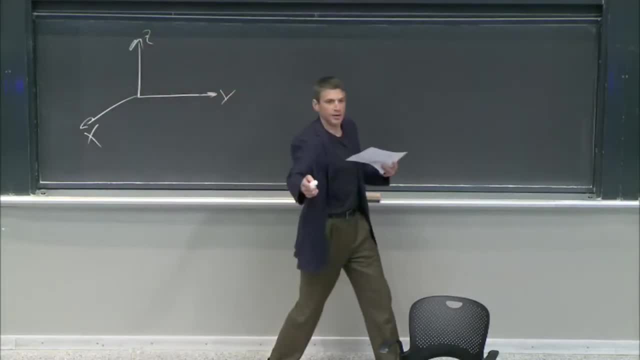 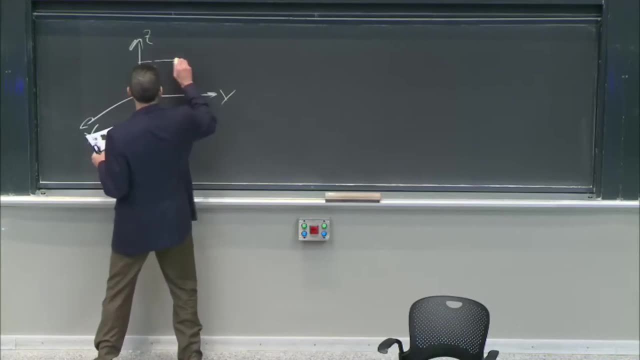 that's z and that's x. x is coming out of the board, y is going that way and z is going that way. OK, Now, if I want to know where I am, then what I can do is draw the cube. 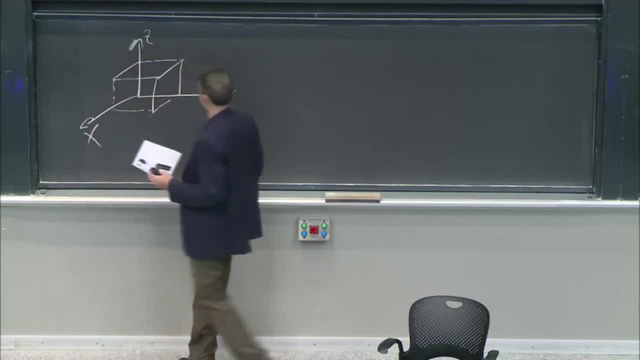 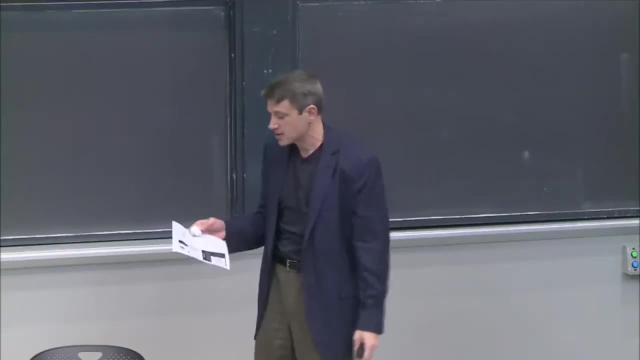 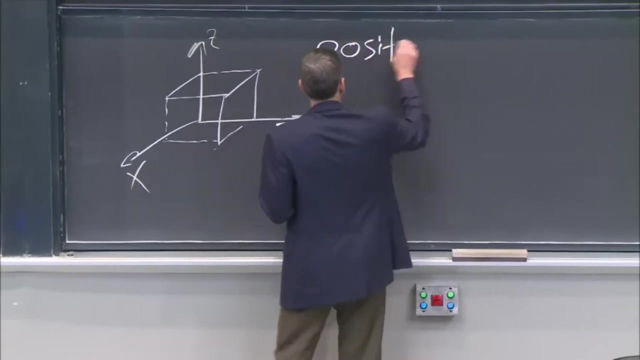 Oh boy, Here we go. OK, there it is, And I can just start looking at points. But instead of having all sorts of different numbers, crystallography And crystallographers like to work with simple numbers. So what we do is we define the position. 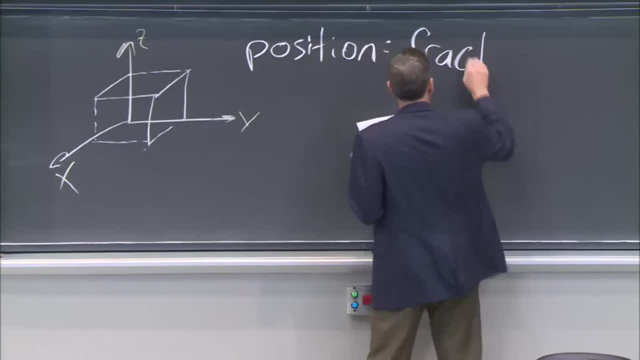 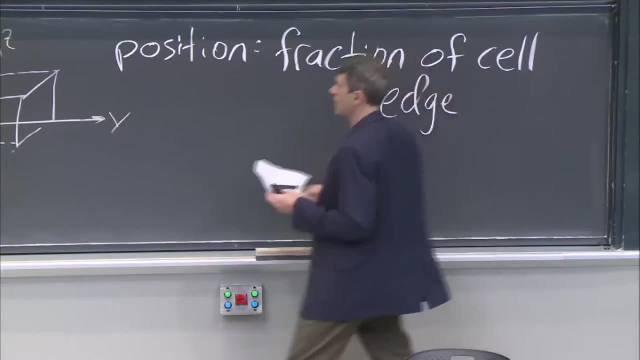 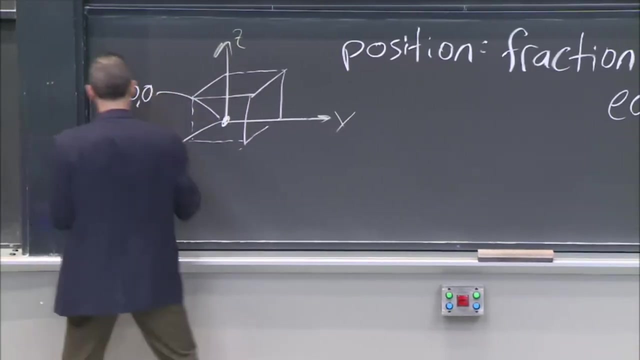 as the fraction of the cell edge. OK, so what that means is, if I you know. so, OK, first of all, the origin is 0, 0, 0, right, So that's 0, 0, 0.. 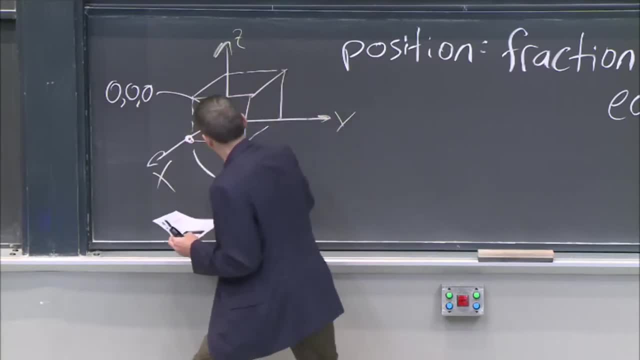 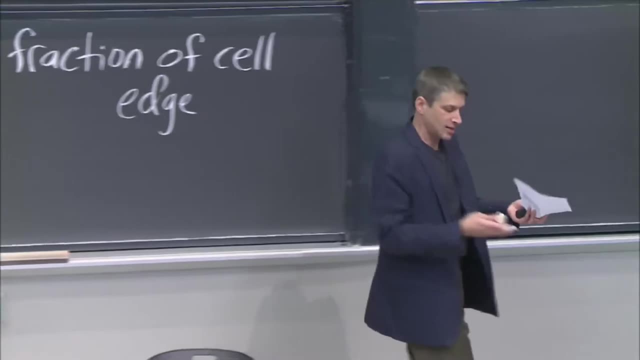 But it also means that you know, if I had this point here, that's going to be 1, 0, 0.. It doesn't matter what a is. Remember. a is the lattice constant, It's the edge of the cube which has a real value. 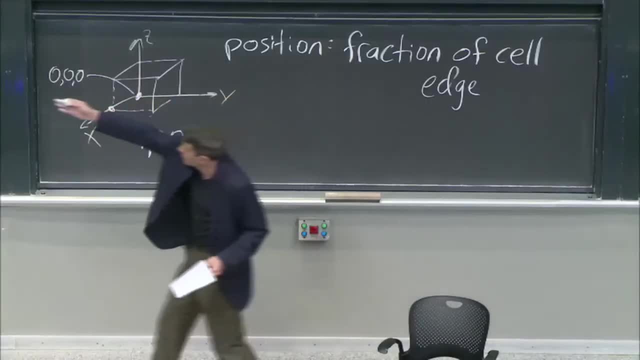 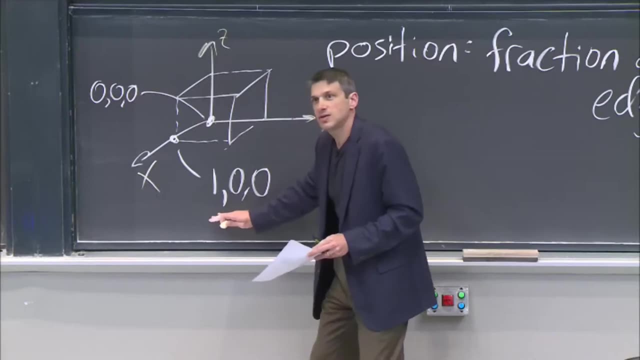 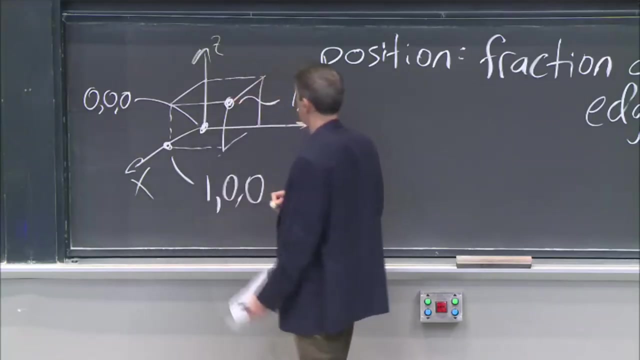 in different crystals. right, There's copper, There's a in copper which we could compute. But no, when we specify positions in crystal, we do it as a fraction of that length. OK, so that's fair. So this point, for example, would be 1, 1, 1 out there. 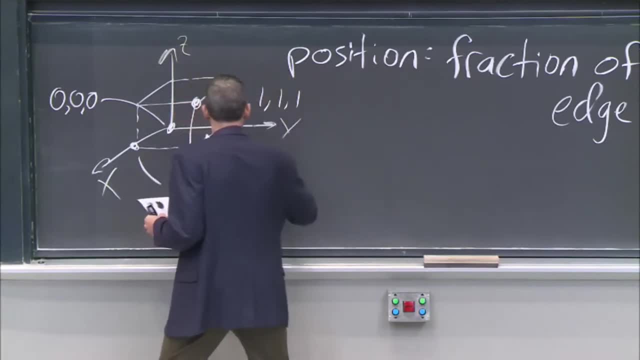 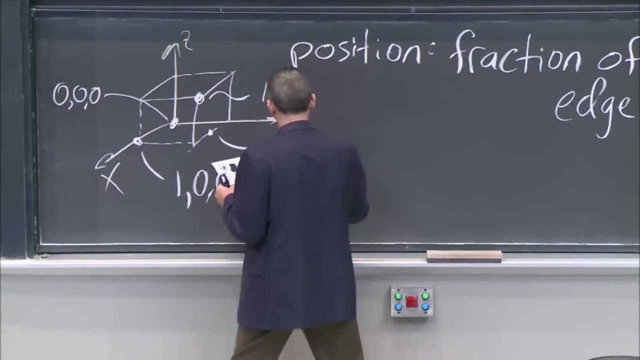 All right, And let's do one more, This point here, right, well, that's going to be Gesundheit, That's going to be, you know, OK, over a half now. So it's a half, and then 1, 0.. 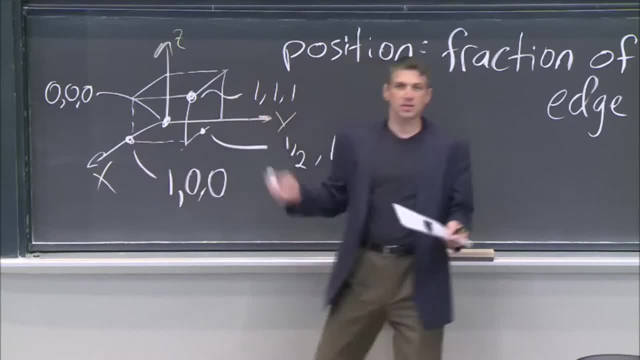 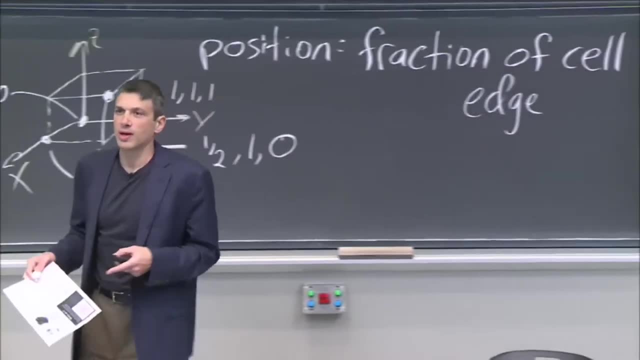 It went over a half, over 1, up 0. So it's a half. OK. good, This is just where we are. We're just getting warmed up, But really what we need to know is where we're going. 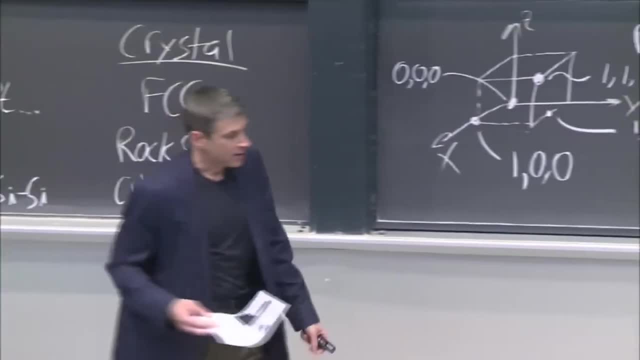 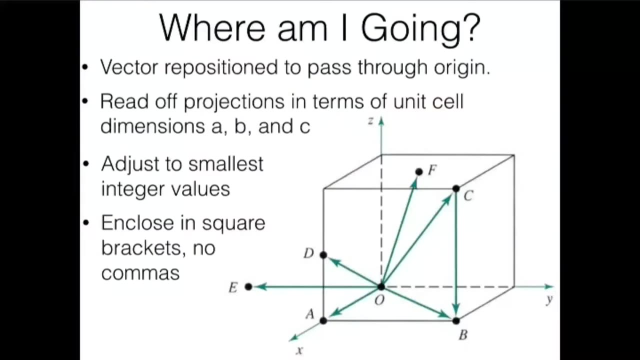 And that goes from a point to a vector. OK, now again, there are some things and some fairly straightforward rules that we follow. Not that we don't know what vectors are. We know what vectors are. The point is, do we know how to specify a vector in a way? 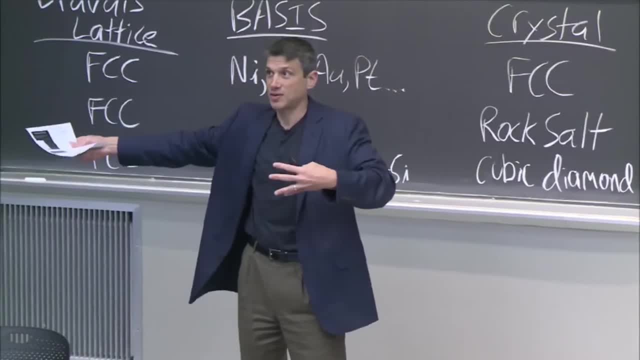 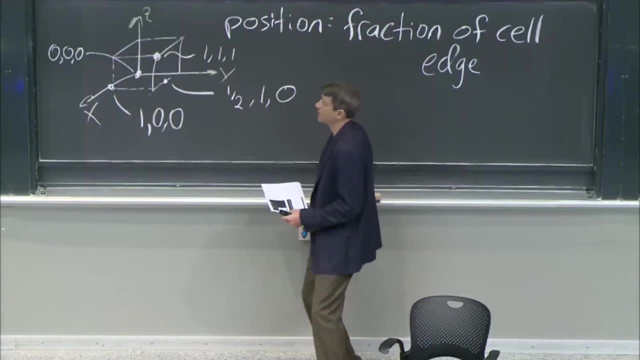 that a crystallographer would be happy with. That's what we have to learn, Because, again, we don't want to make them upset. So there is a set of very simple rules that you can follow, And I've got this for the direction. 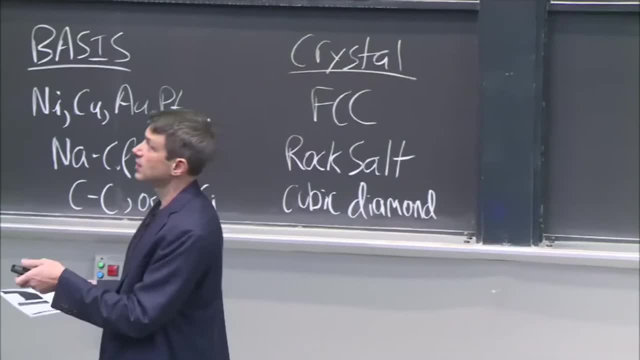 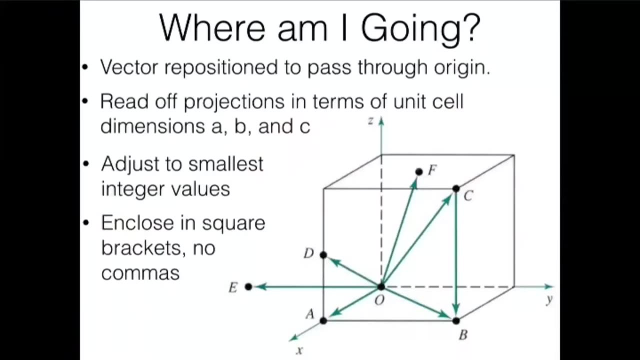 and I've got this for the planes. So here are the rules for the direction. Here's a vector in a crystal Origin O and here are different vectors, And what we do is we position it to start at the origin and then we read off the projections in terms. 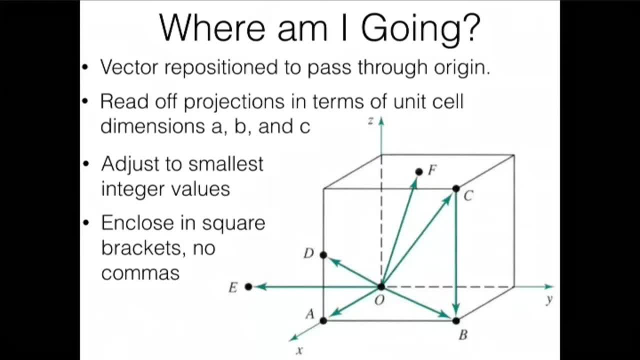 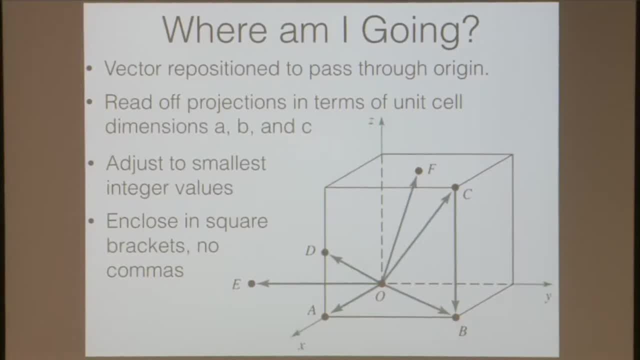 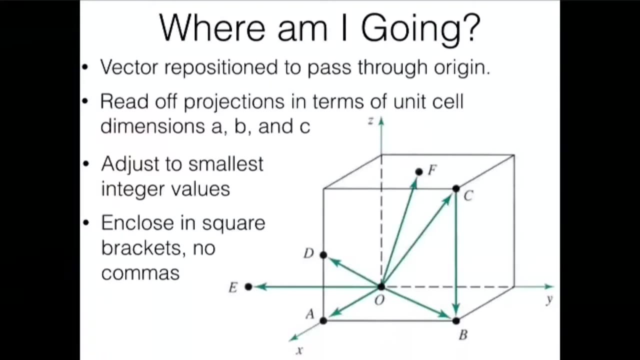 of the unit cell dimensions: A is x, b is y and c is z. Now we know that those have the same length in a cubic crystal. Adjust to the smallest integer values- That's really important- And enclose in square brackets. 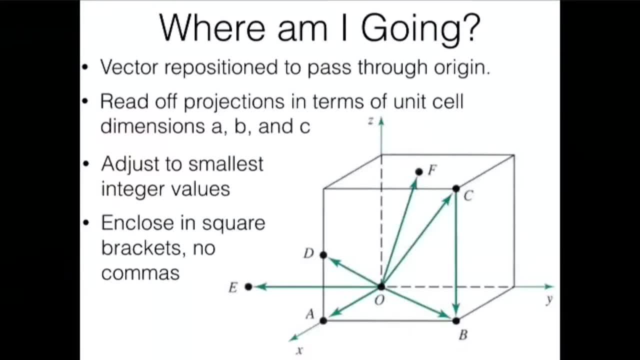 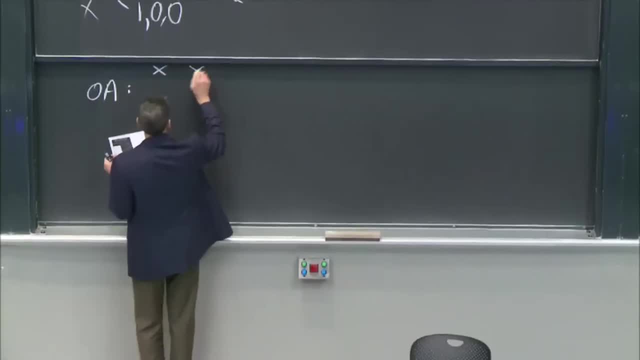 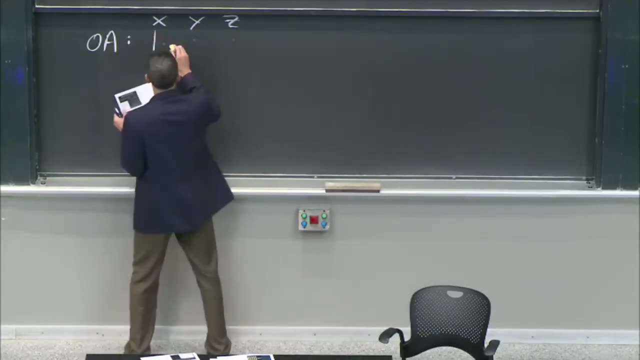 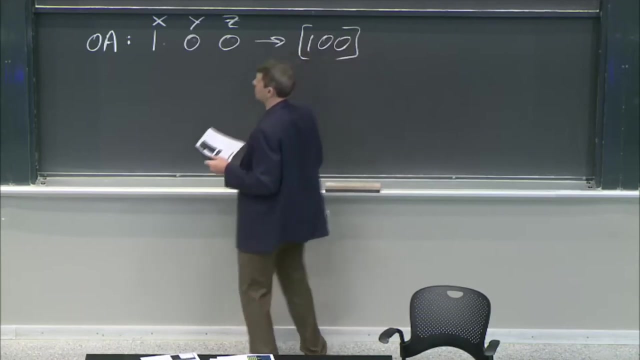 No commas, So let's do a few. So, OA, here are the x y z. the x y z readout: Well, this is 1.. This is 0.. This is 0.. So this would give us this as the notation for the OA vector. 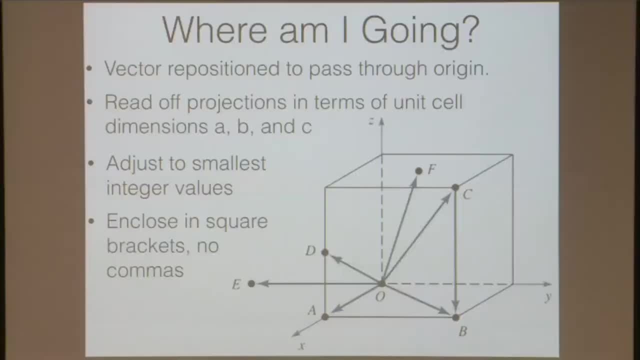 You see that there, right Notice, I've already done step 2.. So the second bullet there read off projections in terms of unit cell dimensions a, b and c, Because it went all the way to the edge. So it's a 1.. 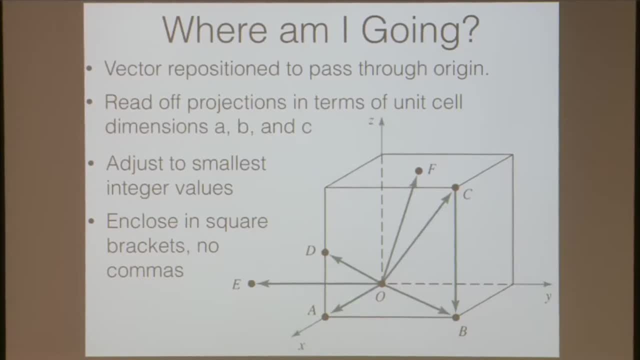 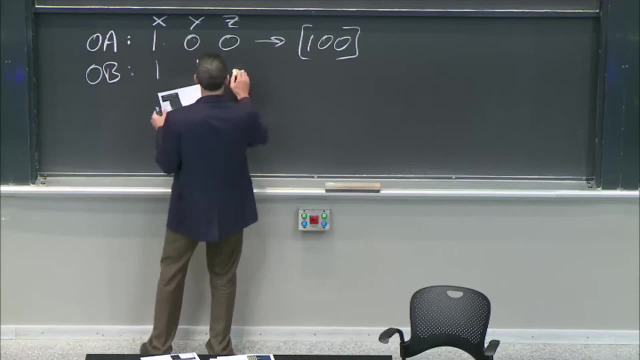 It didn't go halfway. It's not a half right. OK, good, So OB. OK, well, that's going to be 1 along x, 1 along y and 0. So that direction would be written as the 1,, 1, 0.. 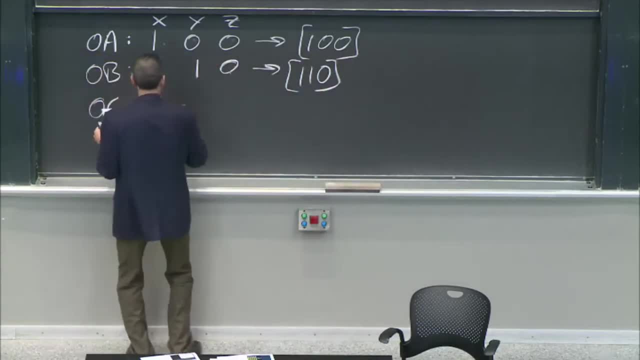 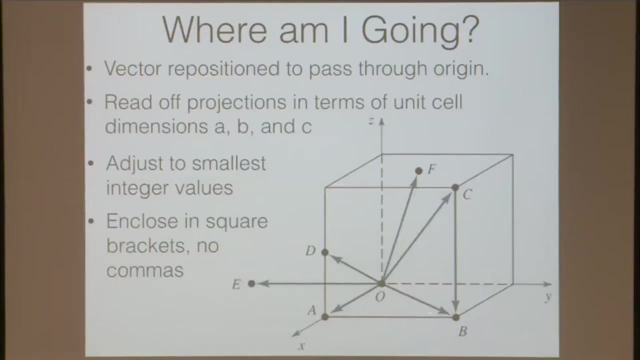 And OC would be 1, 1, 1.. This is feeling kind of boring, Oh Gesundheit. But it gets exciting in just a sec, Because all we're doing here is we're going OK, 1, 0, 0, 1, 1, 0, 1, 1, 1, OK, good. 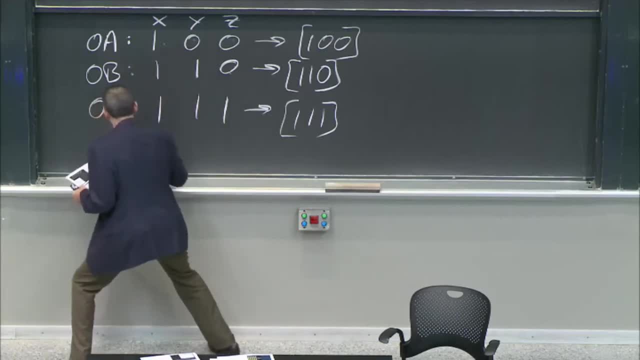 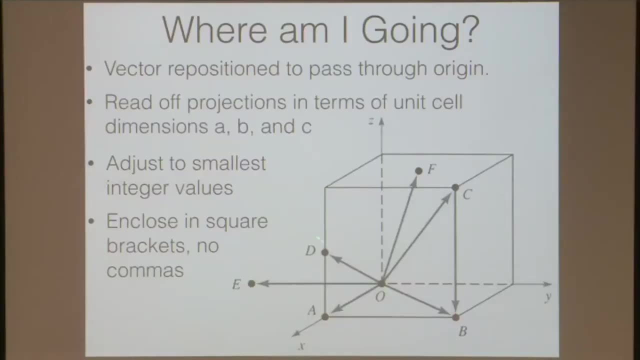 But now we go to OD. Now, OD is one of these cases where we have to be careful. So OD, you see that It's going from here to there Along the x direction. it's still going a full 1 of the edge. 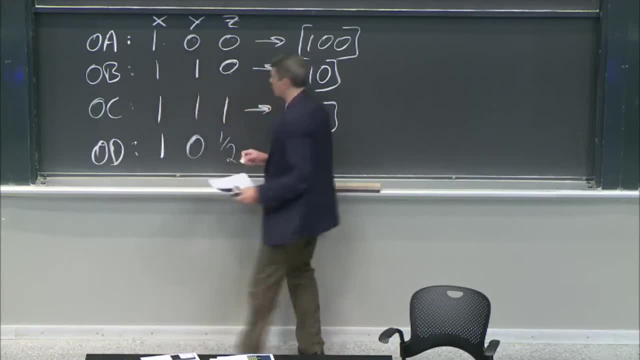 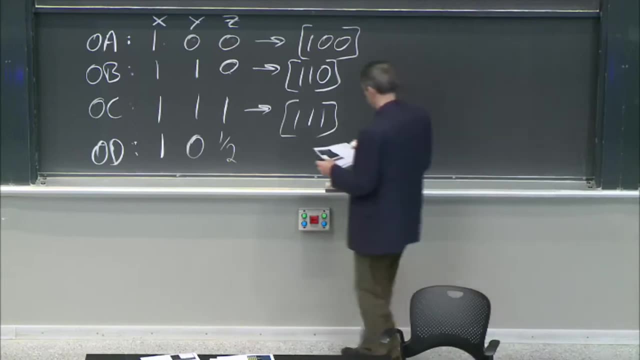 Along the y direction it's 0.. Oh, but along the z direction it's a half, And so because crystallographers don't like fractions when they talk about directions, we have to scale that up, And so we just get rid of it. 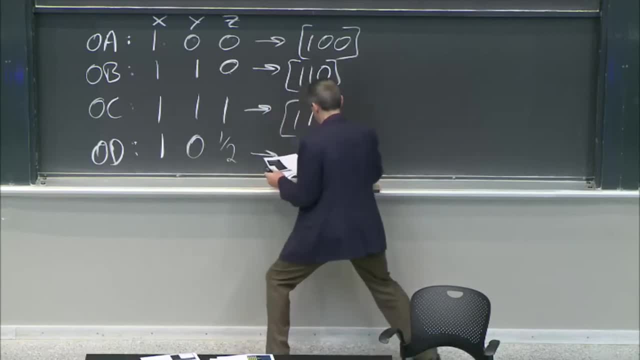 We multiply everything by 2.. We put it in brackets And everyone is happy. 2, 0, 1.. That is the 2, 0, 1 direction in this crystal. That is the 2, 0, 1 direction. 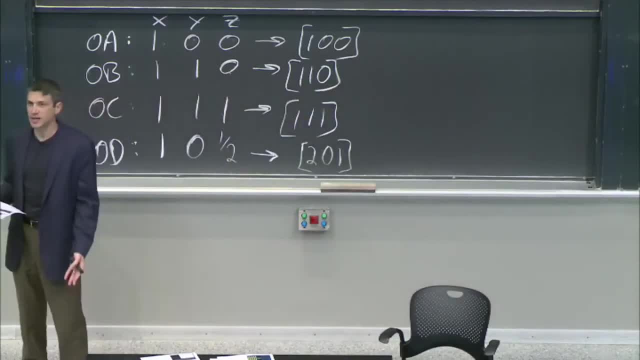 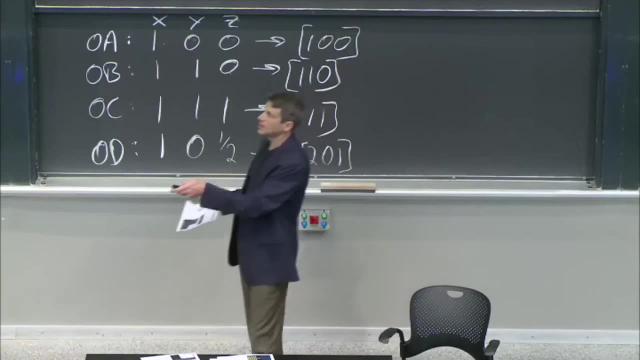 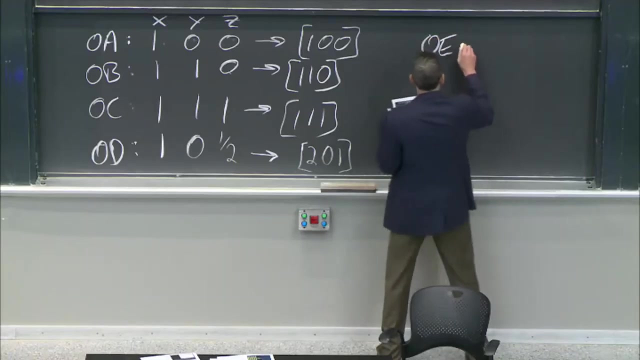 They don't like fractions. They don't like negative signs either. They don't like negative signs. So if I were doing OD, if I were doing OE, OK, that's just going in the other direction. So OE would be, let's see, minus, OK, well, 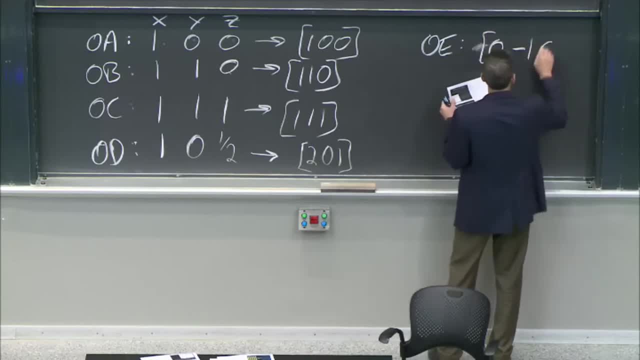 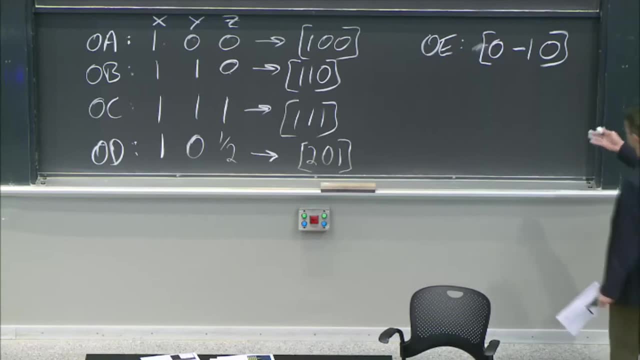 if I just jump to what we think it might be given what we just saw, it would look like that. But crystallographers don't like having negative- you know these- minuses inside of their brackets, So we write a bar. 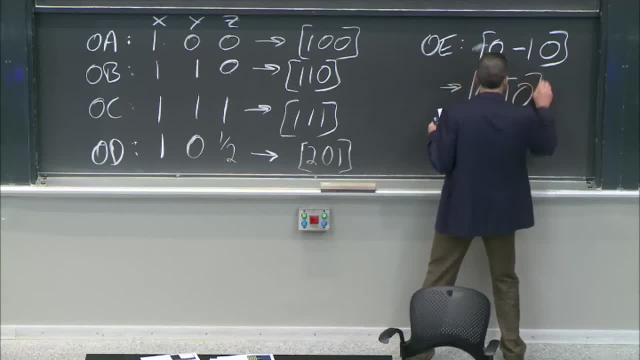 So we write it like this: 0, 1, bar 0. And that is the notation for going in the negative direction. OK, 0, 1, bar 0.. That would be OE. Did I get that right? 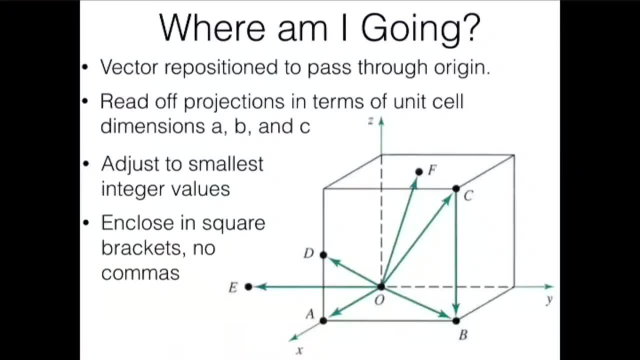 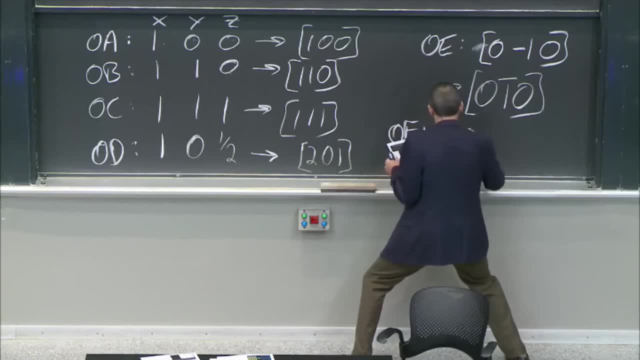 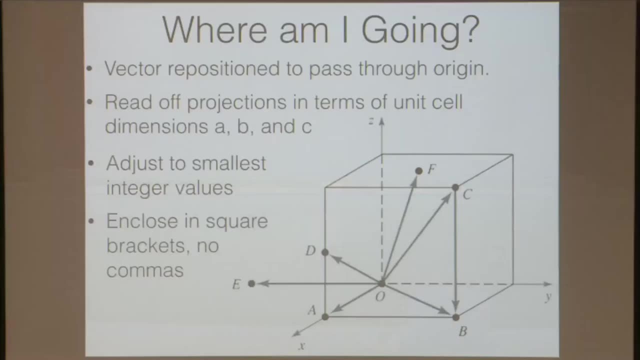 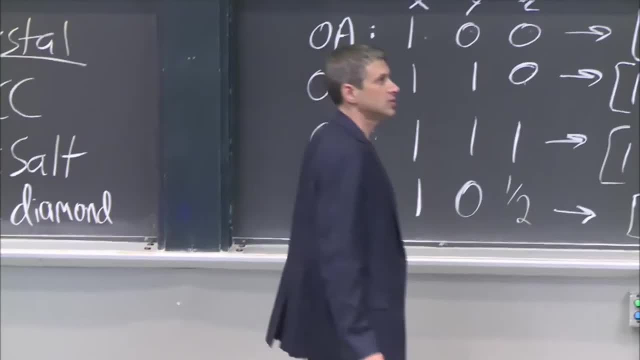 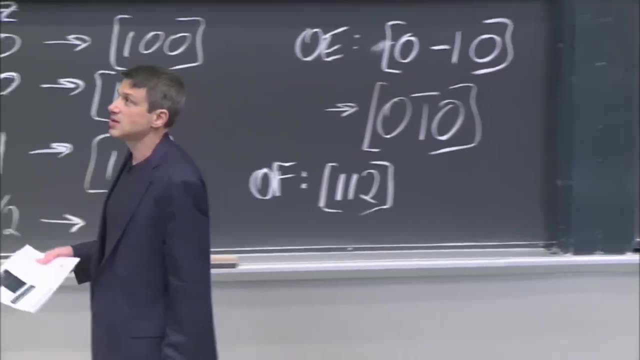 But they don't like the half, So you multiply through by 2, you get the 1, 1, 2.. These are vectors in crystals. Now, there are equivalences here, because this is a cubic lattice right. 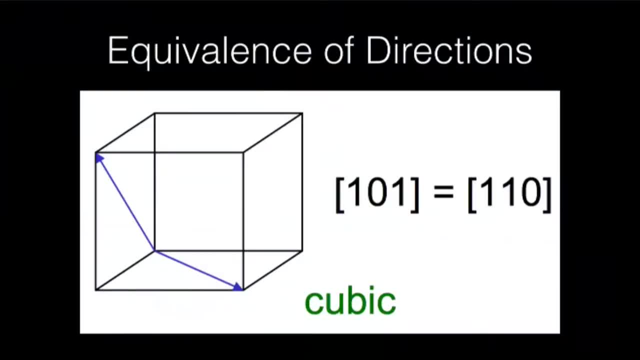 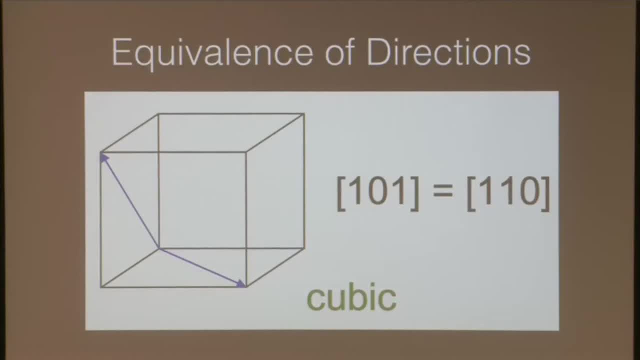 So if I look at this and I say, well, OK, if I went this way and I went that way, where I wind up are equivalent points. right, Where I wind up is you're winding up at the same place, in a way in the crystal. 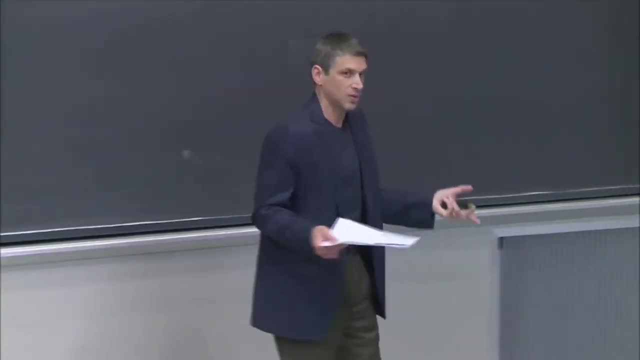 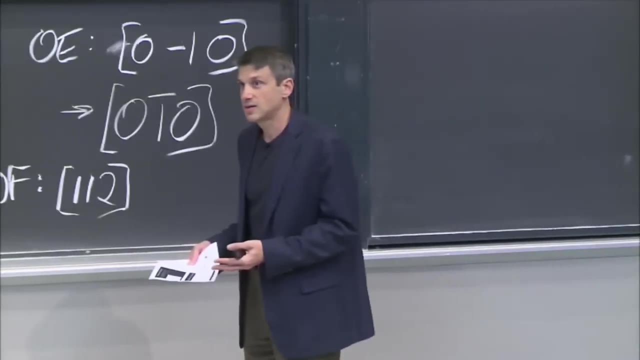 because the definition of that stamp in a cubic lattice is that those are all equivalent. Doesn't matter what's on your basis, right, Because it's defined by the Bravais lattice. That's the stamp. OK, So we have a way of writing that too, right? 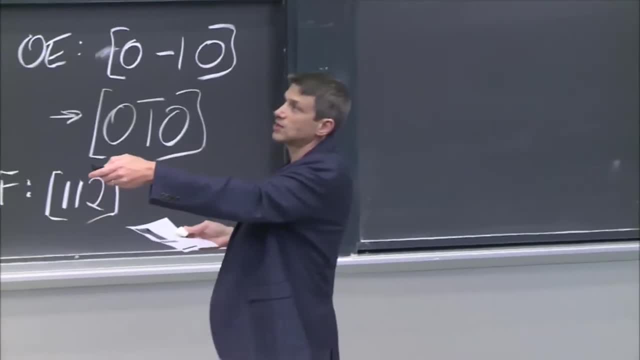 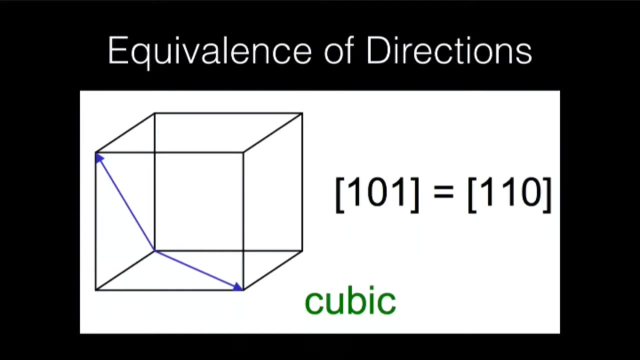 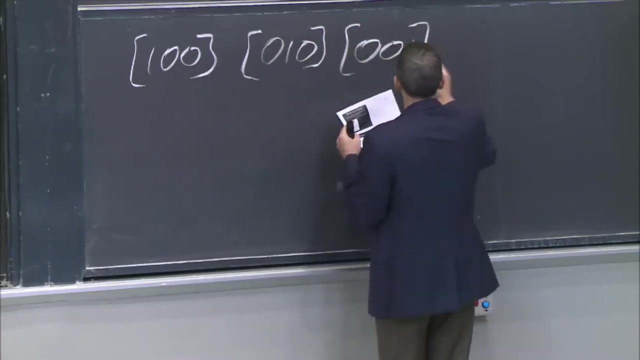 So if I were to take it so the 101, that's the 101 direction and the 110 direction. cool, If I make it a little simpler, I can say that the 100 and the 010 and the 001, oh, let's do them all. 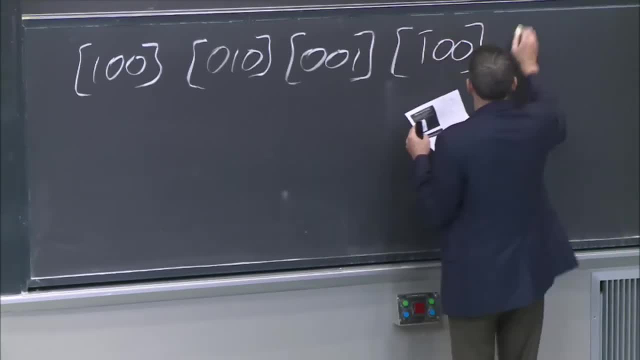 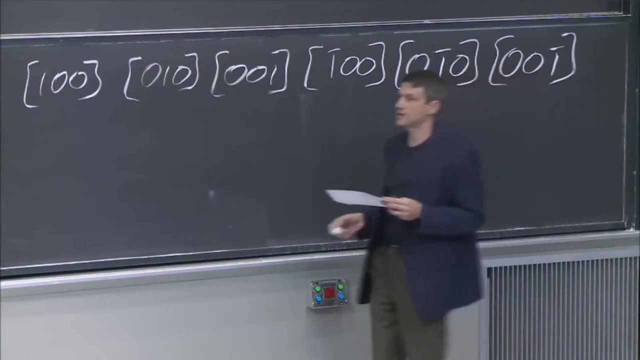 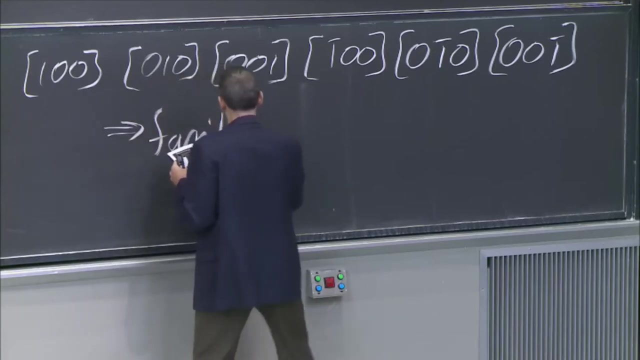 And the 1 bar 00, and the 01 bar oh, and the 001 bar all get me to equivalent places And we can call this a family, Just because we don't want to keep writing them. If they're all equivalent, we can say: 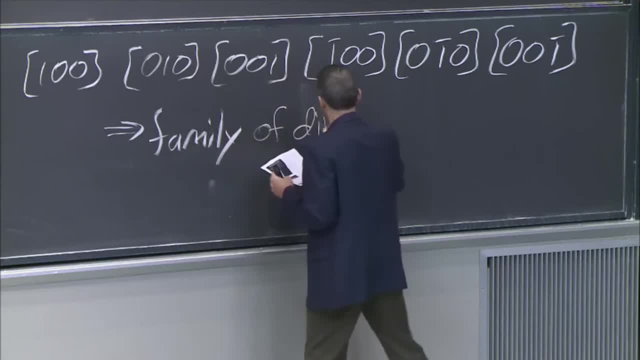 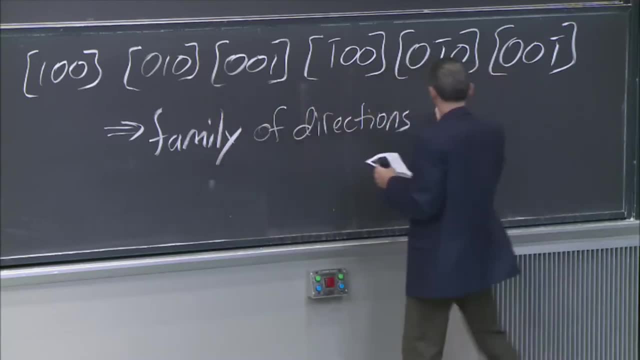 this is a family of directions And you've got to be careful here, because you can't use a bracket anymore, because it would just be one of the directions. Instead we use- sorry, you can't use a square bracket. Instead we use this kind of bracket. 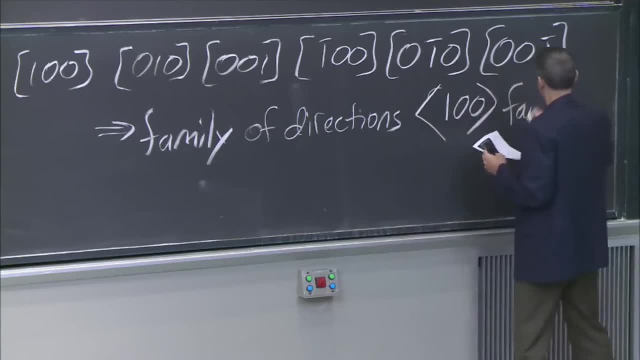 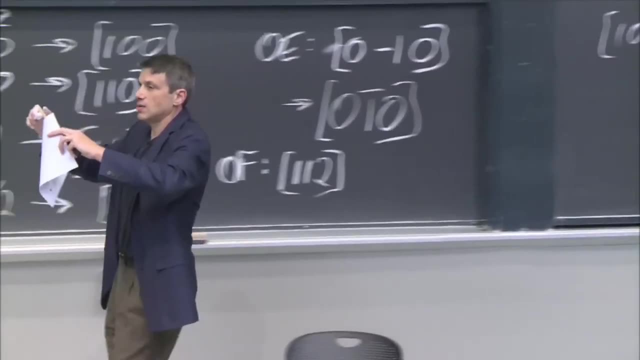 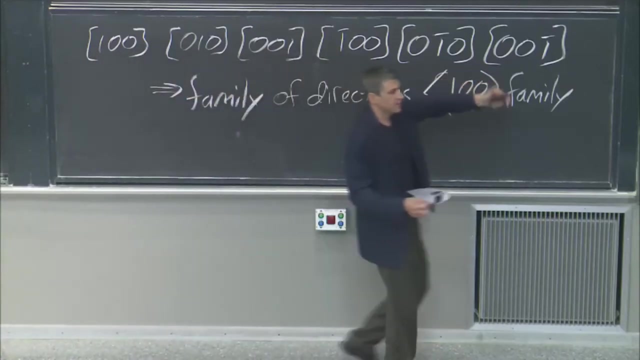 and we say it's the 100 family. So if you see a direction written with brackets like that, But then it means all of these directions, this family of directions, But if you see it written with a bracket like this, it means that one vector OK. 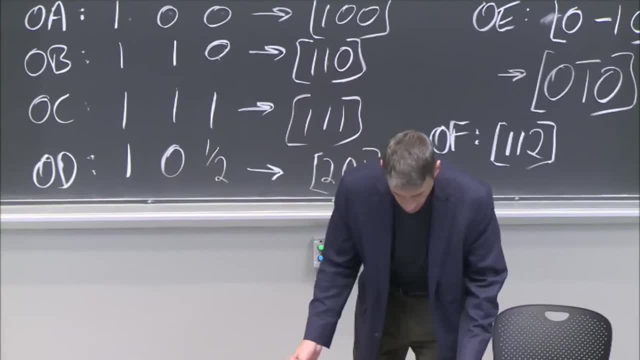 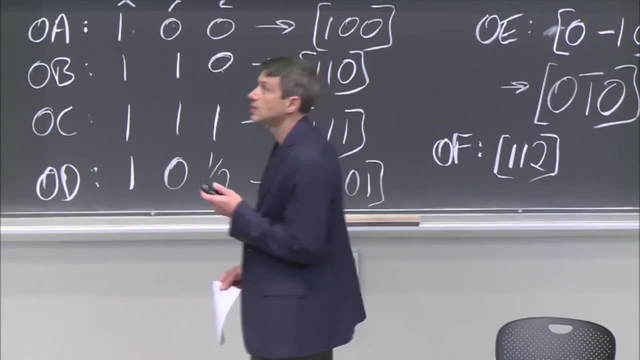 Crystallographers. you've got to keep them happy. You've got to keep them happy. All right now, that is directions, That is direction. But what about cuts? What about? What about planes? So we've got our vectors. 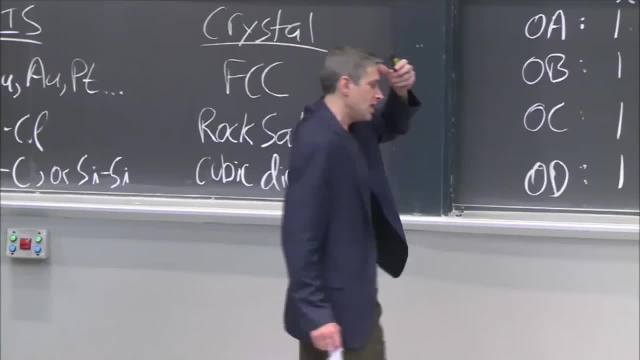 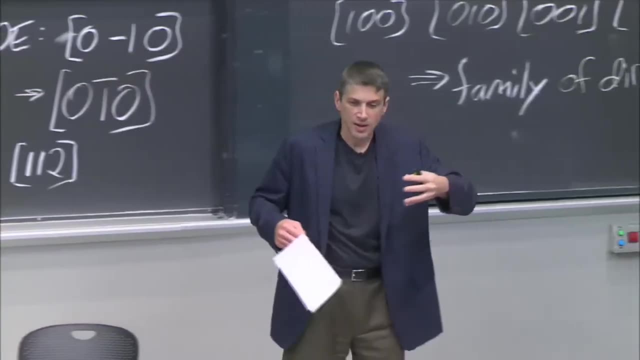 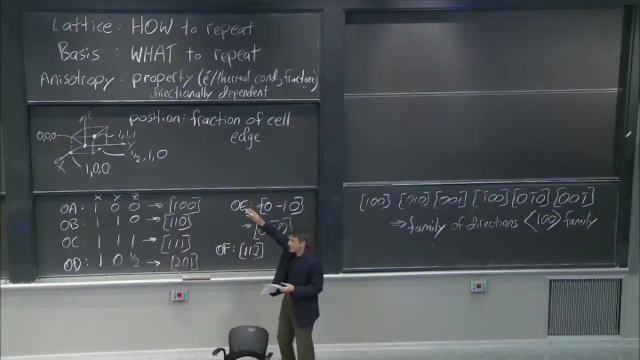 Now we need our cuts, We've got to be able to specify these things And, as we'll see, as we'll see, the properties of materials, of crystals, especially the more anisotropic they are, depend very heavily on what's in what direction. 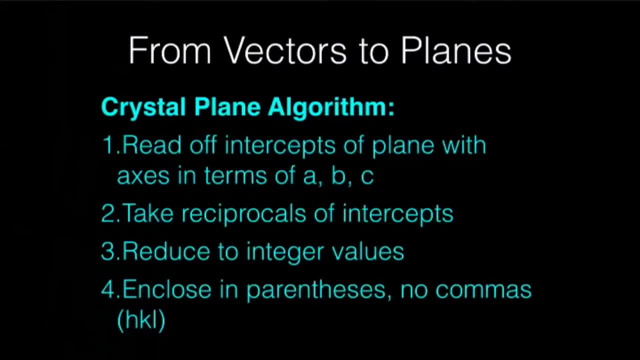 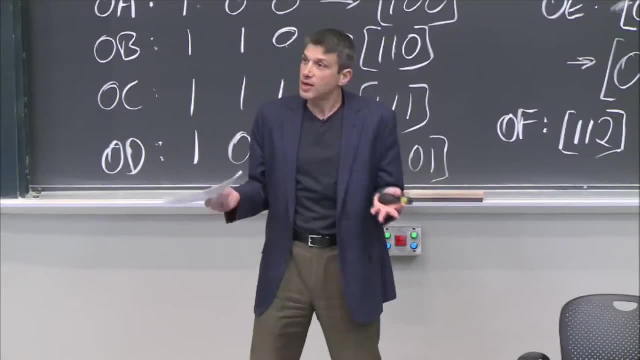 So, for example, if I have a plane in a crystal that doesn't have a high density of atoms and then I've got another plane that's got a lot of density of atoms in that plane, well you might expect those to have different responses to, for example, 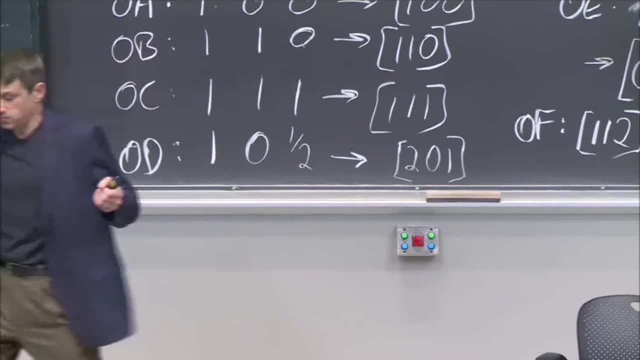 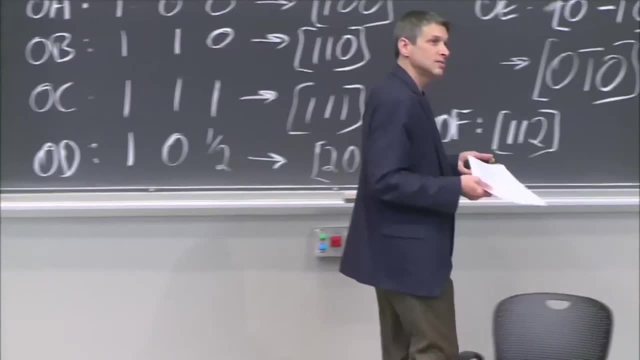 mechanical stress strain right. Let's say: you push it, you pull it, you break it, you hammer it. Maybe one of those planes, if it doesn't have as many bonds in it right, might break first. This is one example. 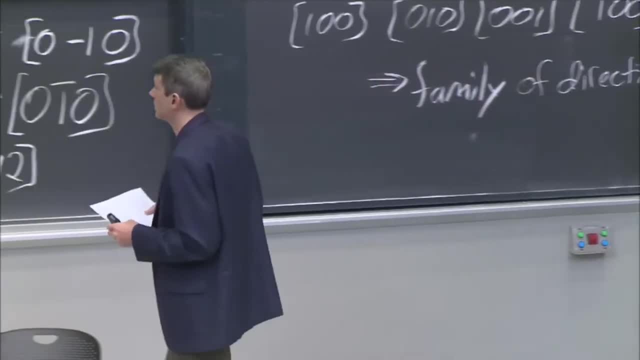 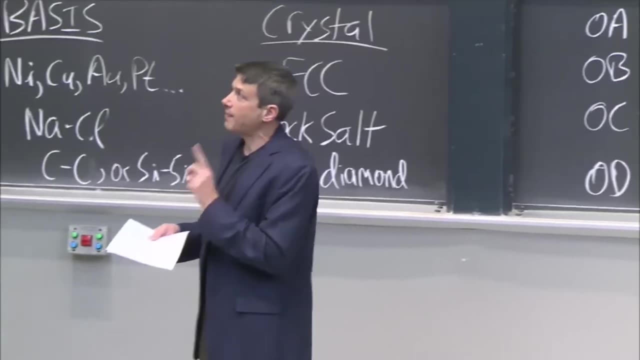 So we've got to know how to talk about these things. We've got to know how to talk about these things. OK, So now with planes. I have another recipe to make crystallographers happy. OK, Now, first read off intersec. 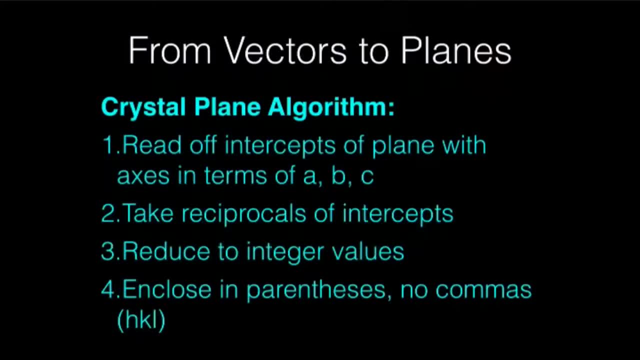 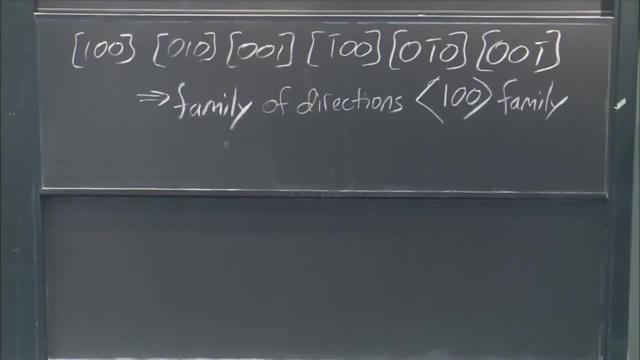 Oh well, let's put an example up. So I've got an example. I'll do a few, And then, as always, you guys need to do more to practice, right? So I'll do a few. So I'm going to draw a plane. 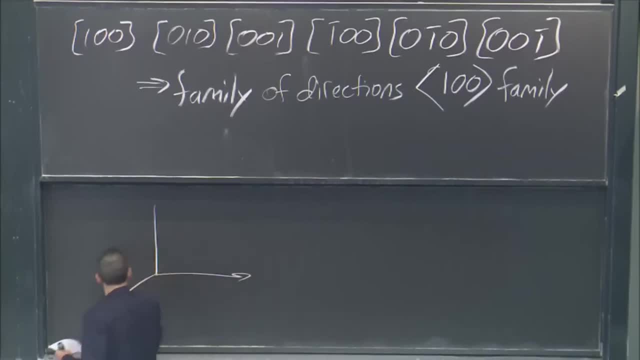 And I'm going to make it a nice simple one. These are my axes: x, y, z, And I'm going to draw. I'm going to draw my cubic crystal, my cubic unit cell, Sorry, OK, here we go. 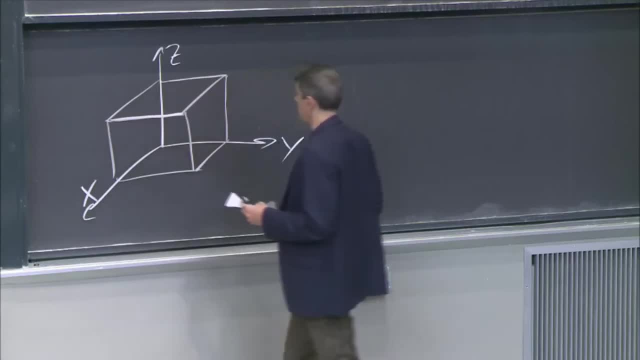 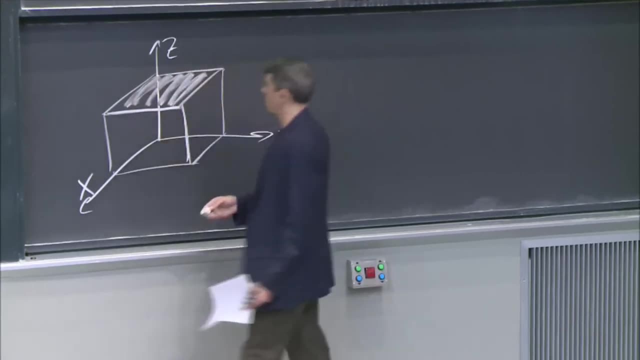 And almost a cube. OK, now I want to take a plane here. I'm going to take this top one, So I'm going to take this And I'm going to go through those. I want to know how do I describe? 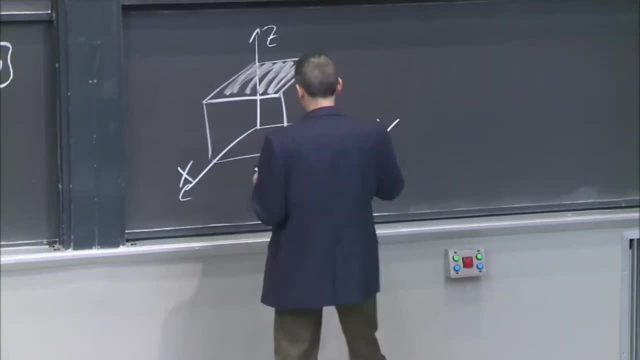 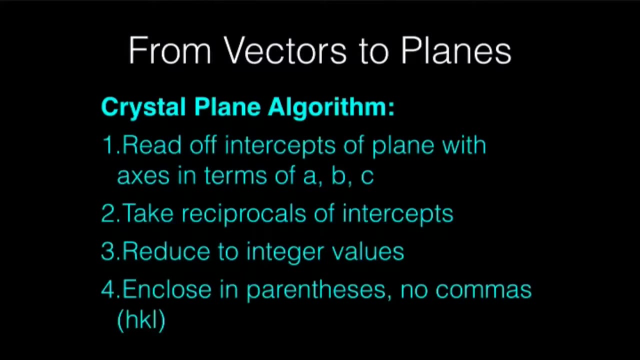 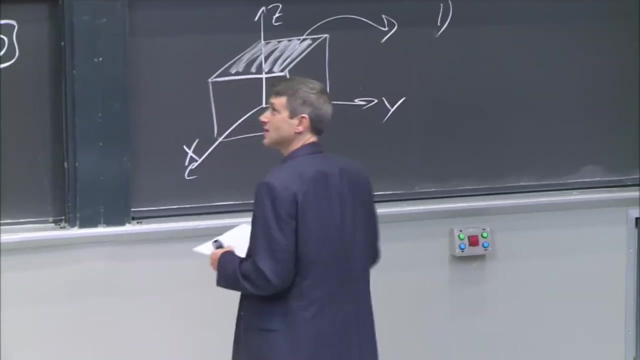 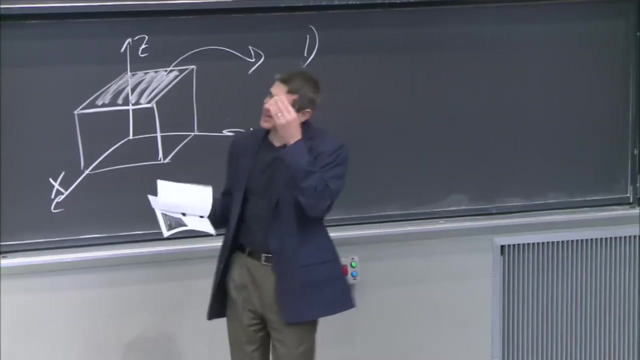 that plane. that cuts that way. OK, so one. these correspond to those Crystal plane algorithm, Algorithm. I hear a few of you like algorithms and computing. in course six, And so we got one whistle. So here's the thing. 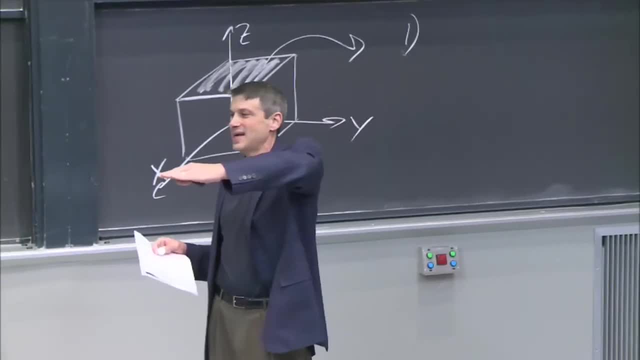 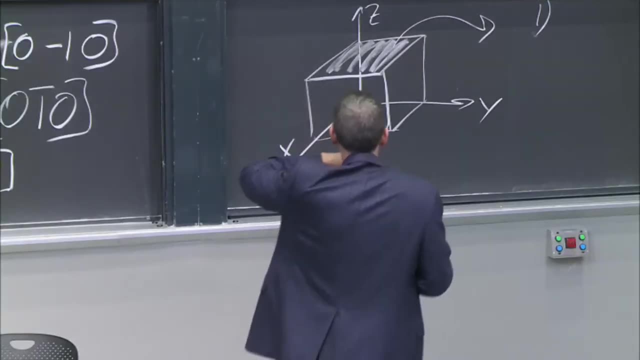 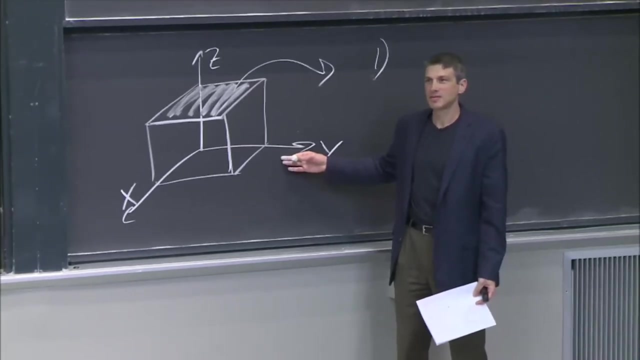 If I have a plane like this and I ask you, where does it intercept? Where does it intercept the axis right? Well, it's never going to intercept the x and y axes. Never. It's never going to intercept them, no matter what I do. 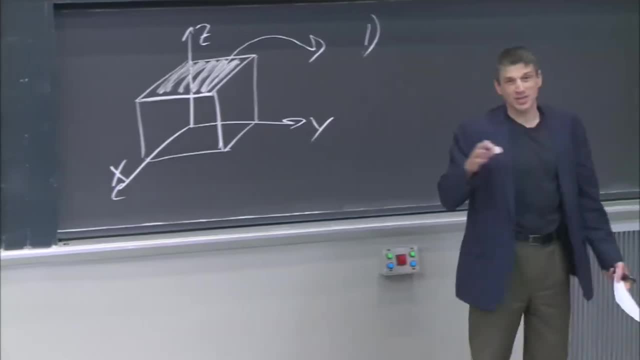 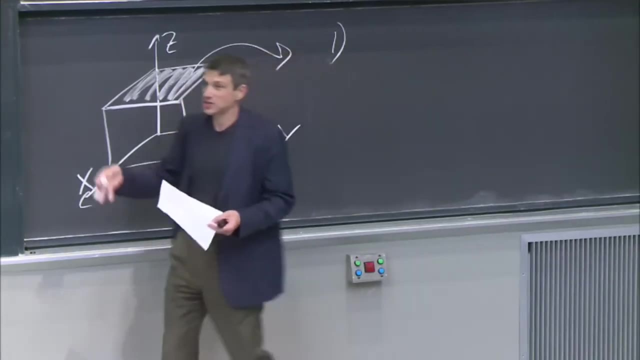 You say: but what if I put it in the xy plane? Then it's always intercepted. No, that's not what we mean by intercept. What I mean by intercept is it has to reach them eventually, no matter where it is. 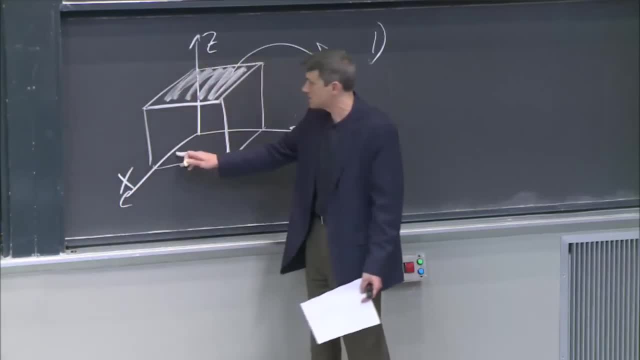 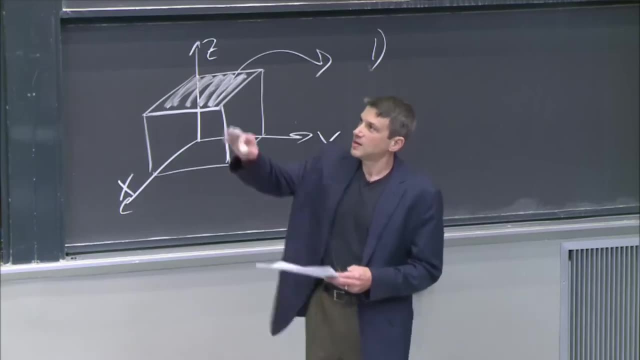 No matter where I position it, it's got to. But this never does, This never does right. And so the intercepts For the abc intercepts, so we can write those here. OK, I'll write the same way. 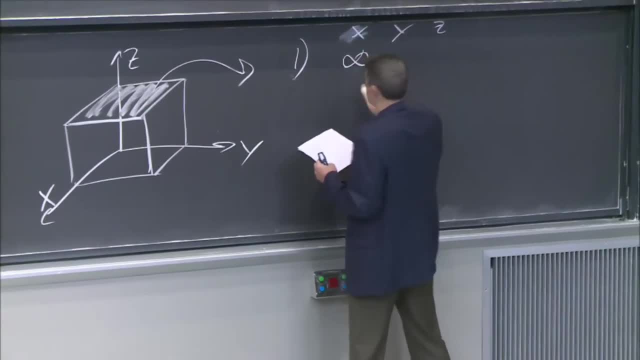 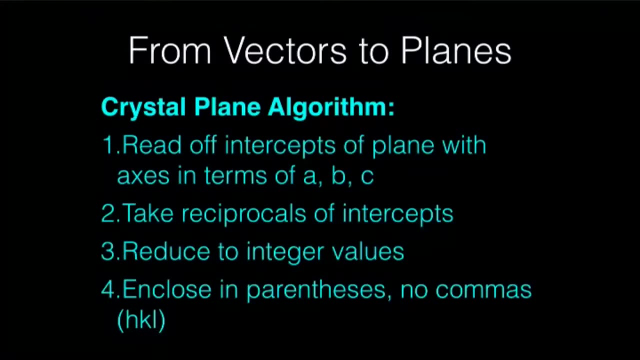 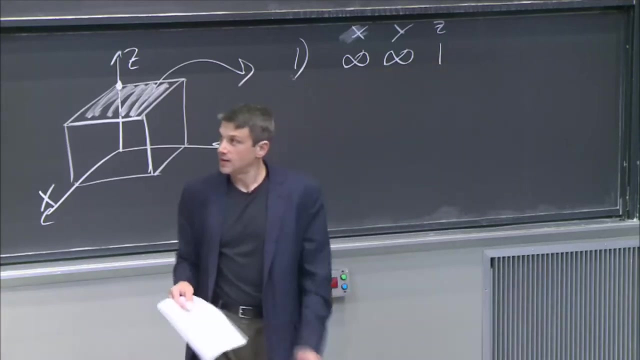 x, y, z intercepts: It's infinite, And it's infinite, right. And then for the z. OK, here I'm intercepting at this part of z, So I'm intercepting at 1.. But the thing is, oh man. 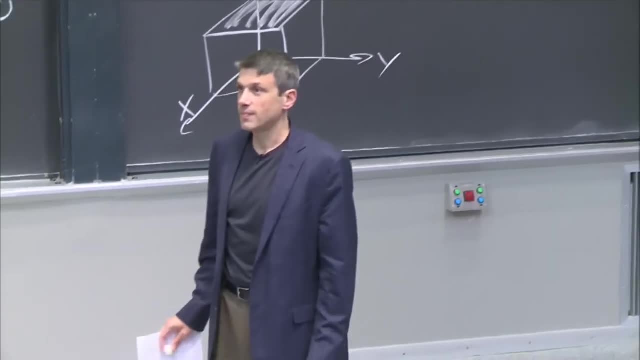 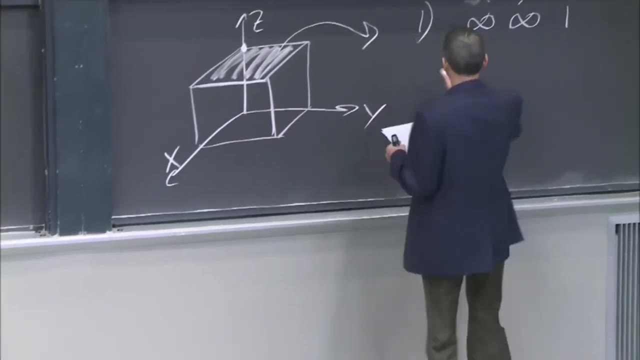 Crystallographers don't like infinity either. They don't, And so what they do is they just take 1 over. That's a nice way to fix infinity. And so step 2, this would become 0, 0.. 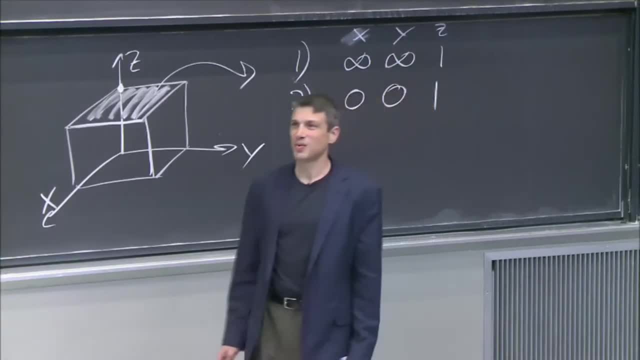 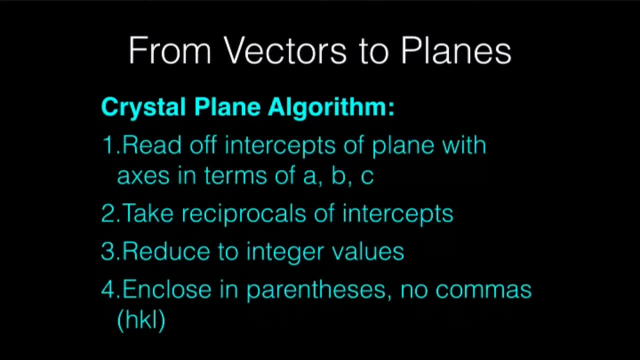 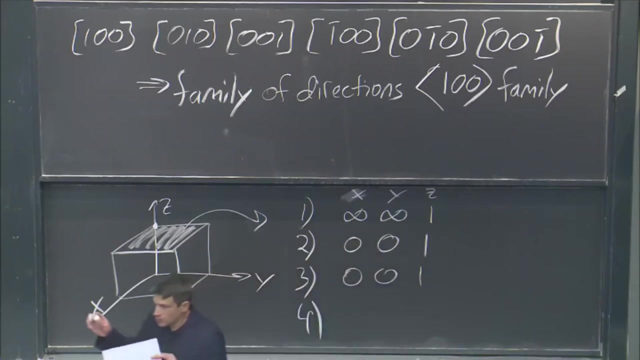 And 1 over 1 is 1, right, 1 over infinity is 0. Now we reduce to integer values And that there's no work to do there, And then- we are very careful about this- We use parentheses. 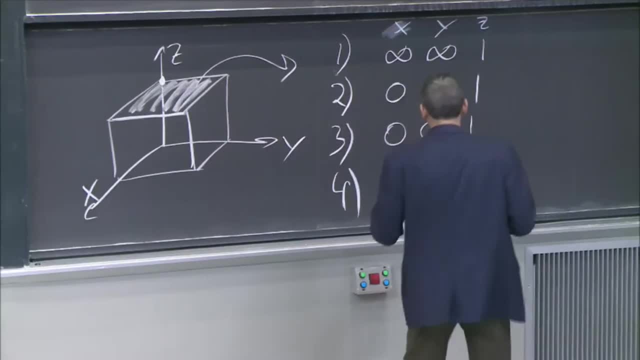 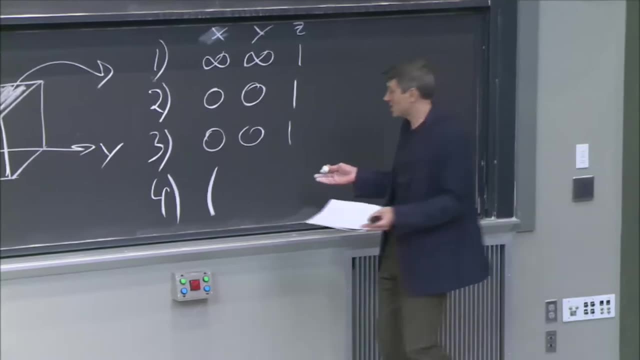 No more brackets. Parentheses, Do not get this wrong, Because you might be talking about a vector by accident. You don't want to talk about a vector by accident. So this is the 0,, 0, 1 plane, No commas. 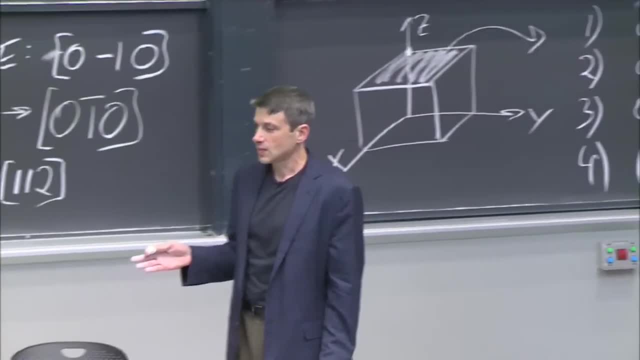 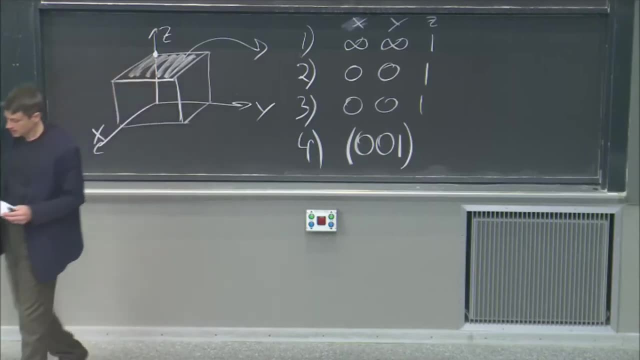 Remember the dislike of commas. It's the 0,, 0, 1 plane in this crystal. That is a cut, OK, good, And that's called a Miller plane. Well, if I do another example, do one more. 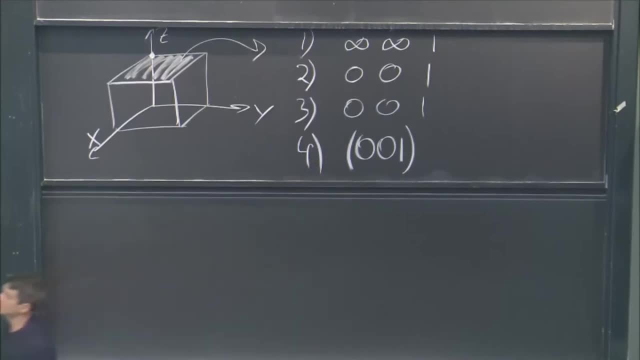 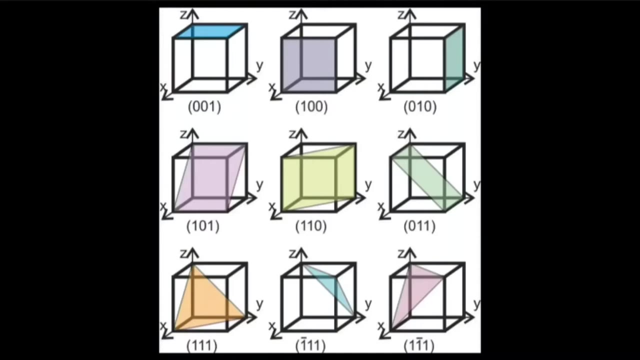 So that is this one. I have it. I've got a bunch of examples here And they can draw it better with the shading and stuff there. But you see, that's what we just did. We did the 0, 0, 1 plane. 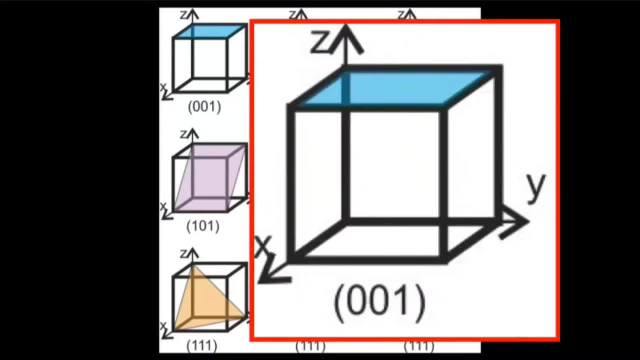 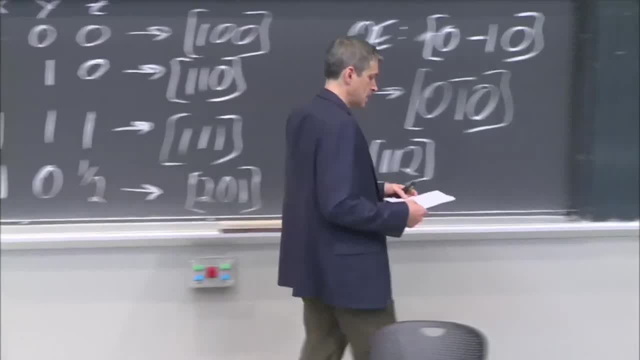 That one there, right There, it is Nice and big. The 0, 0, 1 plane. What about that one? That's the 1, 1, 0. The 1, 1, 0, if you do, the 1, 1, 0, 1, 1, 0, I'm not. 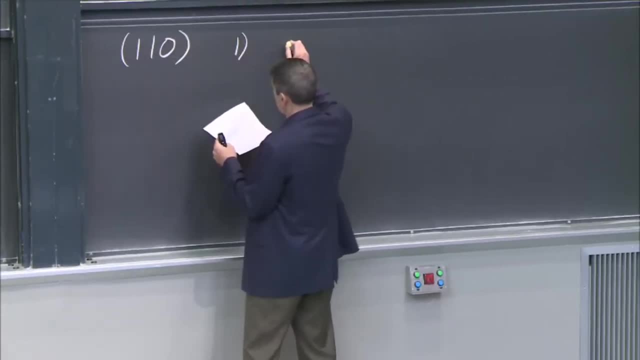 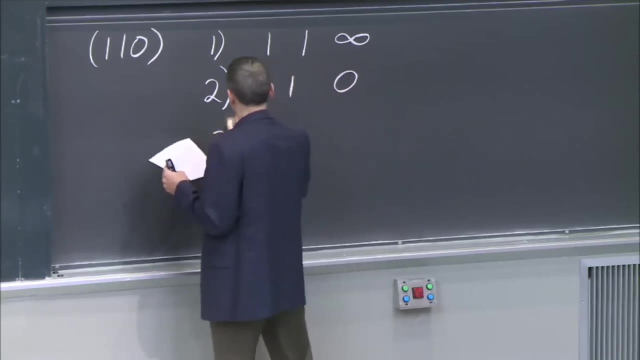 going to try to draw it again. What you get is: step 1, you get 1, 1, infinity. Step 2, you get 1, 1, 0.. Step 3, you get 1, 1, 0.. 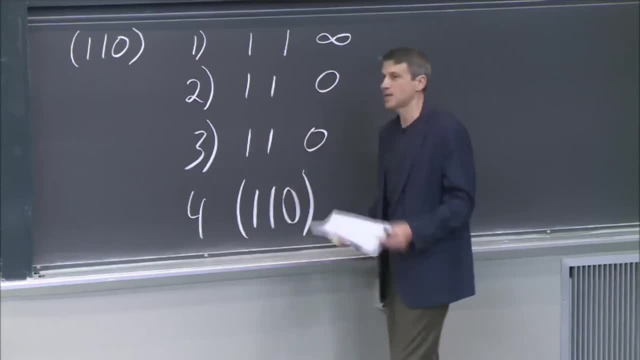 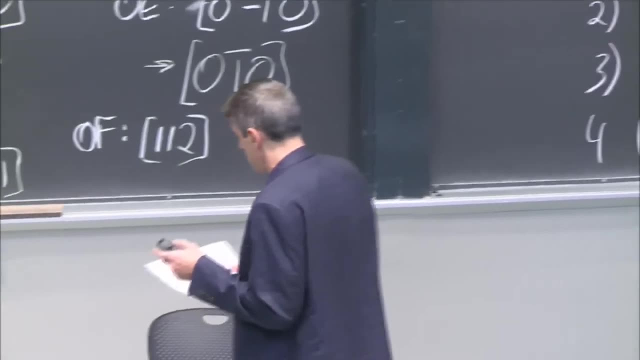 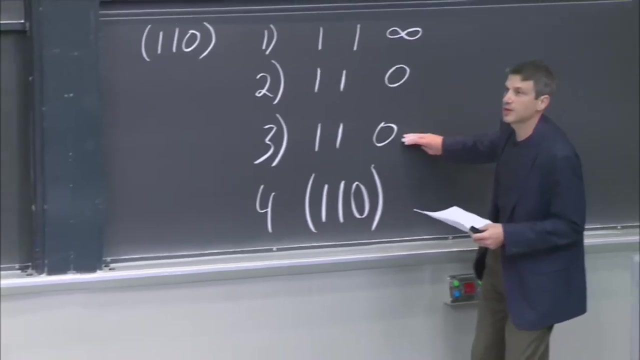 And step 4, you get 1,, 1, 0. Those are the steps to identifying and labeling a crystal plane. Let's make it a little more complicated. We still haven't really done something where we take advantage of the rule of step 3.. 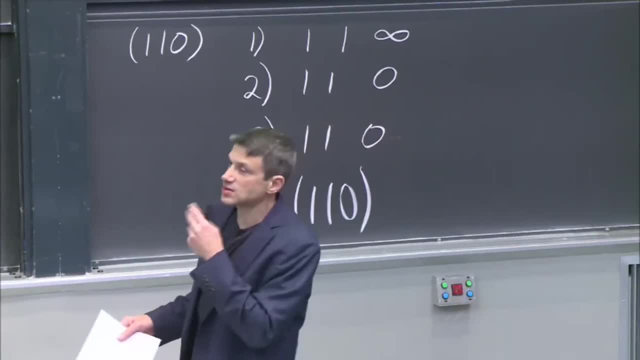 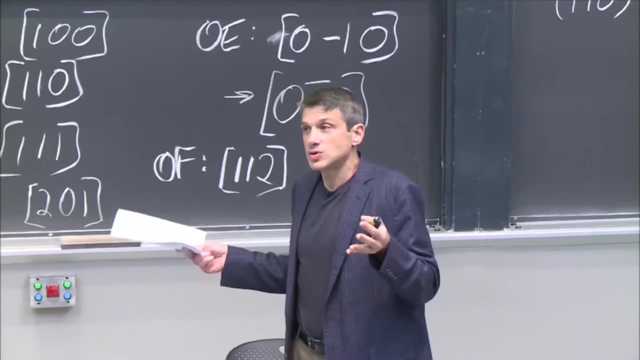 So let's make it harder, Let's bump it up. So there's a slice. Remember, I can slice a crystal in any way I want, And I've got to be able to write it down, I've got to be able to represent it on paper. 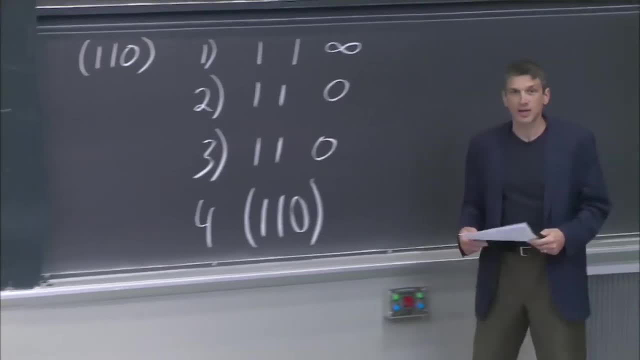 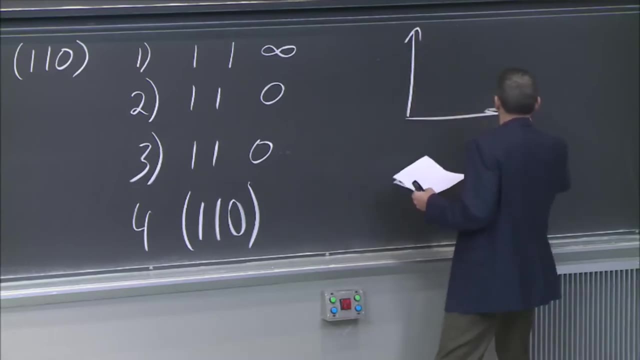 That's what this is about, That's what the Miller indices and the Miller planes let us do. So this one I'm going to try to draw. So here I've got my axes, And that's y, And that's x. 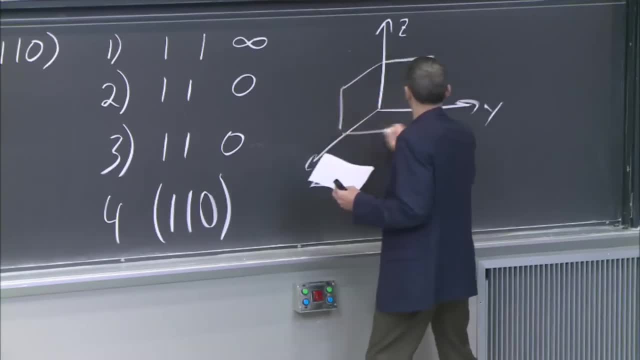 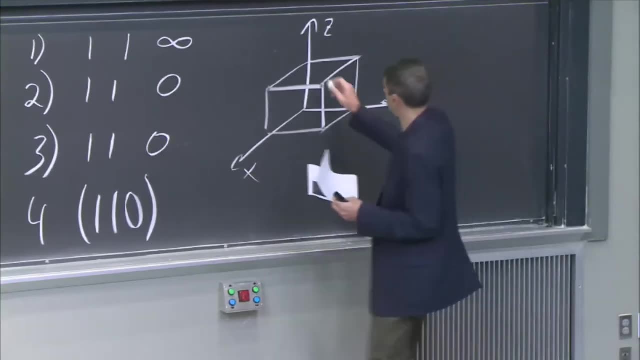 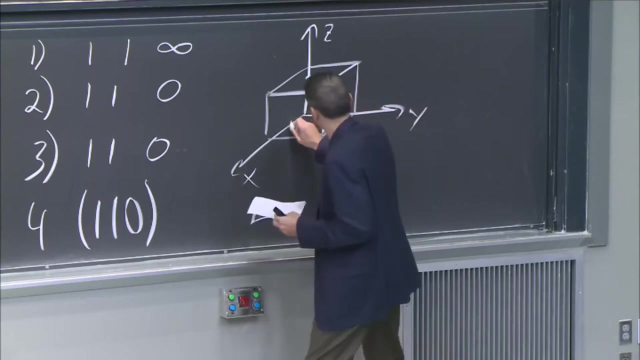 And that's z. Here we go. OK, Oh, that's almost a cube Now. I've gone up here to 3 quarters high. So I've gone up about 3 quarters there. I've gone here to 1 half. 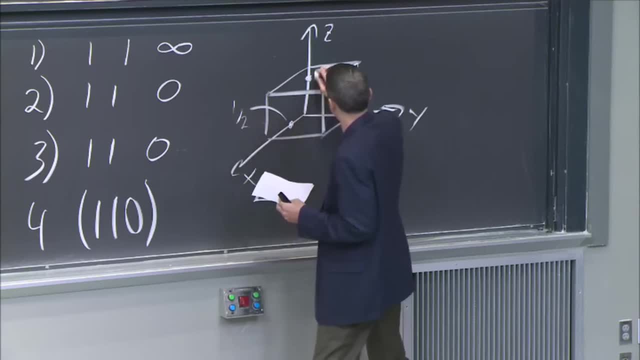 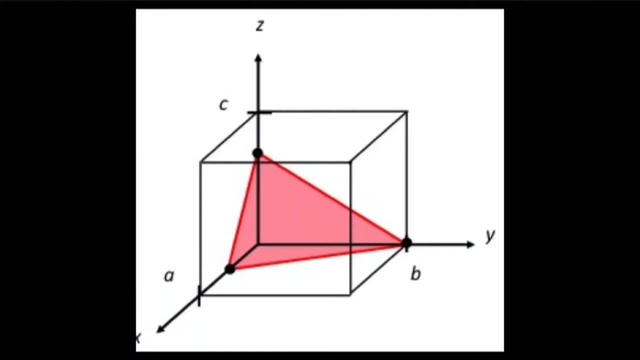 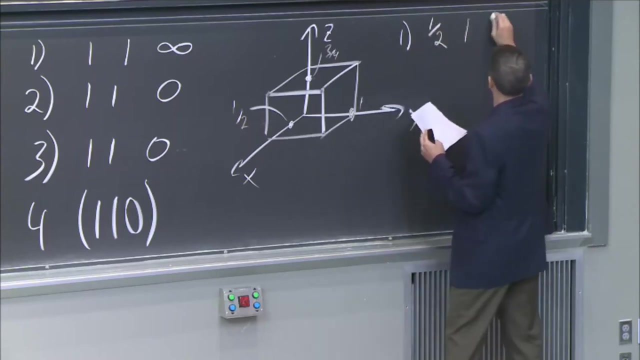 That's 1 half of the cell length. This is 3 quarters of the cell length And then over. I've gone all the way to 1.. So now, if I go through my steps on this one, I've got 1 half, and I've got 1, and I've got 3 quarters. 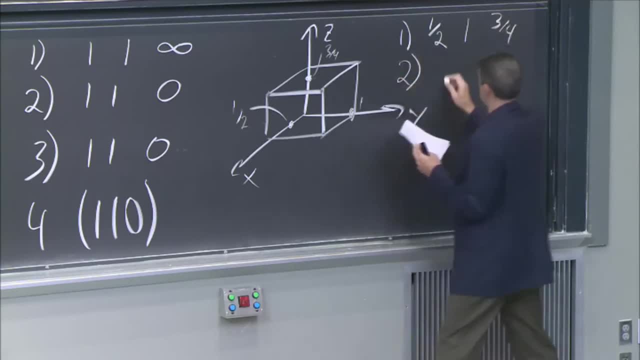 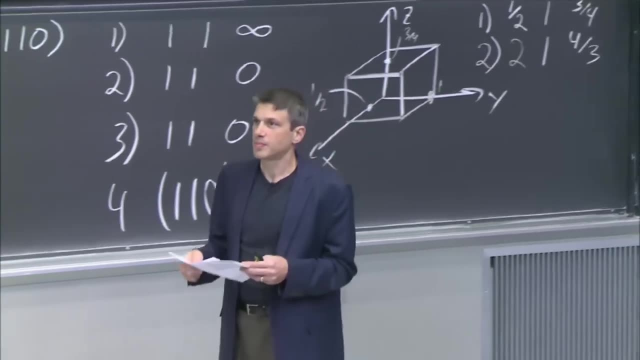 OK, I'm going to take the reciprocals. OK, That becomes 2,, 1,, 4 thirds. Oh, not happy yet. Not happy yet. We don't like fractions. We've got to get rid of fractions. 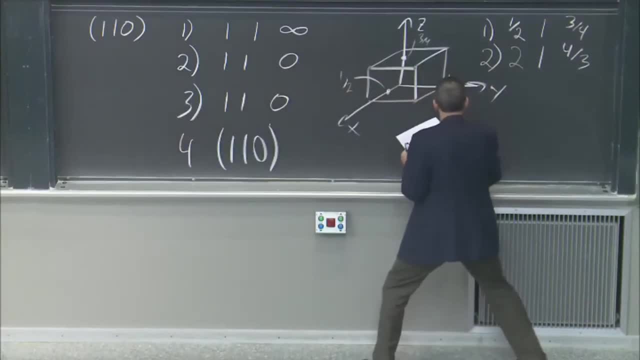 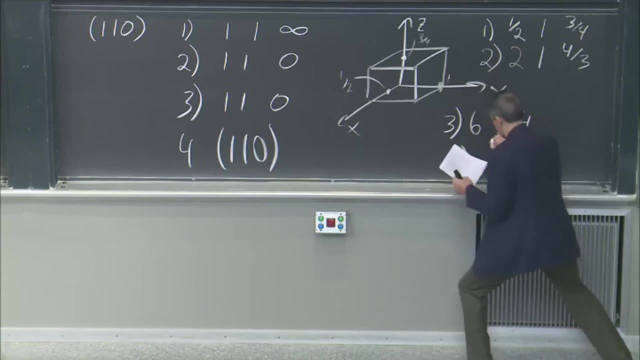 So in step 3, we simply multiply through by 3. And we get 6,, 3,, 4. And then we can write down That plane, That is this 6, 3, 4 plane. OK. 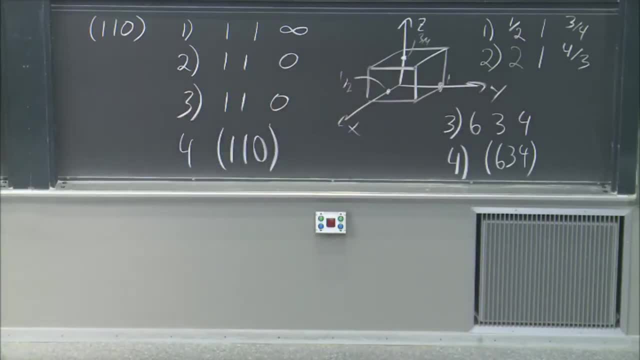 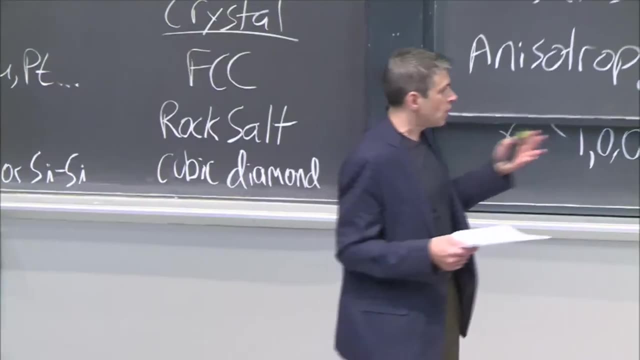 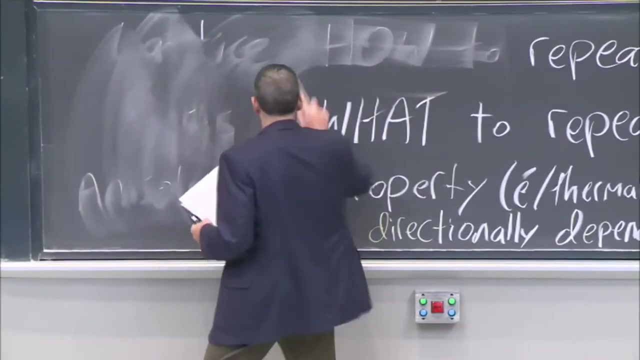 And so on and so on. Now let's go back to let me erase this. There's a couple of things about the planes that once we know what the plane is, we know some other things about it. OK, So let's talk about that now. 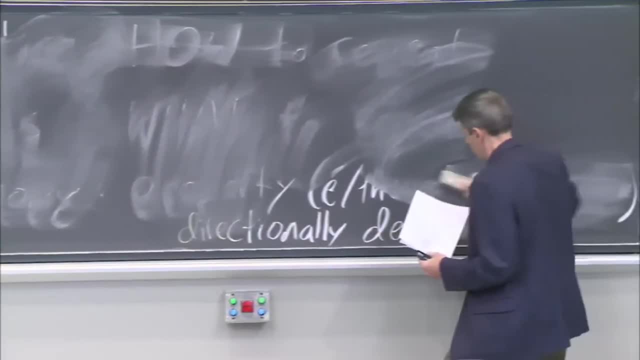 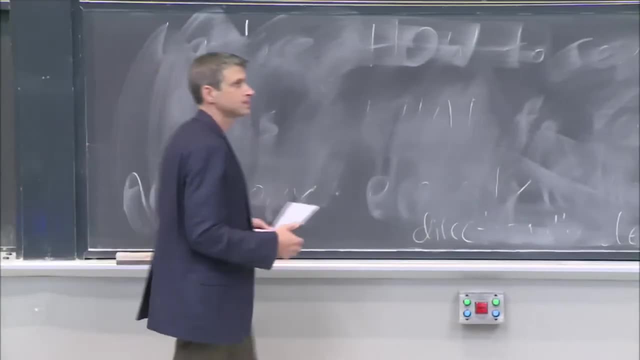 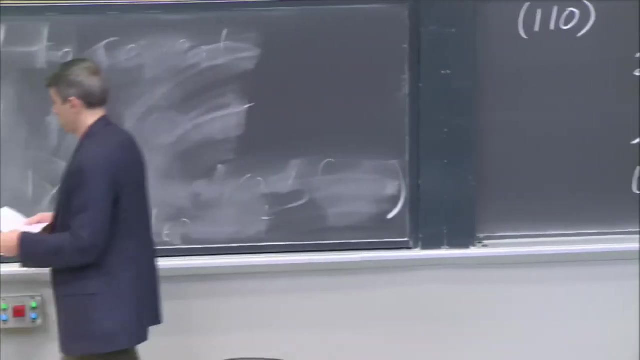 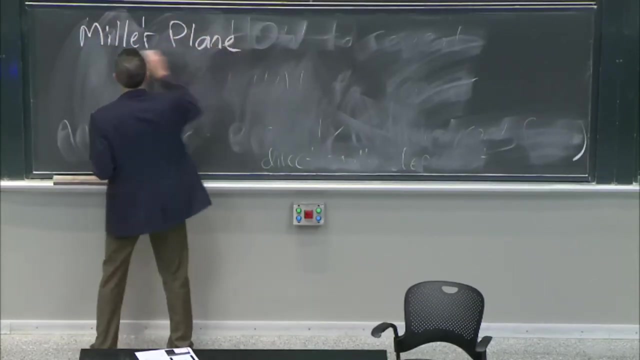 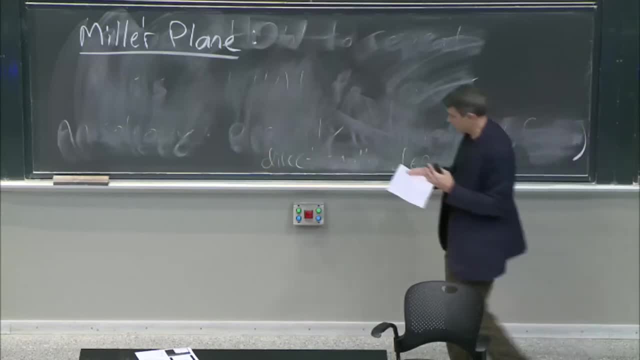 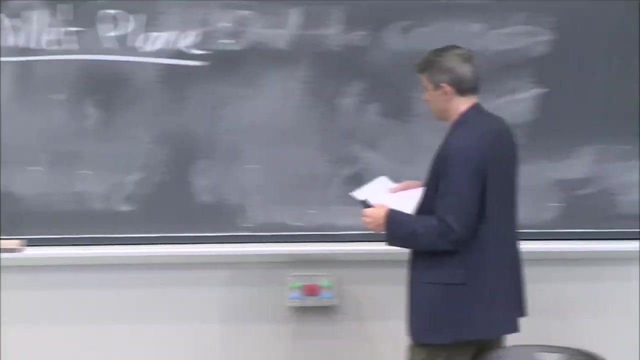 is what we've been doing, All right, Which is you define The plane that's kind of closest somehow to the origin Right In the unit cell, The one that cuts it. You define it that way. But actually what? Miller planes are infinite sets of planes. 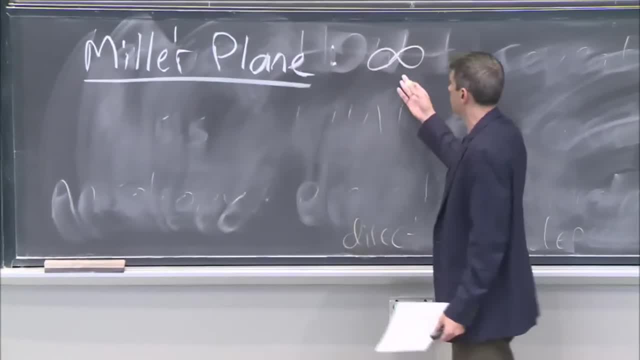 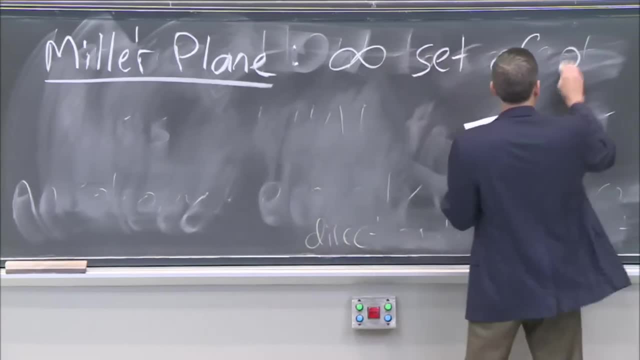 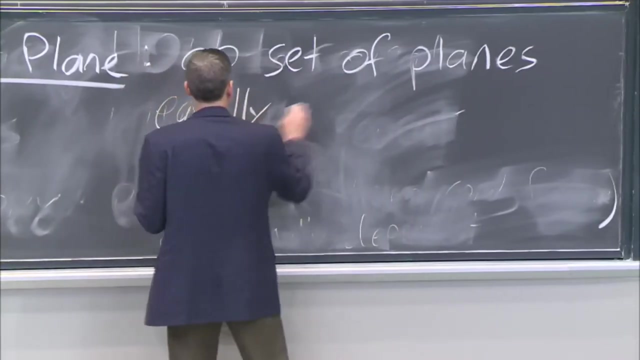 And so I'm going to put: Now I'm not a crystallographer So I can write infinity, I'm OK with that. It's an infinite set of planes, OK, They are equally spaced, Equally spaced. And here's the key. 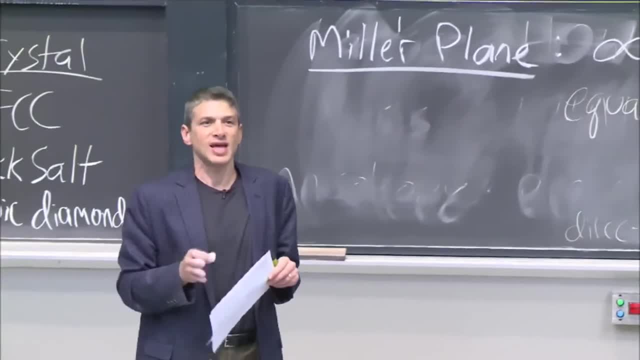 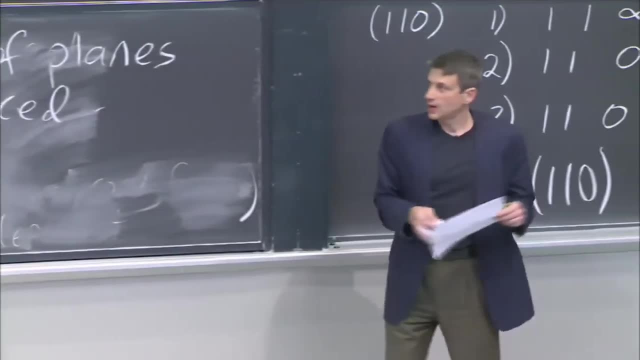 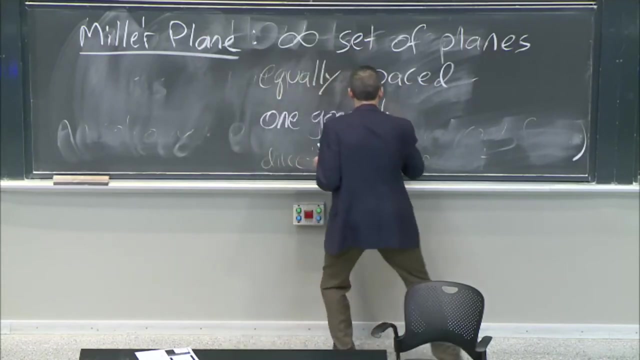 One should always be going through the origin. If you want to look at it as a set of planes, you got to put one at the origin. That will help you think through what I mean. OK, So if one goes through the origin, then what you see, right? 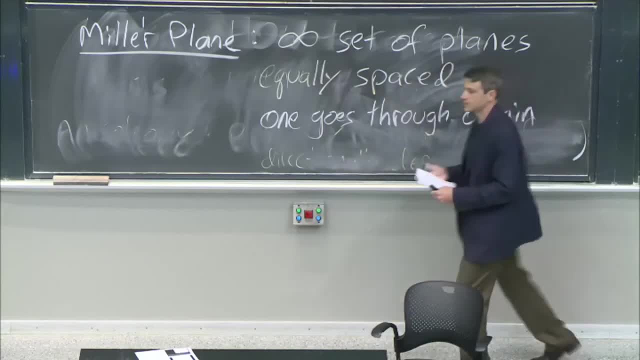 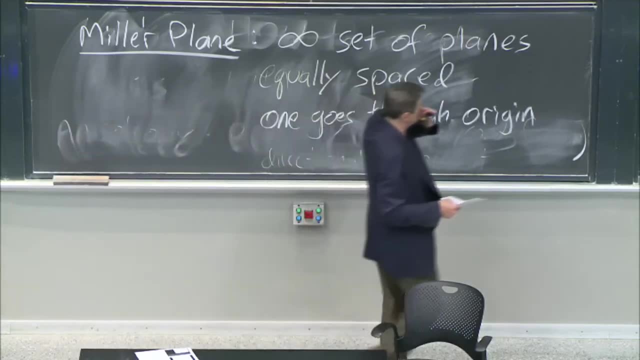 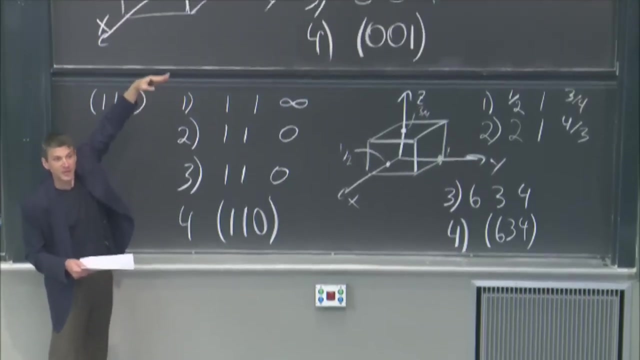 away Is how they repeat, Because it's not just that I go. in that case, Let's take that one. OK, The 001.. Now you say, where's the next one in this infinite set of planes? OK, Well, put that one at the origin and make another one. 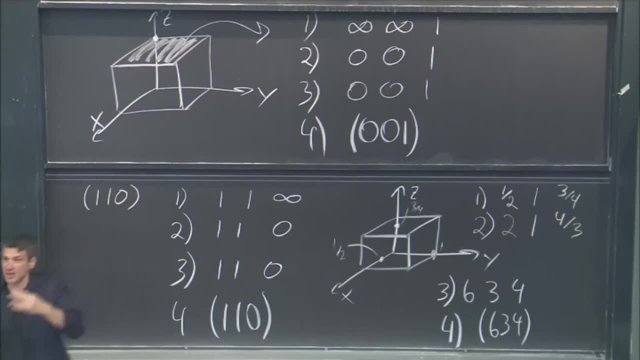 Then put that one at the origin again and make another one. That's how to think about this infinite set of planes. OK, But if I had one that went halfway, a 200 plane, or an 002 plane, as it would be, if it's properly noted, with Miller indices. 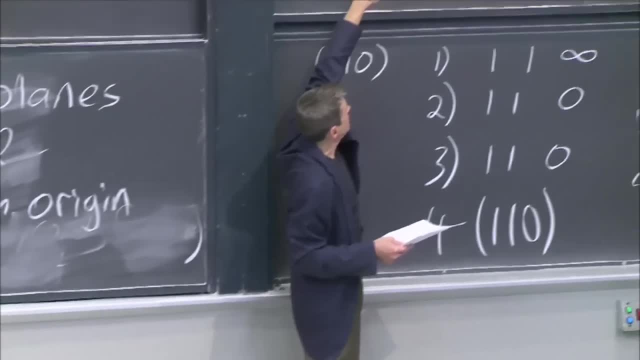 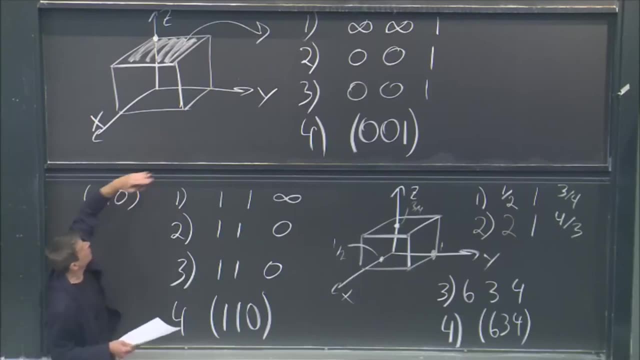 Well then you say, well, OK, I've got one halfway, Isn't that it? No, The set of infinite planes also would have one at the origin, one halfway, one at the top, Because each time you put it back and you do your next one. 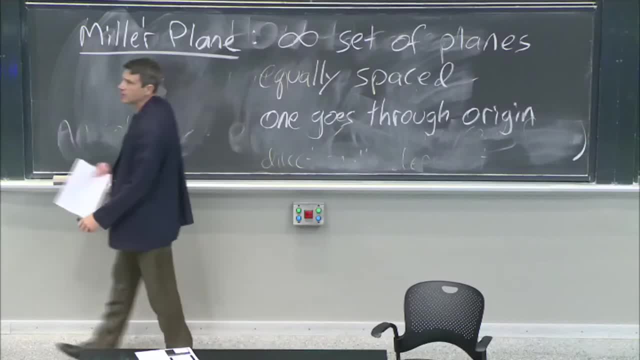 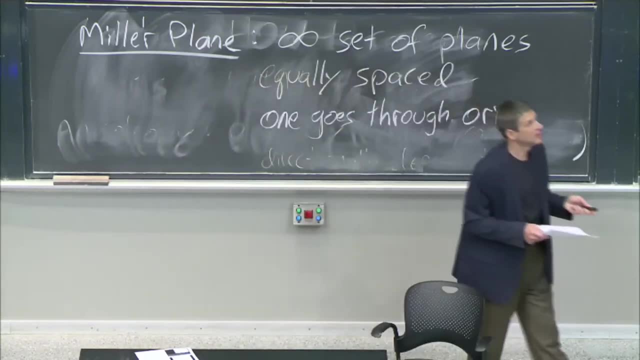 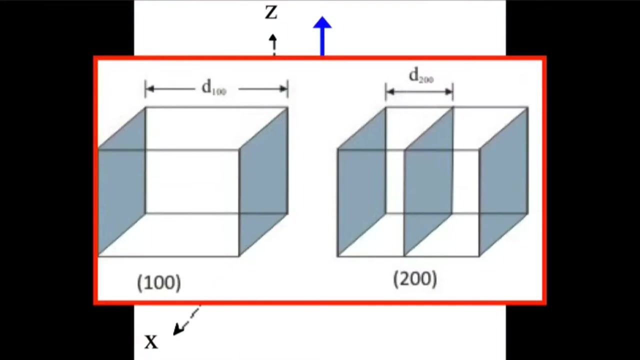 That's how to think about this infinite set of Miller planes. So you get this infinite set of planes that have- I'm going to go to this picture. OK, There it is A 100- that just go on forever. Those are the Miller planes. 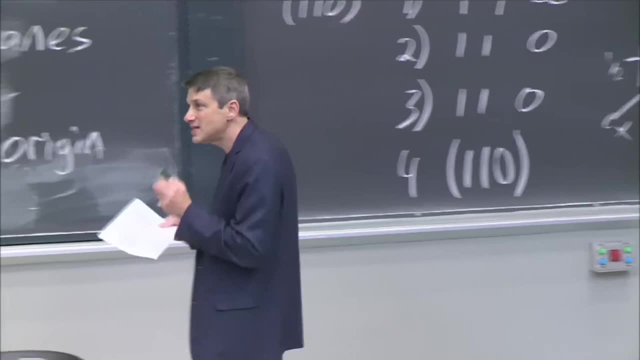 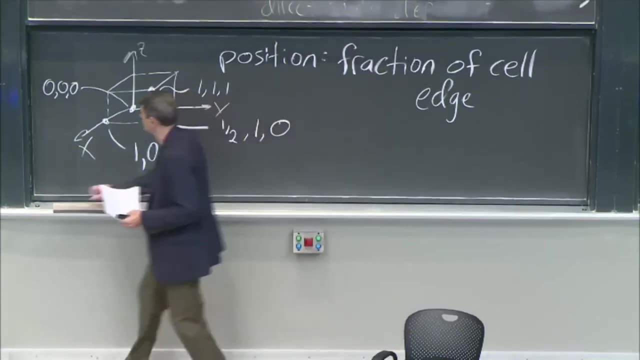 And what they have is a spacing between them, And this is really important. So this is the next thing I want to tell you. So a Miller plane isn't just one, It's infinite, It's an infinite number of them, And 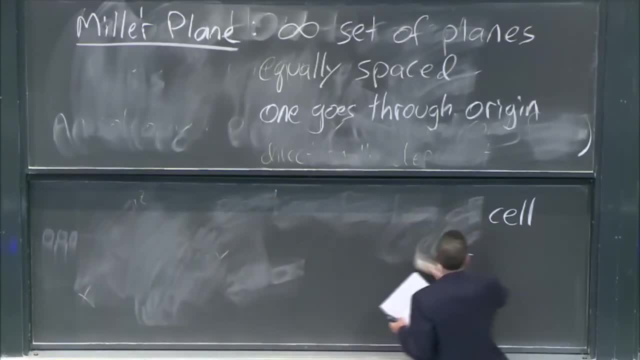 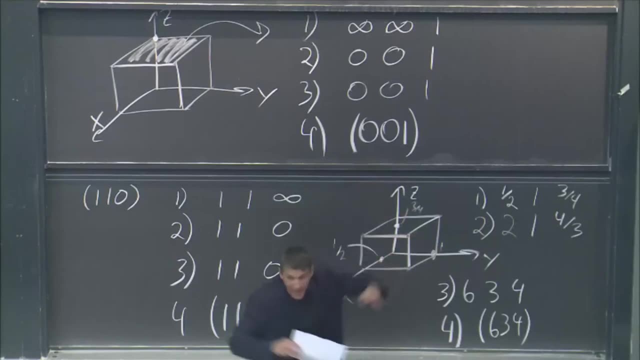 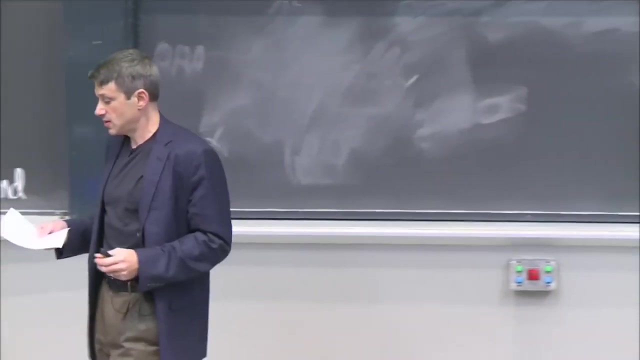 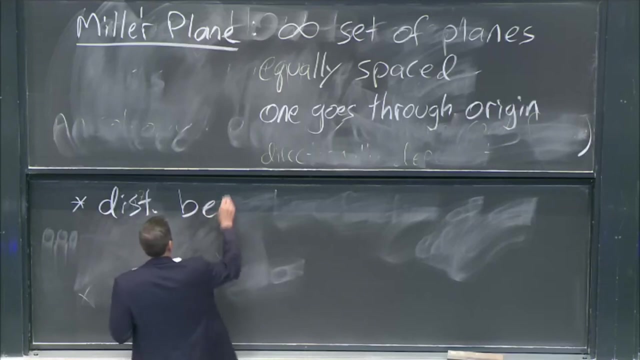 What that means is that when I give you this or that or any Miller plane, I know what the spacing is between them. That is enough information, Because the distance between planes Right Is Actually here. it's very easy to see. 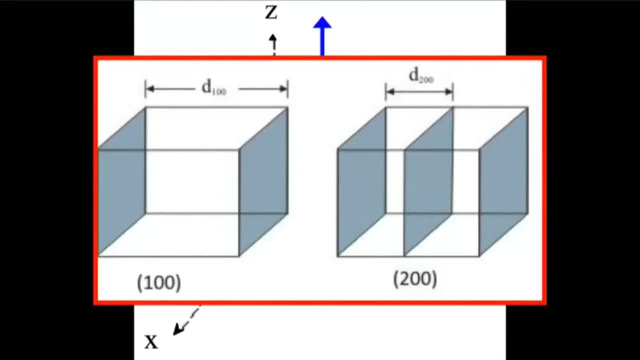 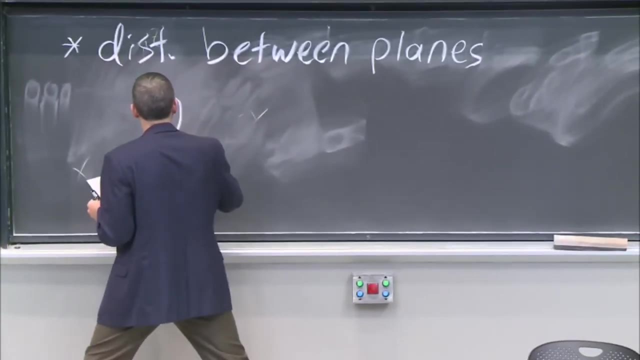 The distance between these planes is a, But the distance between the two 00 planes is a over two, And in fact for a cubic cell there's a formula that you can use for any two planes, The distance between. Well, let's say, I'll write the notation first. 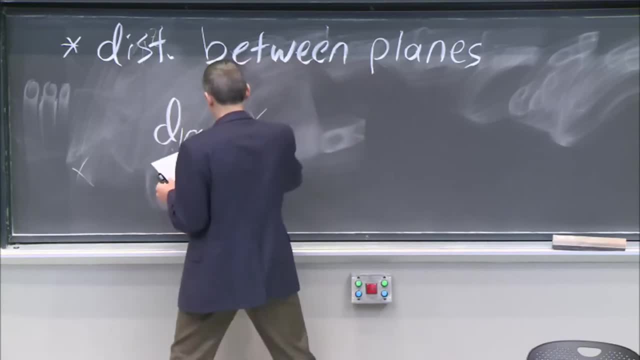 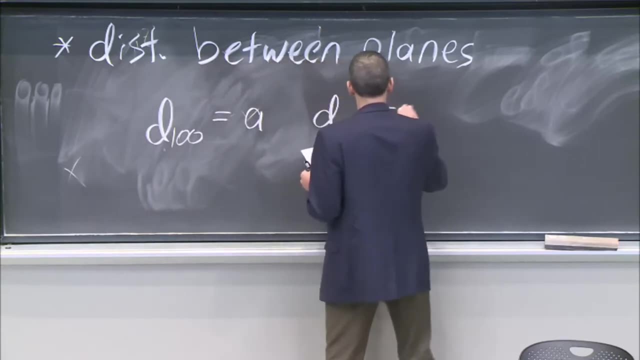 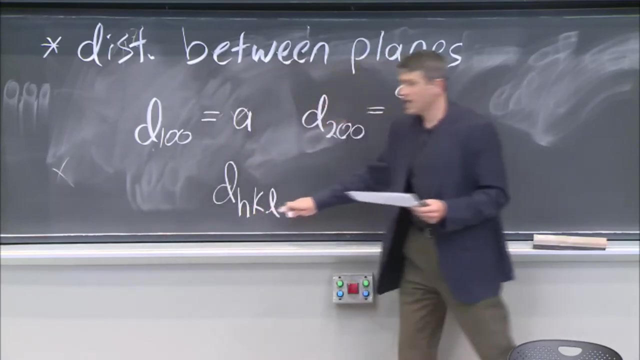 You put the distance and the plane there Is equal to a and the distance of a two, 00 plane between planes is equal to a over two. But there's a general formula of any hkl, hkl, the Miller indices, Those are just variables. 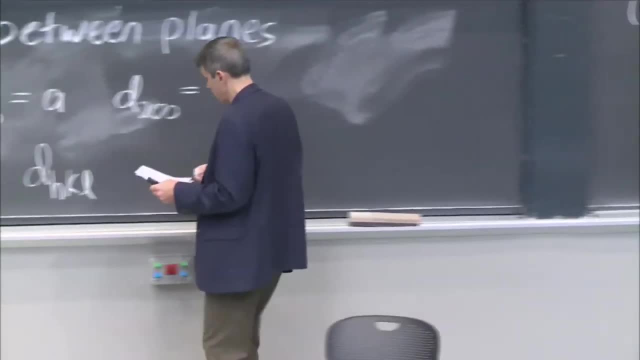 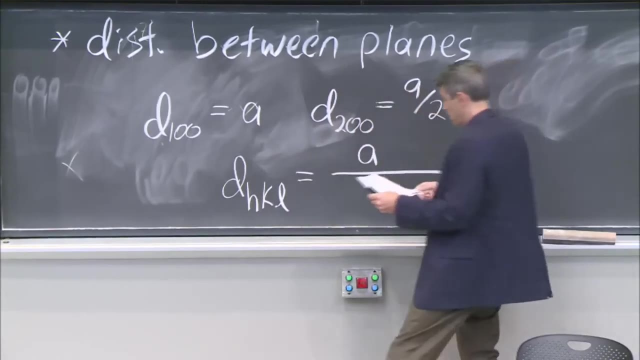 But if those are the variables of the Miller plane, then the distance between two of them is The length of the edge of the unit cell a, Divided by the Square root of the squares added together: H squared plus k squared Plus l squared. 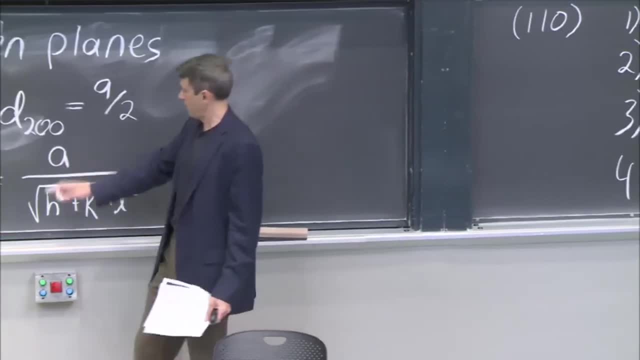 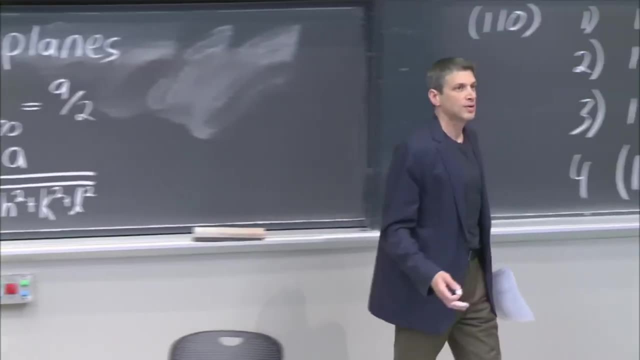 OK, H squared plus k squared. So you see, OK, If it's one, 00, that's a, That works. If it's two, 00, a over two, that works, And it's general. So now, just by knowing, because I figured out, 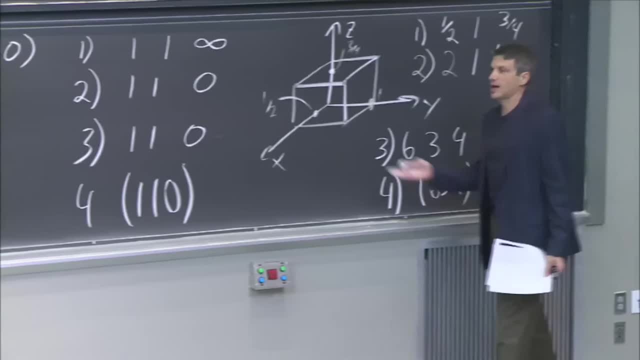 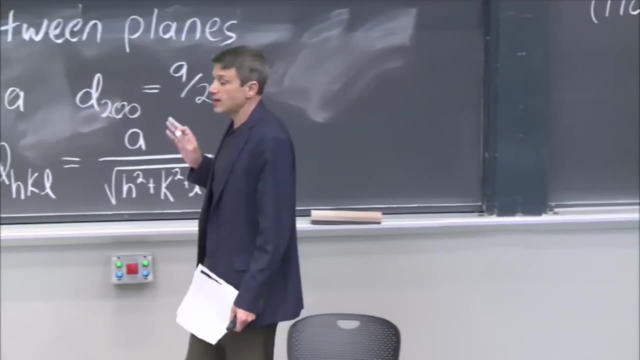 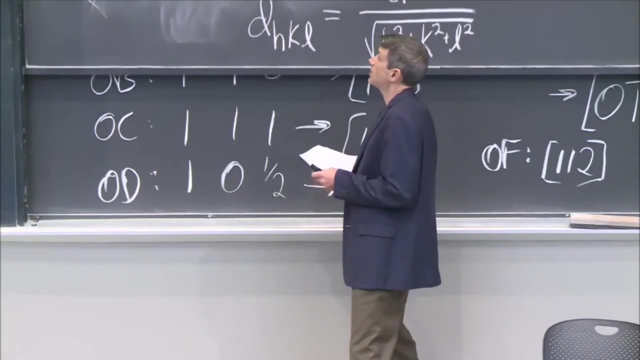 how to write a plane in hkl notation. I also know the distance between these infinite planes. That becomes very, very important once we shine x-rays on crystals next week. That becomes very important, OK, OK. So what else can we know from the Miller planes? 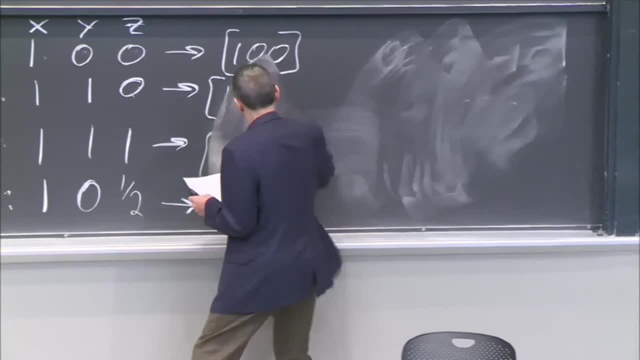 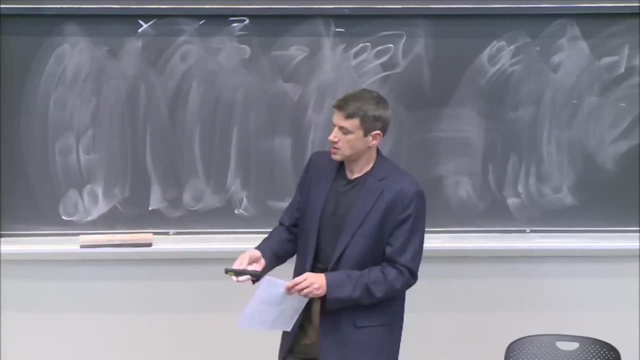 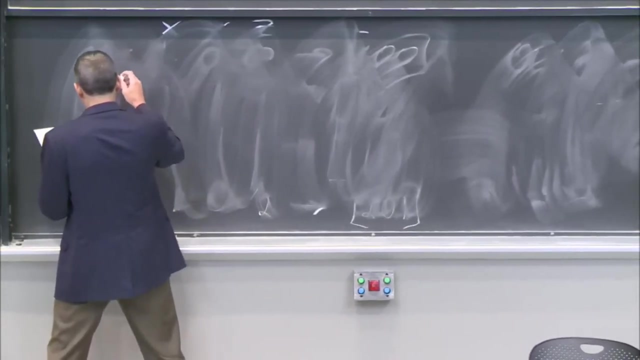 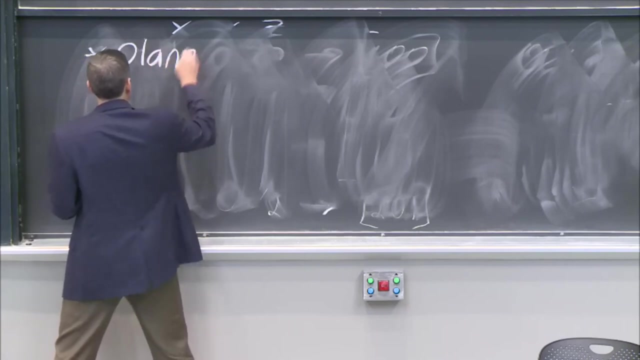 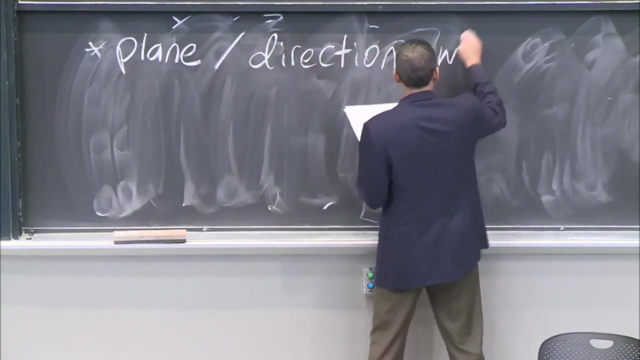 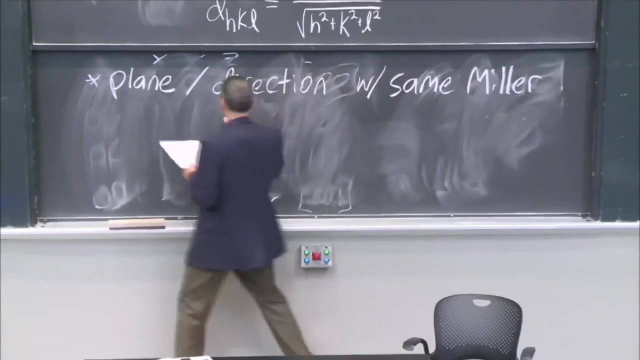 OK, So that's the distance between them, And the other thing that actually becomes fairly self-evident when you play around with this a little bit- and that was on the slide before- is that The Let's see The plane and the direction with the same Miller indices. 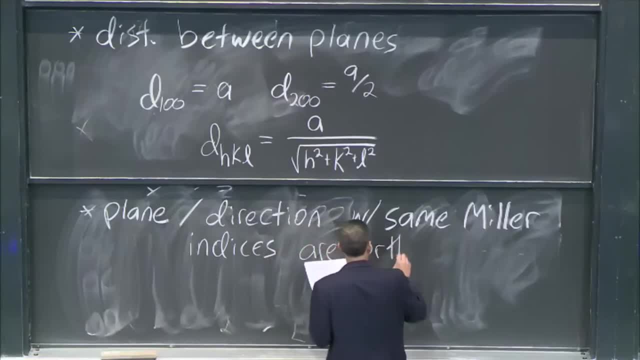 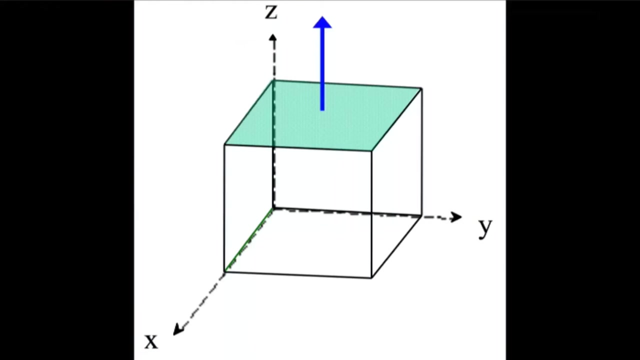 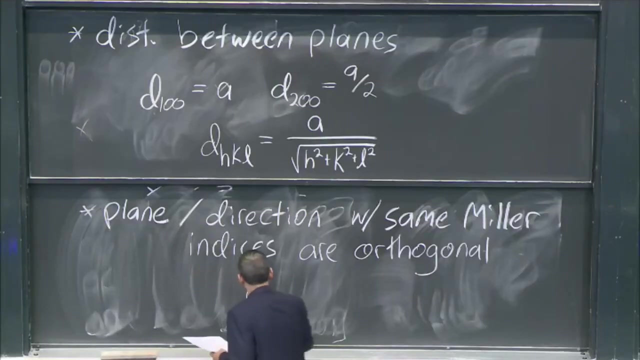 are orthogonal, And you can see this from this very simple picture. There's the 001 plane, But that's also the 001 vector, just as we defined it today. So the 001 plane and the 001 vector are orthogonal. So this is an example. 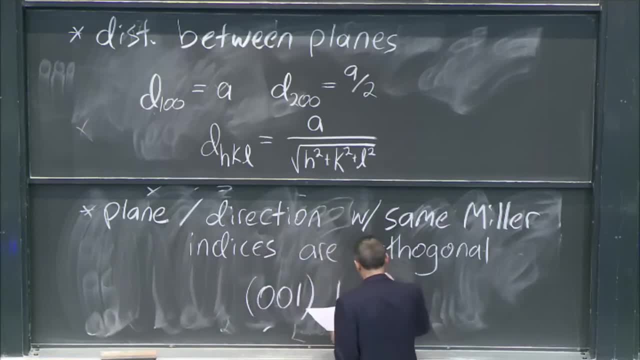 The 001 plane is orthogonal to Oh, and I've got to get this right. The 001 vector, Oh, Oh. No commas, brackets, parentheses, no negatives, no fractions, no infinities. I followed the rules. 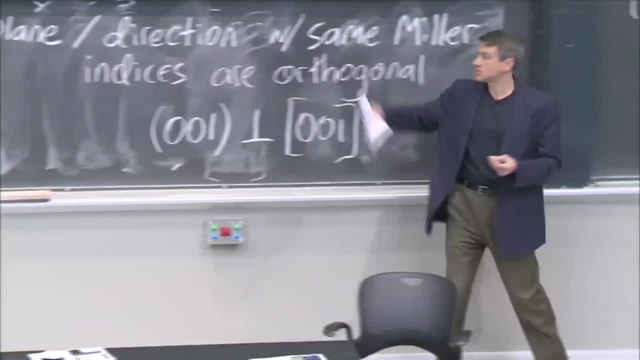 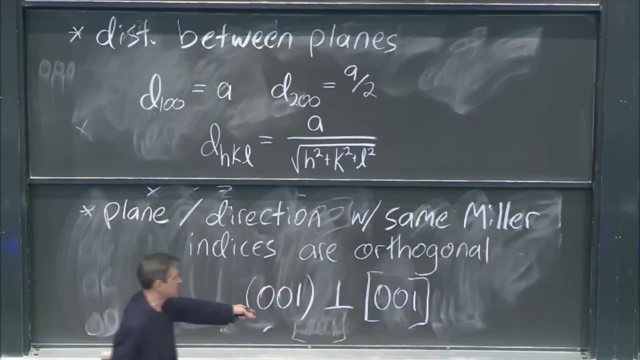 And because of that, these indices have meaning, as I'm showing you. Because of that, Now you can play around with this, But this can also be fairly straightforwardly derived, things like this: But you don't need to know that derivation. 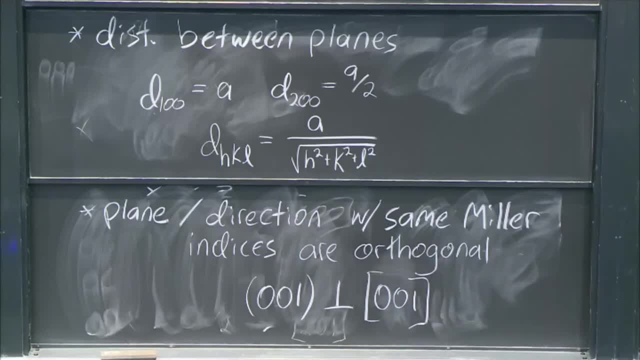 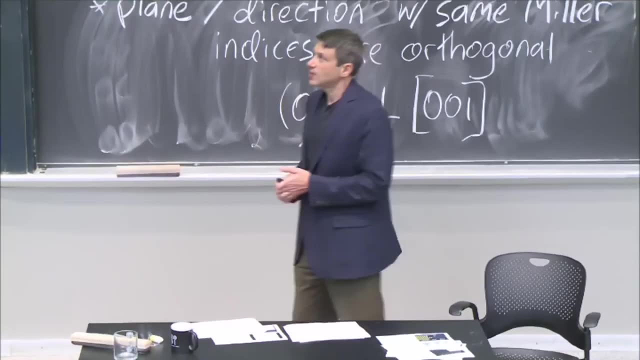 So I'm just telling it to you. OK, All right, So these are the kinds of things that you can do with Miller indices, As I said in the beginning, one of the things that you would want to know what planes you're talking about. 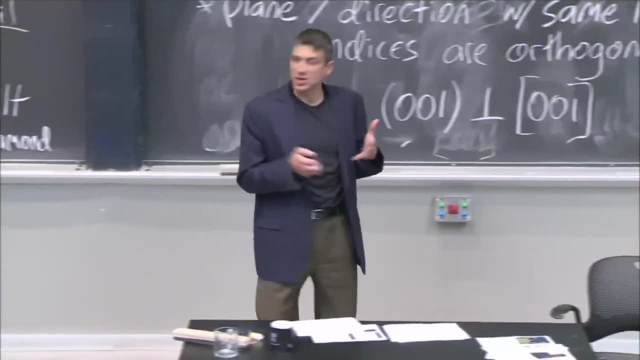 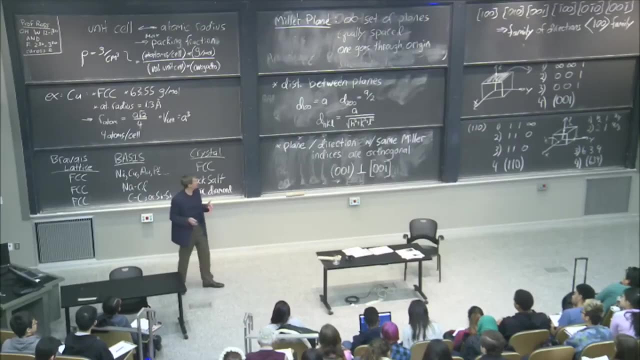 is because you want to know what the packing in that plane is, Just like we talked about packing for- well, we talked about it before, on Monday- the atomic packing fraction. There it is the max packing fraction in a volume. We also want to know: 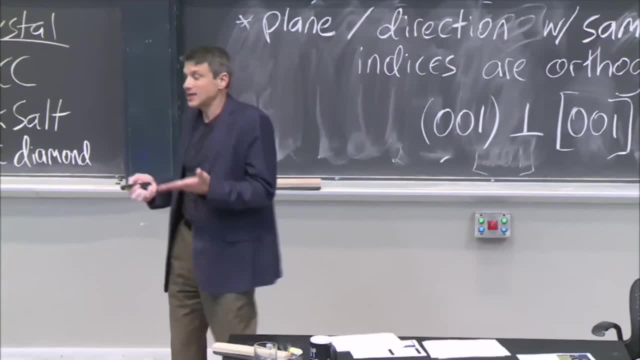 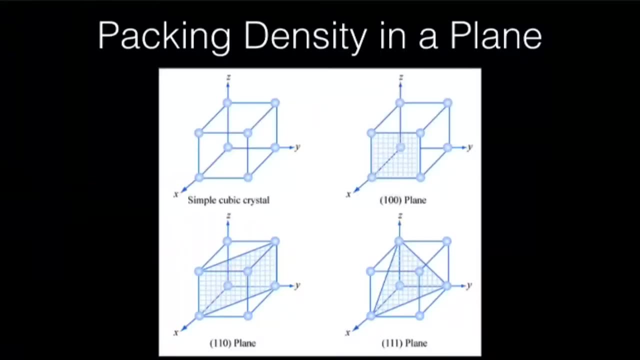 Especially if a crystal is anisotropic. we want to know about packings in planes, right? And so, if you take a simple, a very simple example, like a simple cubic, there's a simple cubic lattice And now we're all good with our notation, right? 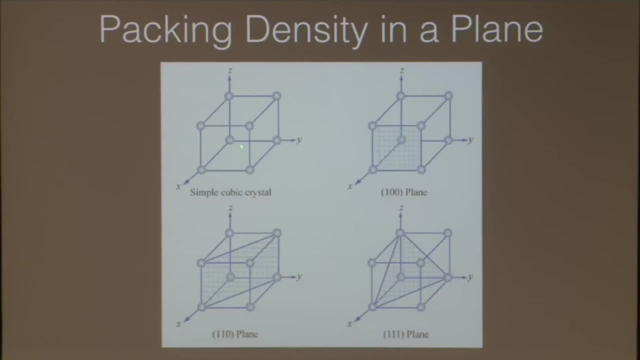 There's a simple cubic crystal. OK, The basis is one atom. I don't have anything else in here. Those are the atoms, Simple crystal. It must be polonium, right. And there's the 100 plane, The 110 plane and the 111 plane. 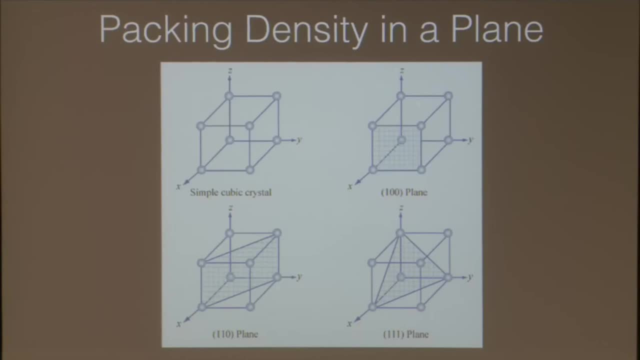 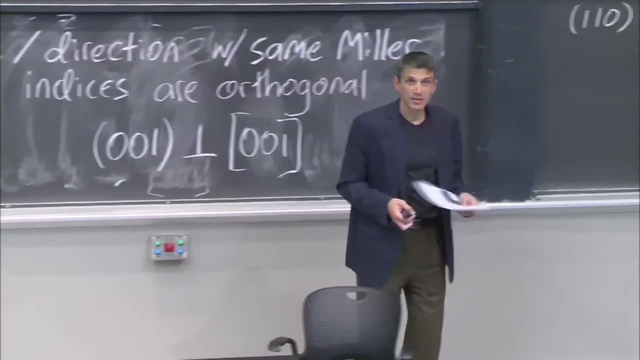 111 plane, 110 plane, right, 110 plane. But, as you can see, the density of atoms in these planes is different. The density of atoms in these planes is different And that has a real, serious impact on the properties. 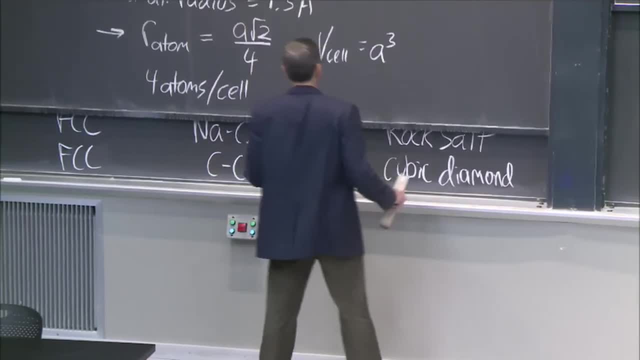 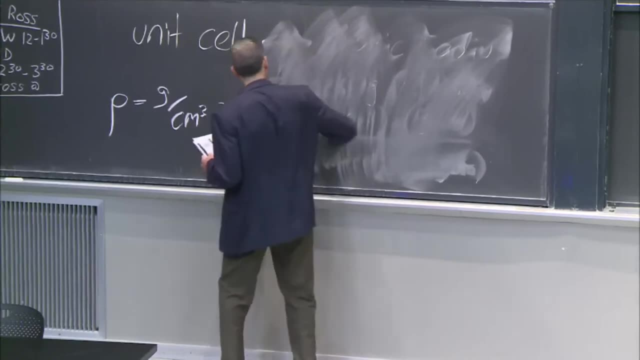 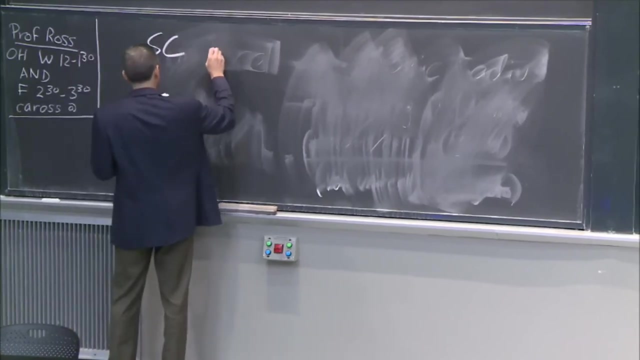 right. So if we look at this, so I'll do a couple quick examples. If we look at this example of simple cubic, that's a very easy case. And so for a simple cubic, for a simple cubic with a lattice, this A is called the lattice constant. 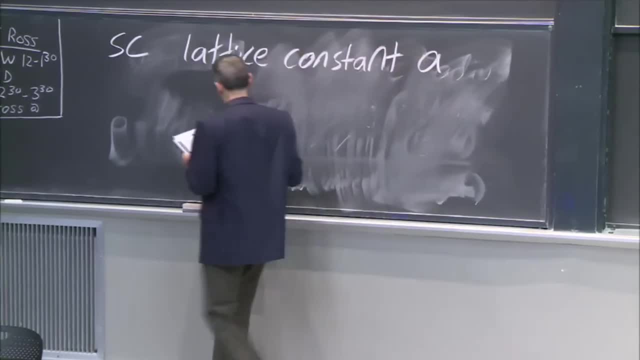 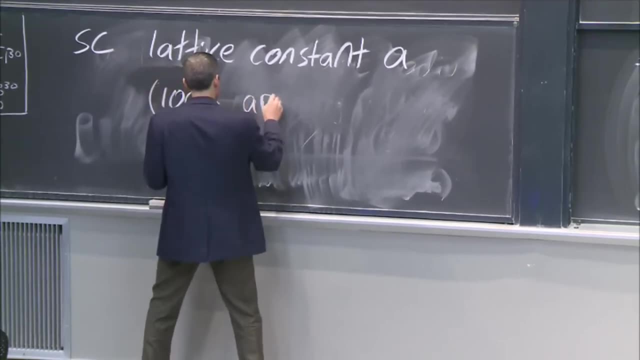 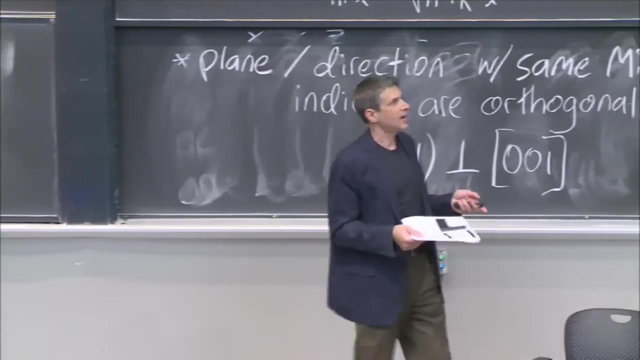 I've mentioned it a few times: Lattice, constant A. Then if we look at the 100 plane, then the area is A squared. The area of that plane is A squared. No, The question is how many atoms are in that A squared? 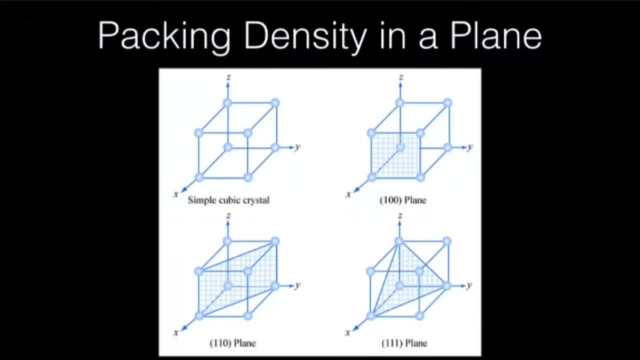 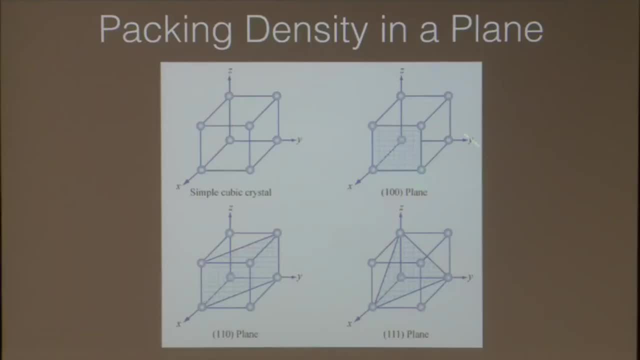 Well, you do the same thing that we did before. So I'm looking at a plane here And I'm trying to figure out how many atoms are in this. Well, you know, this is being shared in this whole big plane. that goes on and on. 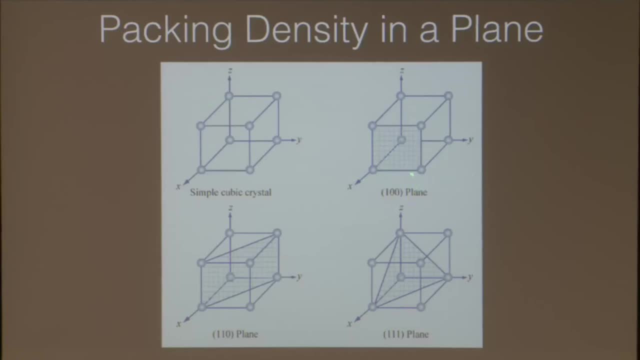 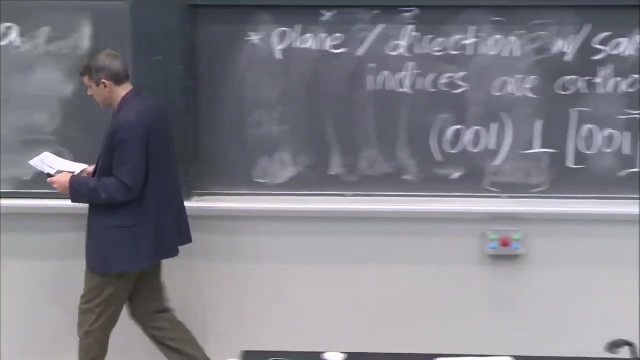 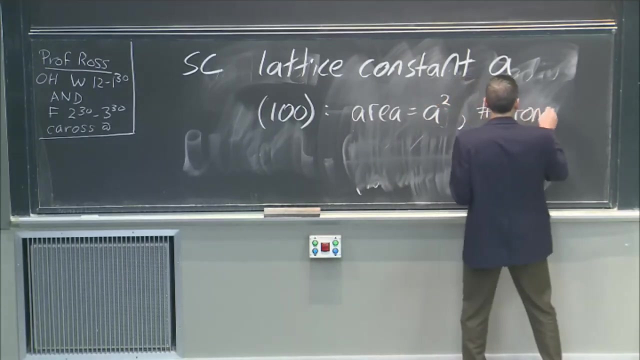 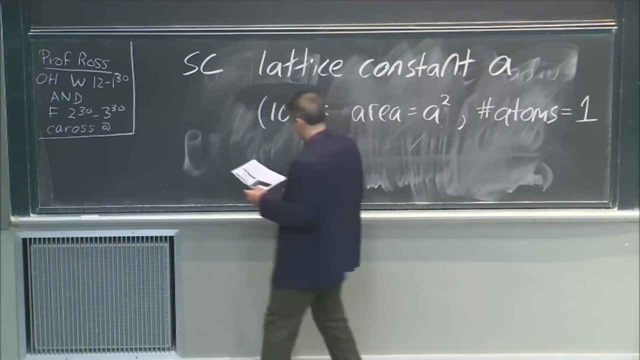 It's being shared by four other squares, right, And so there's a fourth of each atom in there, So there's one atom effectively in that plane. Again, this is one of the simplest cases, right? But the number of atoms is equal to 1,, right? 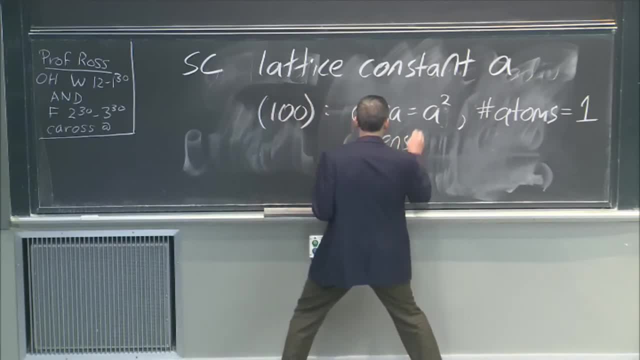 And so the density of atoms per area is equal to 1 over A squared. That's a pretty easy case, right? If I did the 1,, 1, 1, 1, 1, 0 direction, it's a little bit different, because the area is now. 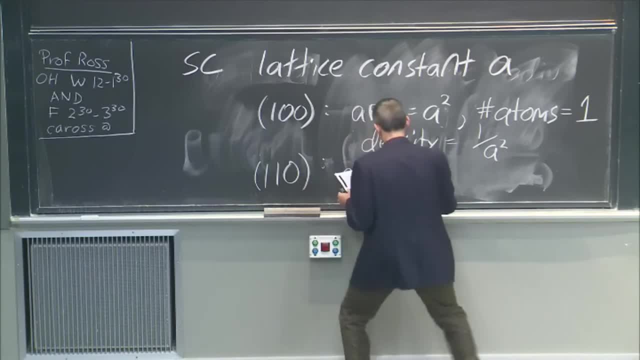 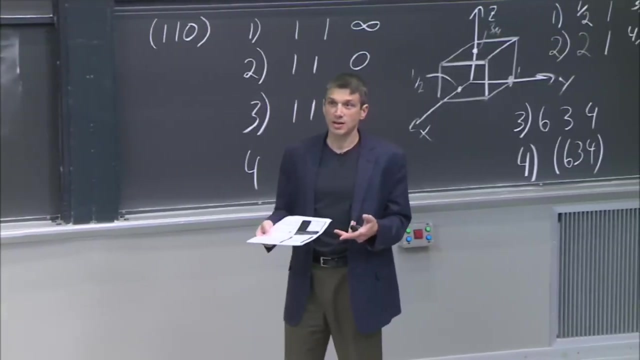 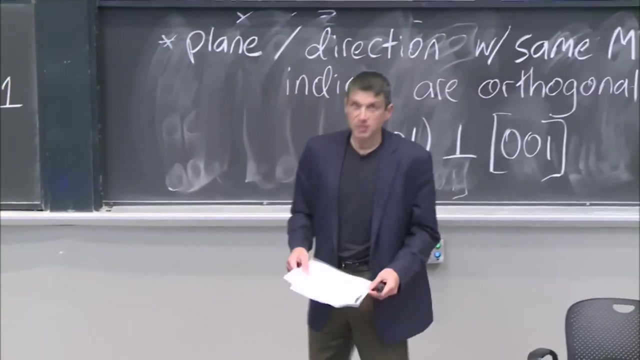 different right. So the area in this case is root 2 A squared. You see that The area in that plane is different, So the density of atoms in the plane is different. OK, So the density in the plane affects properties. 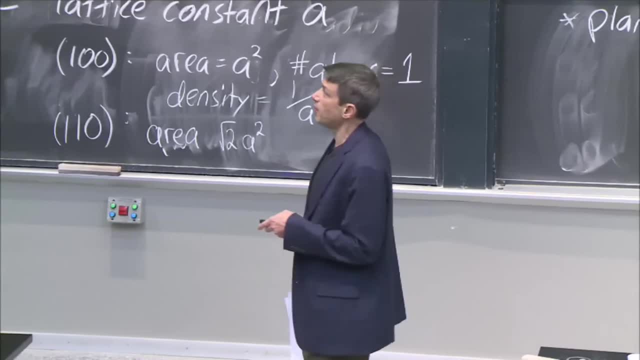 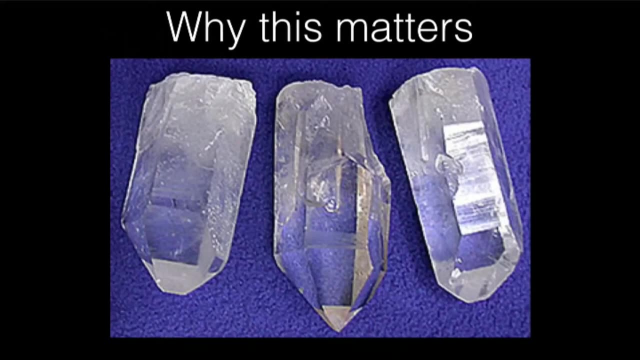 And I want to give you just a quick example of that in the why this matters, Because in fact, this is one of the things. all the way back to Hooke and his cannonballs and even way before that, people noticed this stuff. 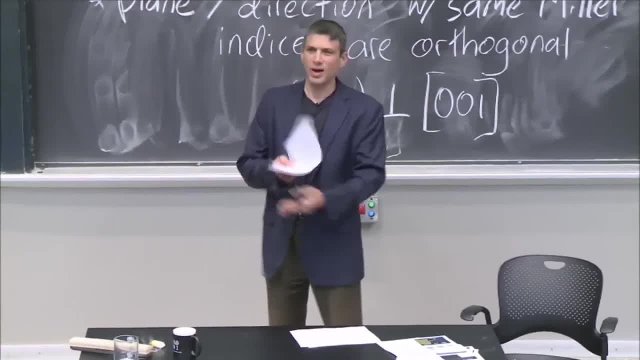 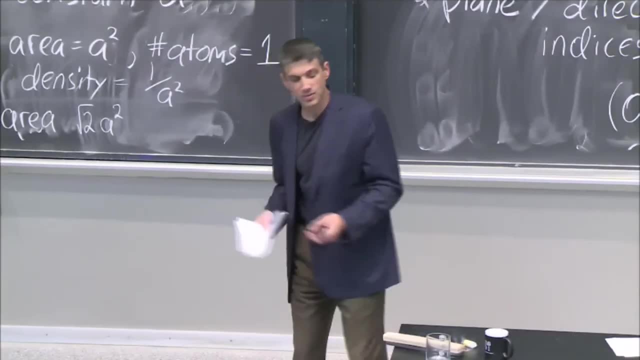 I broke something, but it always seems to slice in a certain way. Why is that? Why would something always break in the same way, every time, with the same kind of you know? how do they? what does way mean here? It means like the angles that form right. 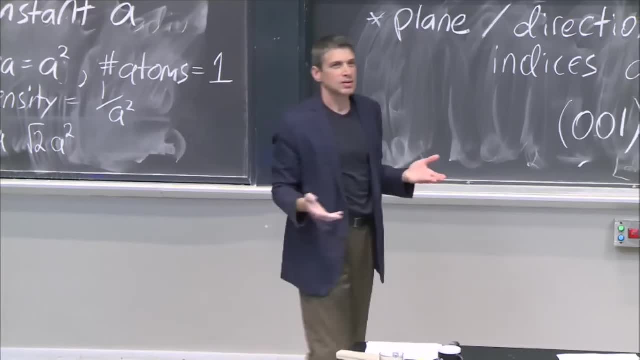 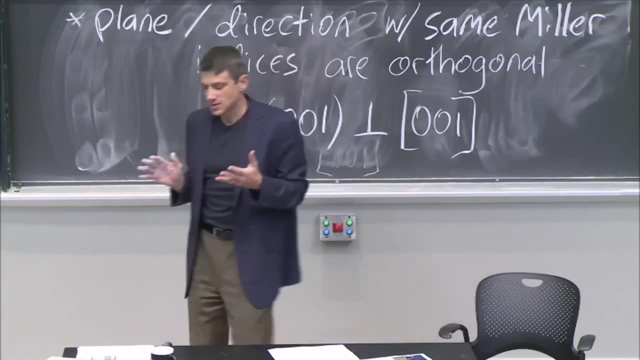 So why are those angles always kind of the same right? Well, it has to do. It has to do with the strength, the relative strength of the planes inside of these crystals, right? And in fact, here's a beautiful piece of work. 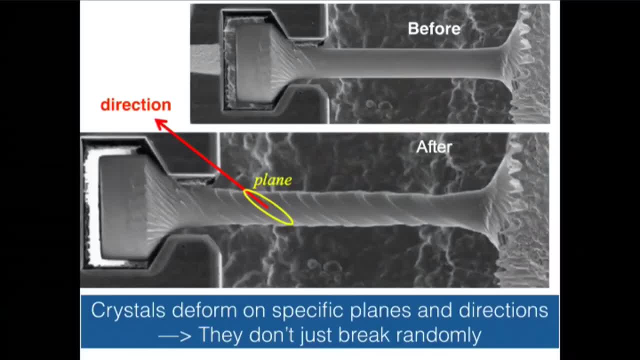 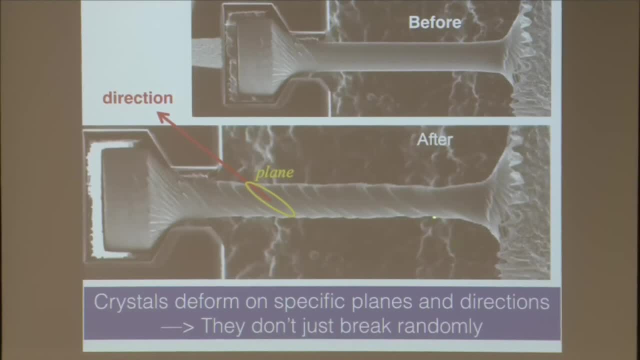 on stretching a wire right. So here you're taking a wire that is crystalline and you're pulling it And you can see how it breaks. You can actually see how it breaks. It's breaking along the weakest plane. It's breaking along the weakest plane. 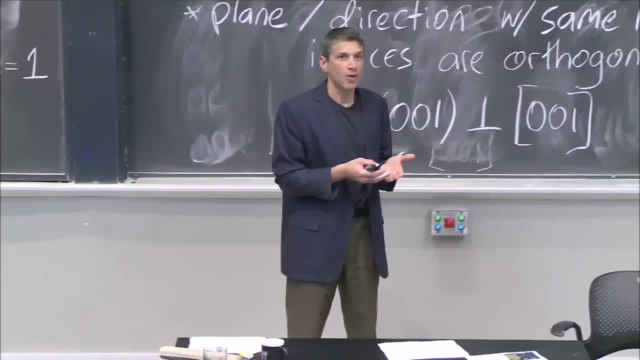 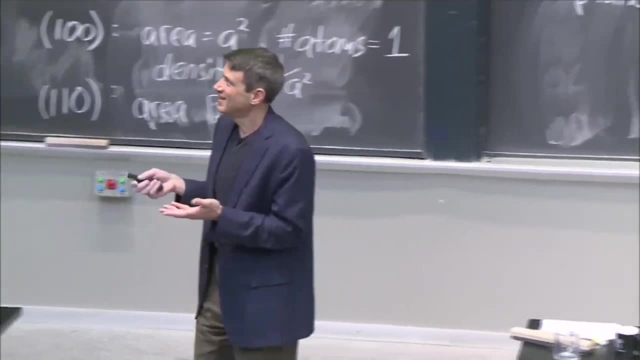 So if you want to think, then about: well, OK, how do I know how to make this stronger, For example, so it stops breaking? You know, the weakest link is the weakest link. right, That was deep, But so then that's the plane of the crystal. 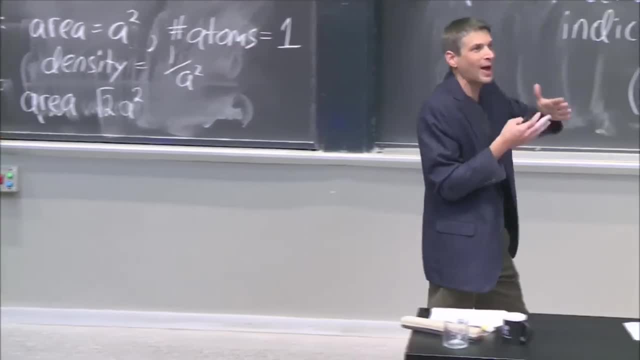 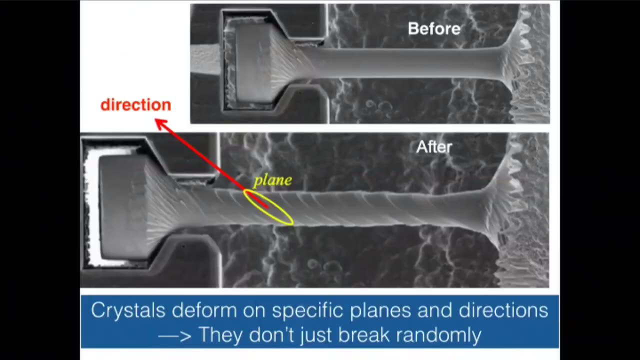 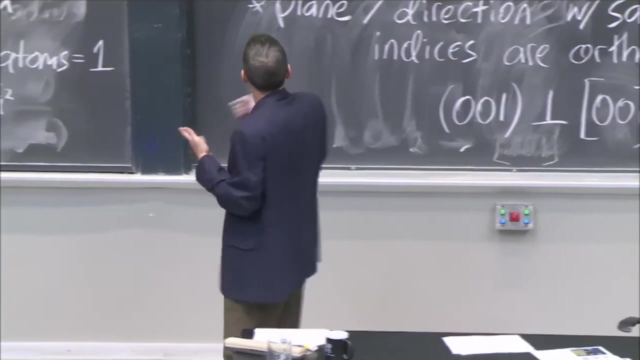 that I need to think about. How are atoms bonding together or packing in in that plane? right, This is real stuff. This comes about in many of the properties, not just the fracture, but in many of the properties of these materials, the property, as I said before. 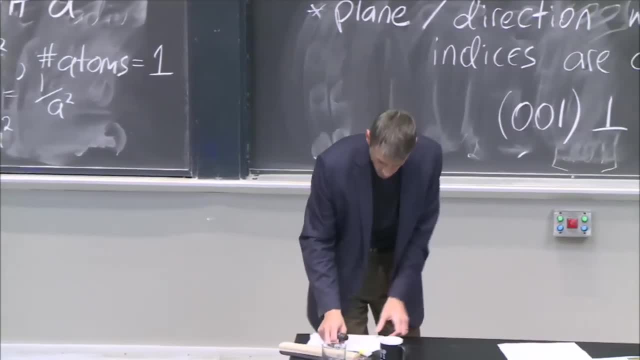 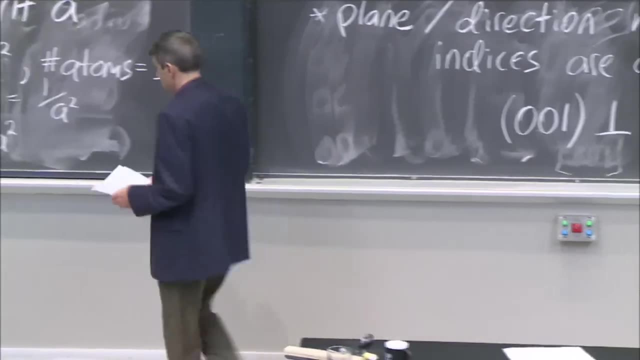 depends heavily on which plane you're in, And we'll see that more and more. As one last example, as one last example of this, you could go a little right. So if I say again, you go back to your periodic table.